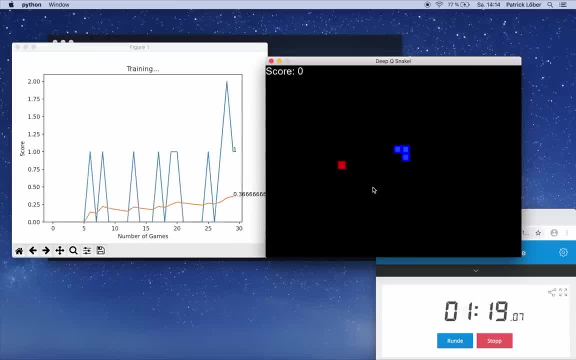 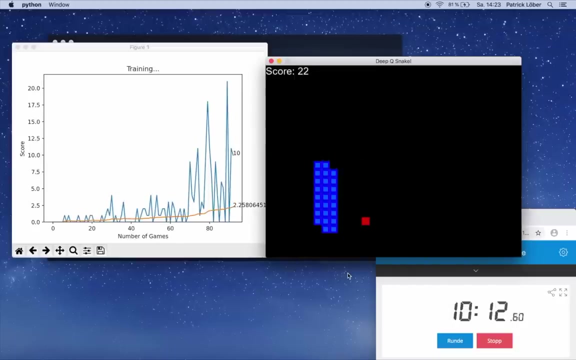 Okay, so let me speed this up a little bit, Alright, so now about 10 minutes have passed and we are at about game 90, I guess, And now we can clearly see that our snake knows what it should do, So it's more or less going straight for. 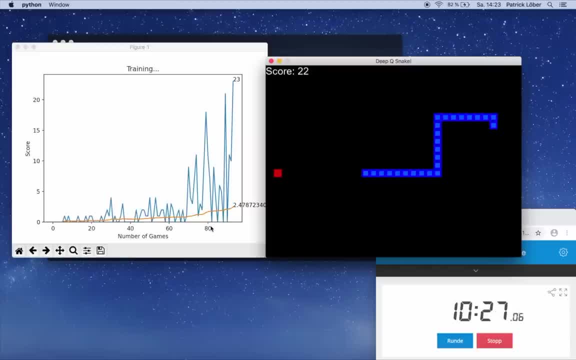 the food and tries not to hit the boundaries. So it's not perfect at this point, but we can see that it's getting better and better. So we also see that the average score here is increasing And now the best score so far is 25.. And, to be honest, for me this is super exciting. So if 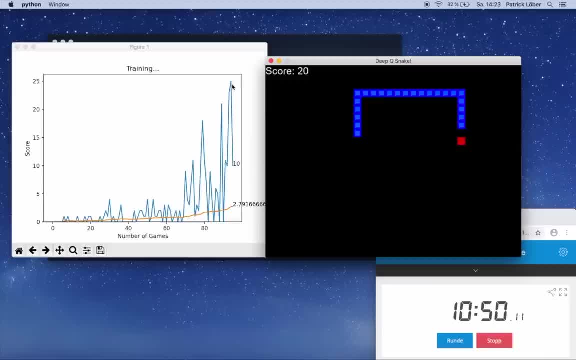 we imagine that we are going to have a game of chess. we are going to have a game of chess and that at the beginning, our snake didn't know anything about the game, And now, with a little bit of math behind the scenes, it's clearly following a strategy. So this is just super cool, don't you? 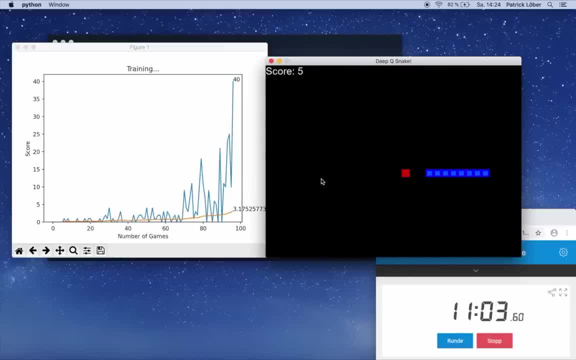 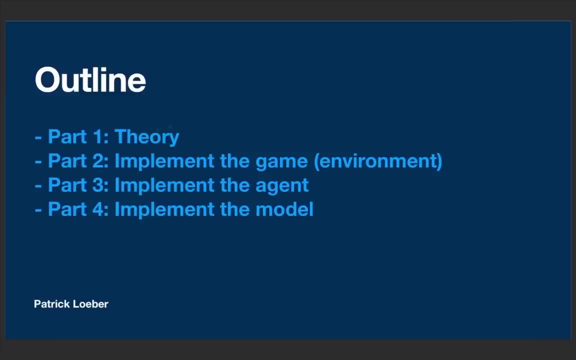 think. All right. so let me speed this up a little bit more, All right. so after 12 minutes, our snake is getting better and better, So I think you can clearly see that our algorithm works. So now let me stop this, And then let's start with the theory. So I will split the series into four. 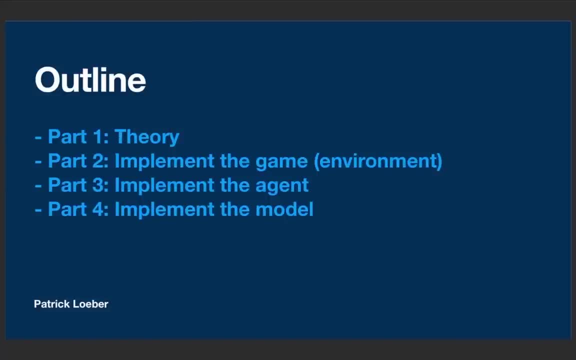 parts. In this first video we learn a little bit about the theory of reinforcement learning. In the second part we implement the actual game, or also called the environment, here with pi game. Then we implement the actual game, And then we implement the actual game, And then we implement the actual. 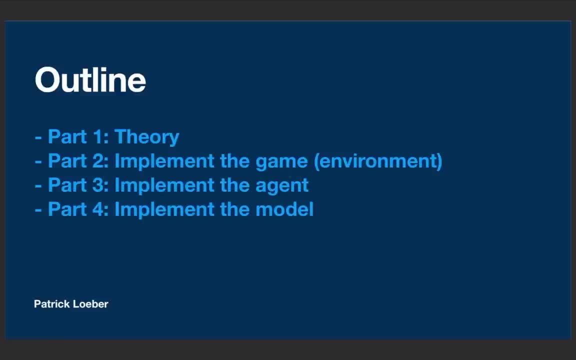 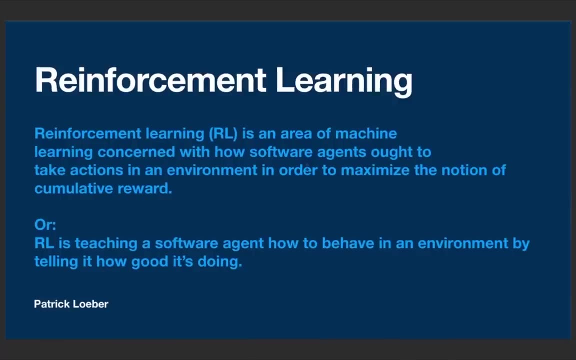 agent. So I will tell you what this means in a second And in the last part we implement the actual model with PyTorch. So let's start with a little bit of theory about reinforcement learning. So this is the definition from Wikipedia. So reinforcement learning is an area of machine. 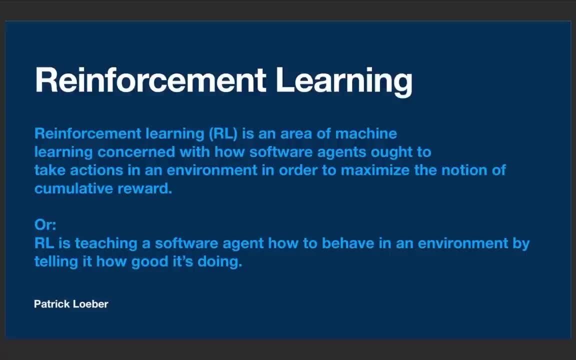 learning concerned with how software agents ought to take actions in an environment in order to maximize the notion of cumulative reward. this might sound a little bit complicated, So in other words, we can also say that reinforcement learning is teaching a software agent how to behave in an environment by telling it how good 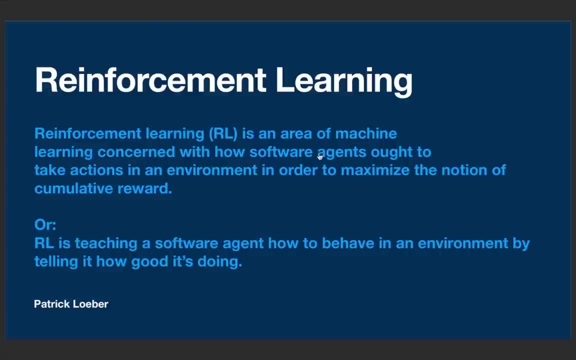 it's doing. So what we should remember here is that we have an agent, So that's basically our computer player- then we have an environment- So this is our game in this case- And then we give the agent a reward. So with this, we tell it how good it's doing And then, based on their reward, 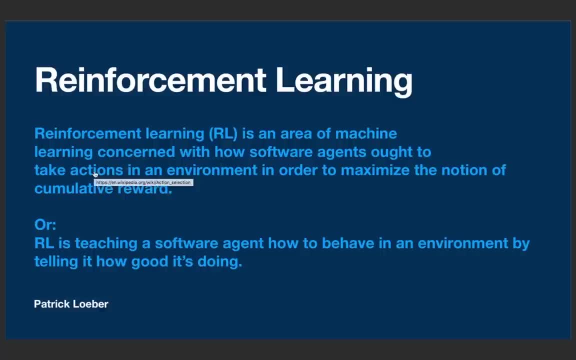 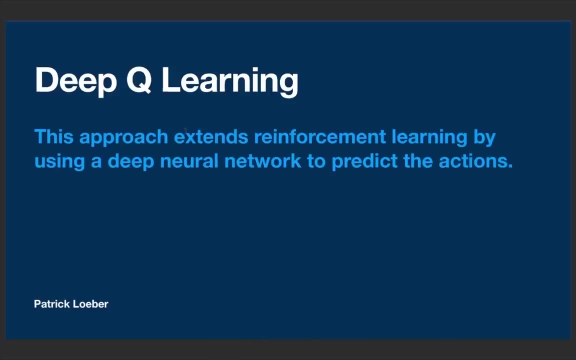 it should try to find the best next action. So yeah, that's reinforcement learning And to train the agent. there are a lot of different approaches and not all of them involve deep learning, But in our case, we use deep learning, And this is also called deep Q learning. So 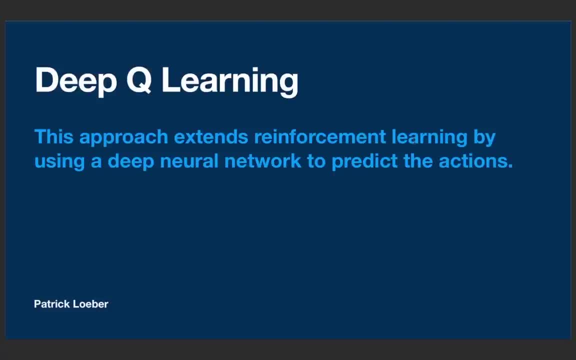 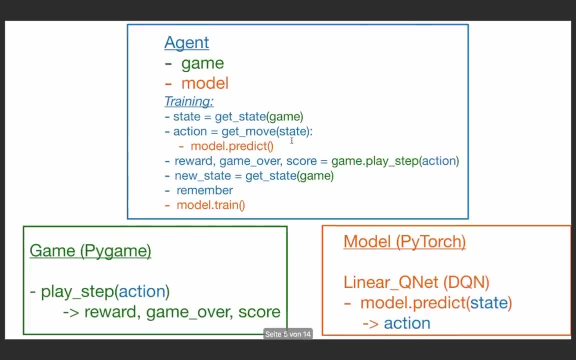 this approach extends reinforcement learning by using a deep neural network to predict the actions, And that's we're going to use in this tutorial. Alright, so let me show you the rough overview of how I organize the code. So, as I said, we're having four parts, So in the next part we implement the. 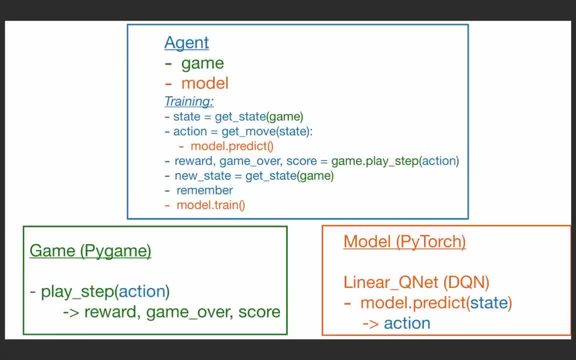 game with pi game, then we implement the agent and then we implement the model with pi torch. So our game has to be this sign, such that we have a game loop And then with each game loop we do a play step that gets an action, And then it does a step So it moves the snake, and then, after the move, 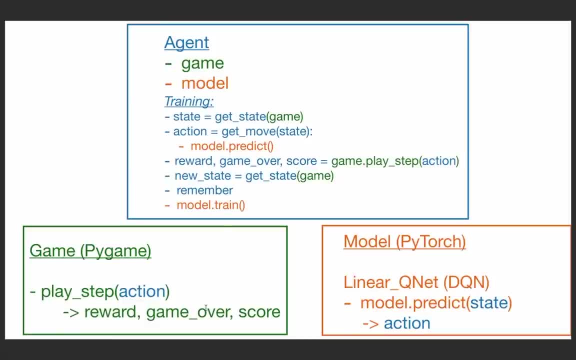 it returns the current reward and if we are game over or not, and then also the current score, then we have the agent, And the agent basically puts everything together. So that's why it must know about the game And it also knows about the model. So we store both, both of them- in our agent And then we implement the 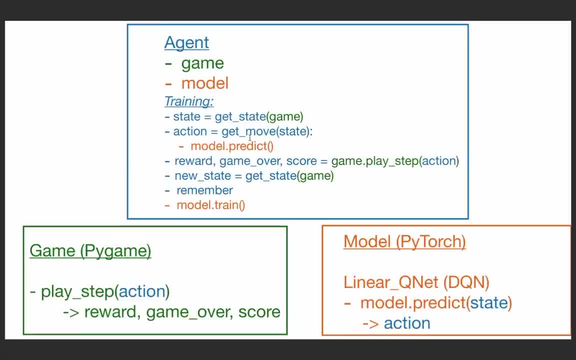 training loop. So this is roughly what we have to do. So, based on the game, we have to calculate a state, And then, based on the state, we calculate the next action, And this involves calling model predict, And then, with this new action, we do a next play step And 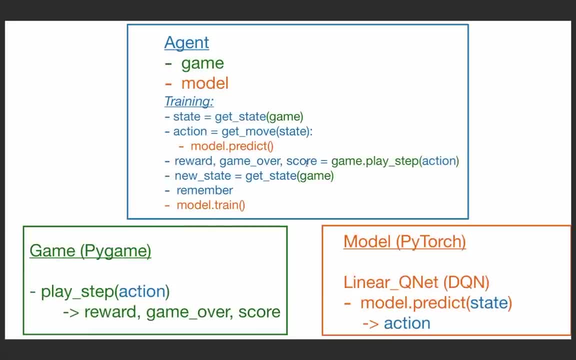 then, as I said, we get the reward, the game over state and the score, And now, with this information, we calculate a new state And then we remember all of this. So we store the new state and the old state and the game over state and the score. 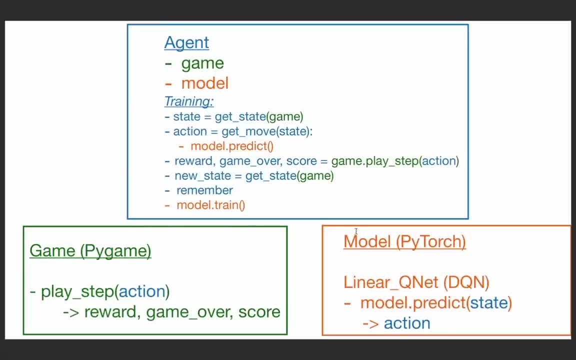 And we, And with this we then train our model. So for the model, I call this linear q net. So this is not too complicated. This is just a feed forward neural net with a few linear layers and it needs to have the these information, So the new state and the old state, and then 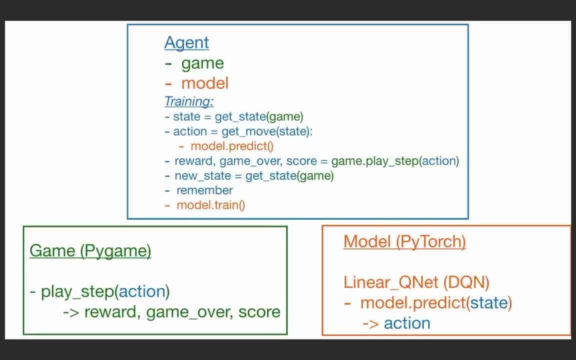 we can train the model and we can call model predict, And then this gets us the next action. So yeah, this is a rough overview how the code should look like, And now let's talk about some of those variables in more detail, for example, the action or the state or the reward. So 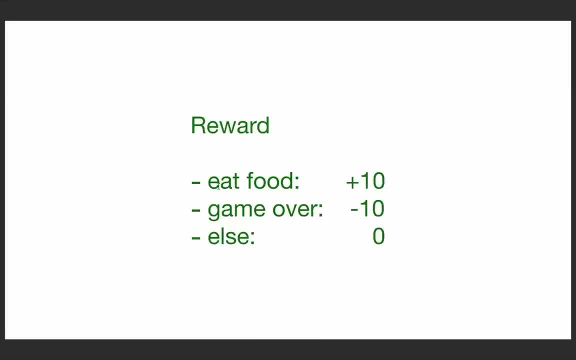 let's start with the reward. So that's pretty easy. So whenever our snake eats a food, we give it a plus 10 reward when we are game over. so when we die, then we get minus 10.. And for everything else we just stay. 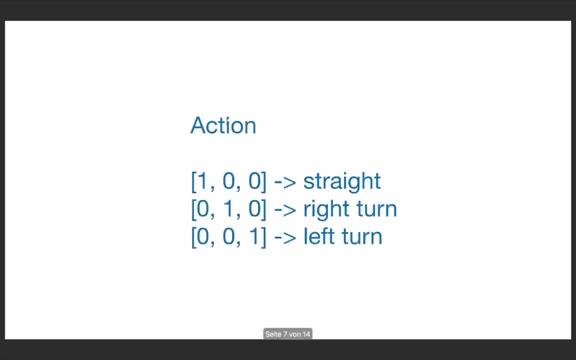 Okay, Okay at zero. So that's pretty simple. Then we have the action, So the action determines our next move. So we could think that we have four different actions, So left, right, up and down. But if we design it like this, then, for example, what can happen is if we go right, 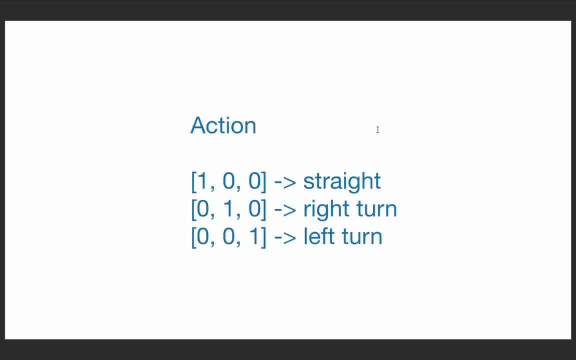 then we might take the action left and then we immediately die. So this is basically a 180 degree turn. So we don't allow that. So a better approach to design the action is to only use three different numbers. And now this is dependent on the current direction. 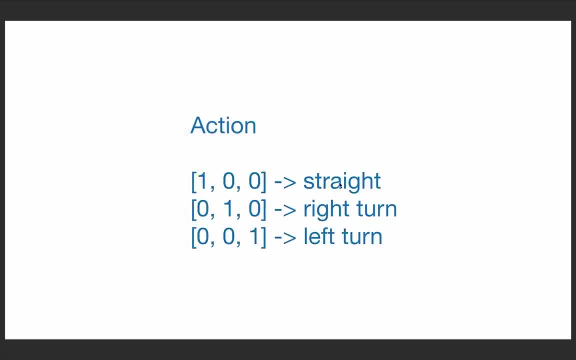 So one zero zero means we stay in the current direction, So we go straight. So this means if we go right, then we stay right, If we go left, then we go left, and so on. Then if we have 010, this means we do a right turn. And again, this depends. 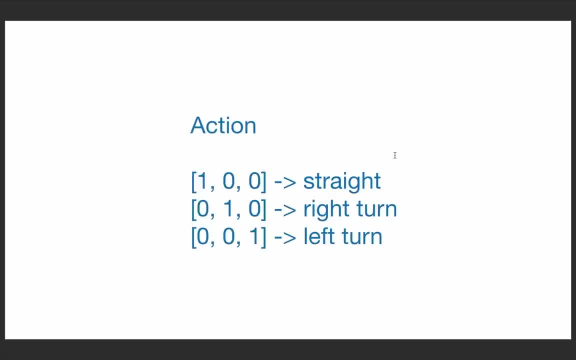 on the current direction. So if we go right and do a right turn, then we go down. next, If we go down and do a right turn again, then we go left, and then again we would go up. So this is the writer. 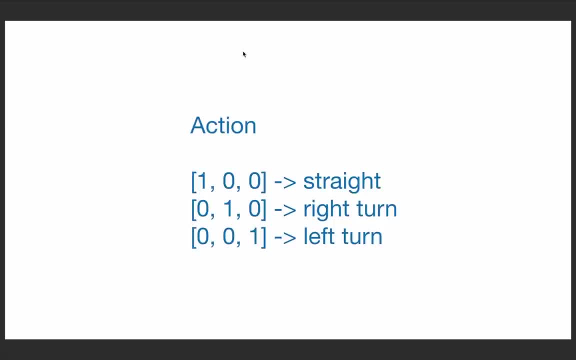 You could always do only two options which can take this in the right direction. So we go left and then click on do left from here and then do a rest, three different an turn. We go left and do a left turn, then we go down And then we go 80 degree turn and also. 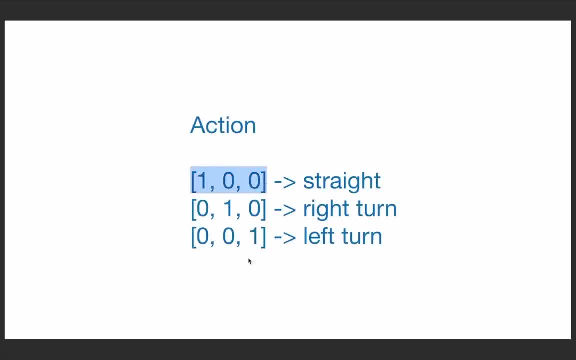 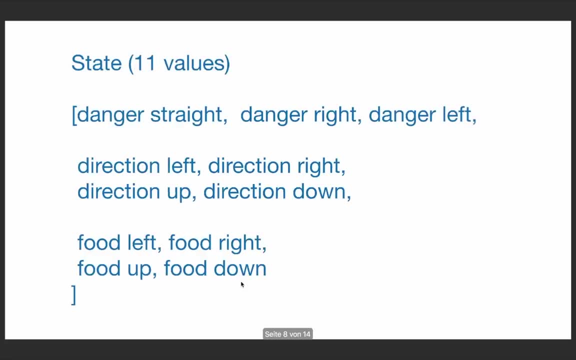 we only have to predict three different states, So this will make it a little bit easier for our model. So now we have the reward and the action, then we also need to calculate the state, And the state means that we have to tell your model that there is a right Scotland. 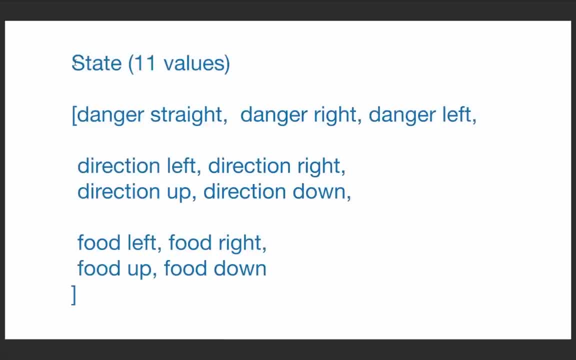 snake some information about the game that it knows about, So it needs to know about the environment, And in this case, our state has 11 values, So it has the information if the danger is straight or if it's a hat, if the danger is right or if the danger is left. 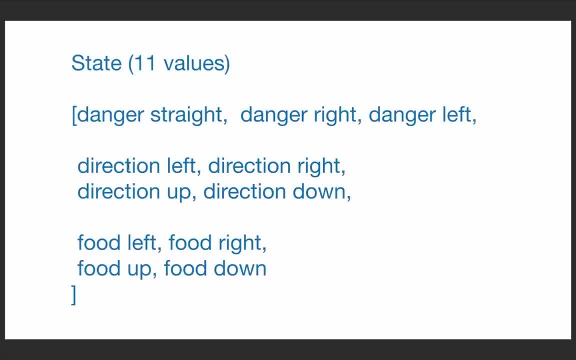 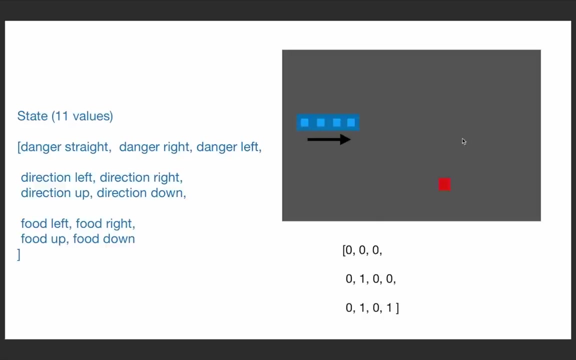 then it has the current direction, So direction left, right, up and down, And then it has the information if the food is left or right, or up or down, And all of these are boolean values. So let me show you an actual example. So in this case, if we are going right and our 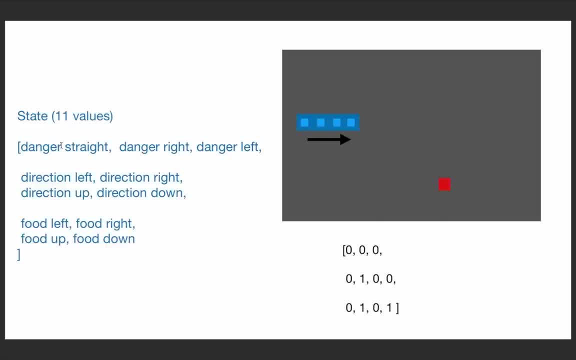 food is here, then we see danger straight, right, left, up and down, And then it has right and left. none of this is true. So, for example, if our snake is over here at this end and it's still going right, then danger straight would be a one. So this again also. 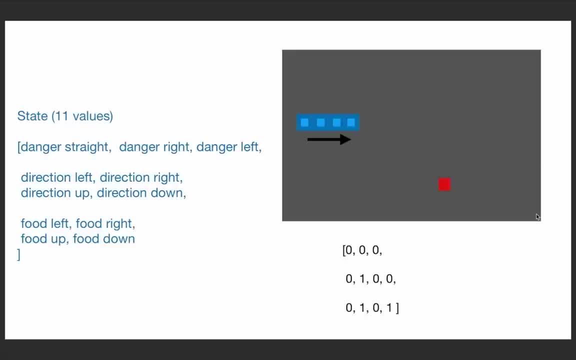 depends on the current direction. For example, if we move up at this corner here, then danger right would be a one. Then for these directions only one of them is one and the rest is always zero. So in this case we have danger right set to one. And then for this, in our case, our food is. 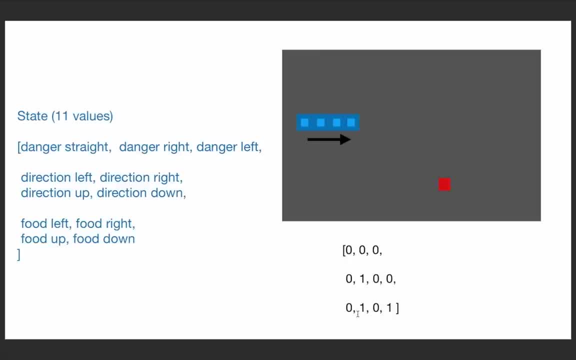 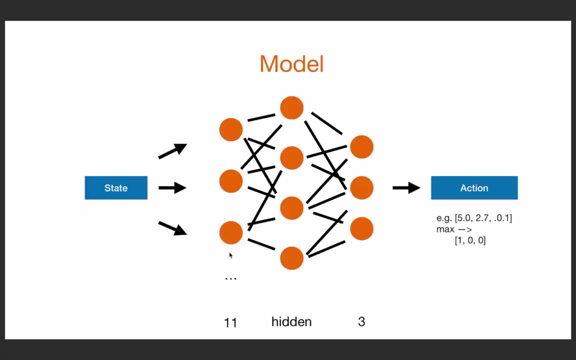 right of the snake and also down of the snake. So food right is one and food down is one. Alright, so now with the state and the action, we can design our model. So this is just a feed forward neural net with an input layer, a hidden layer and an output layer. And for the input, 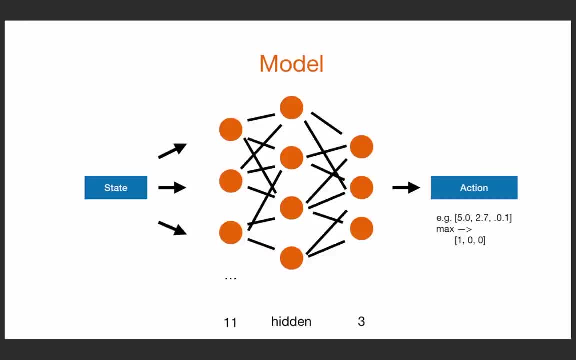 it gets the state. So, as I said, we have 11 different numbers in our state, 11 different Boolean values, zero or one, So we need this size, 11.. At the beginning then we can choose a hidden size And for the output we need three outputs. 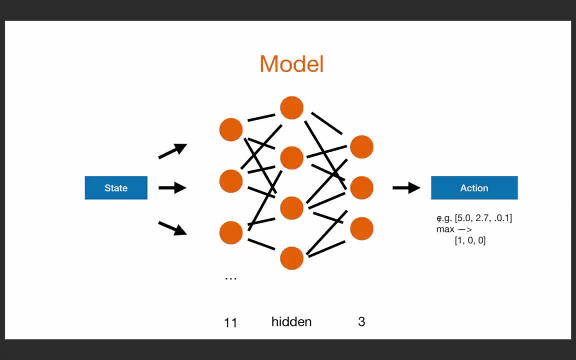 Because then we predict the action. So these can be some numbers And these don't need to be probabilities. So here we can have raw numbers And then we simply choose the maximum. So, for example, if we take 100, and if we go back, then we see this would be the action. 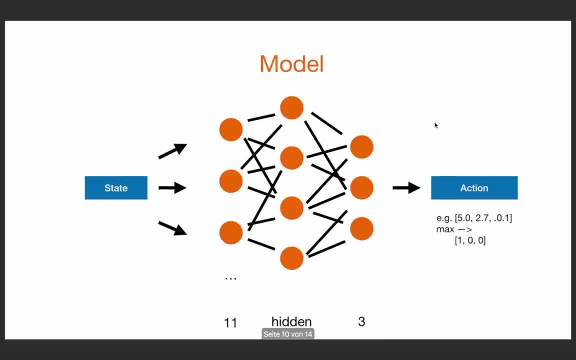 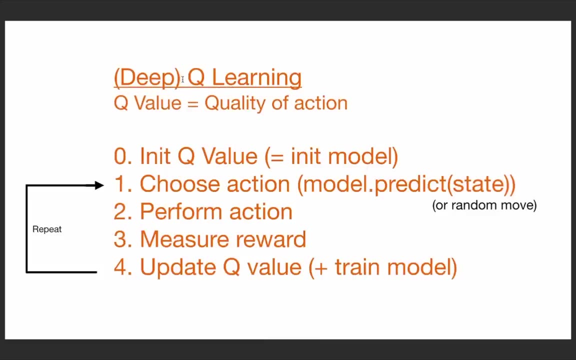 straight, So keep the current direction. So yeah, that's how our model looks like And, of course, now we have to train the model. So for this, let's talk a little bit about this deep Q learning. So Q stands for the, this is the Q value And this stands for the. 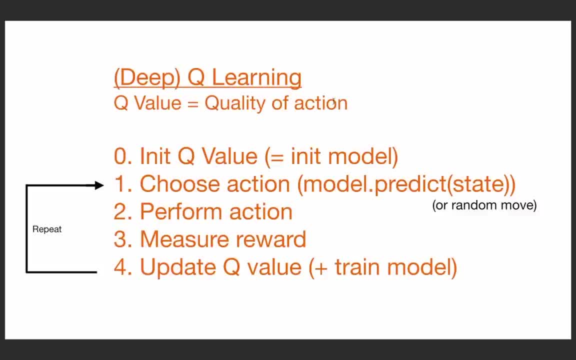 quality of the action. So this is what we want to improve. So each actions should improve the quality of the snake. So we start by initializing the Q value. So in this example we have a snake. In this case we initialize our model with some random parameters, then we choose an. 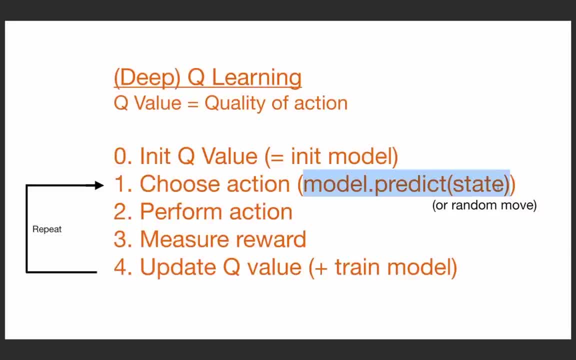 action by calling model, predict state, And we also sometimes choose a random move. So we do this especially at the beginning, when we don't know a lot about the game yet. So and then later we have to do a trade off when we don't want to do a random move anymore. 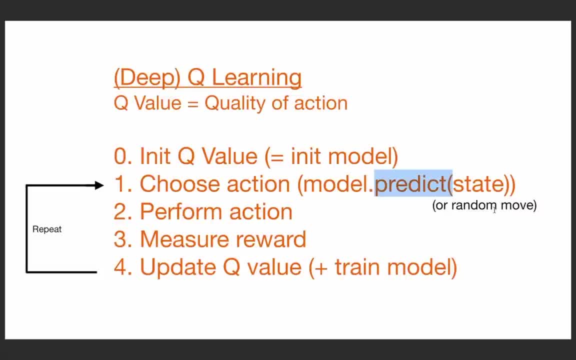 and only call model predict, And this is also called a trade off between exploration and exploitation. So this will get clearer later when we do the actual coding. So then, with this new action, we perform this action, So we perform the next move, and then we measure the reward. And with this information, 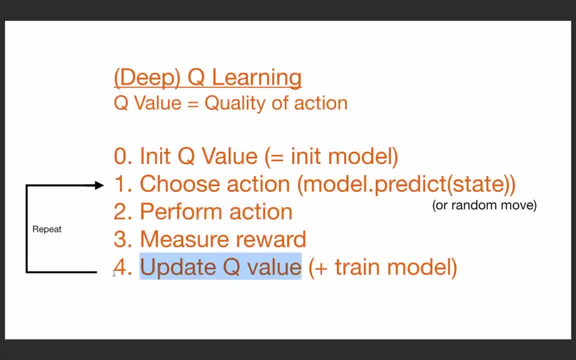 we can update our Q value and then train the model, And then we repeat this step. So this is an iterate training loop. So now, to train the model, as always, we need to have some kind of loss function that we want to optimize or minimize. So for the loss function, we have to look at a little bit of. 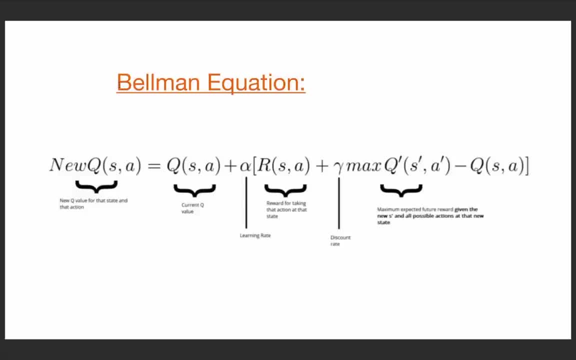 math, And for this I want to present you the so called Bellman equation. So this might look scary, So don't be scared. Here I will explain everything, And actually it's not that difficult when we understand this and then code this later. So what we want to do here? we need to update the 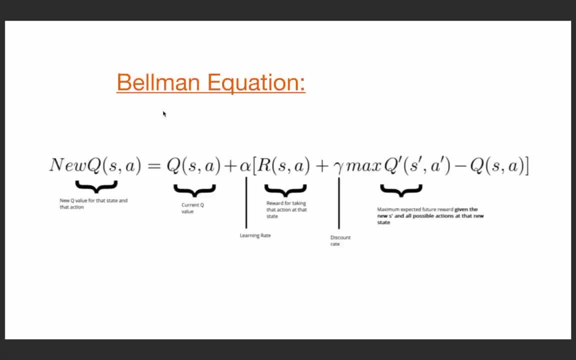 Q value, as I said here. so according to the Bellman equation, the new Q value is calculated like this. So we have the current Q value plus the learning rate, and then we have the reward for the loss function. What we want to do here is we want to calculate the value of our model. So 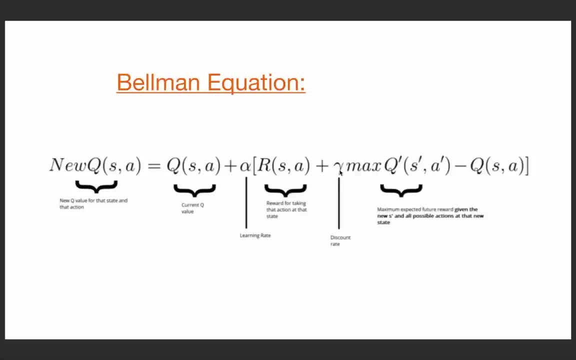 taking that action at that state, plus a gamma parameter which is called this count rate. So don't worry about this, I will also show this later in the code again. And then we take the maximum expected future reward given the new state and all possible actions at that new state. 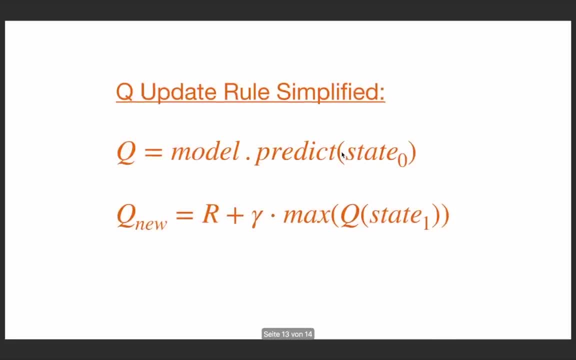 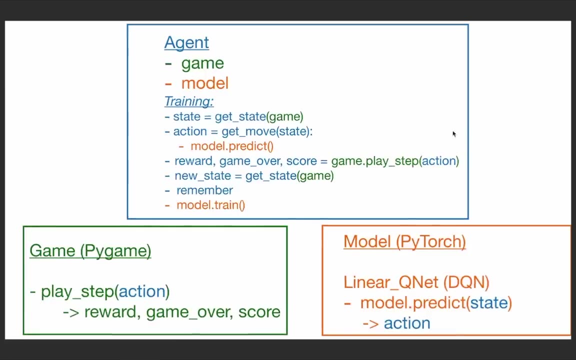 So yeah, this looks scary, but I will simplify that for you And then it's actually not that difficult. So the old Q value is model predict with state zero. So if we go back at this overview, so the first time we say, get state from the game, this is our state zero. And then, after we took 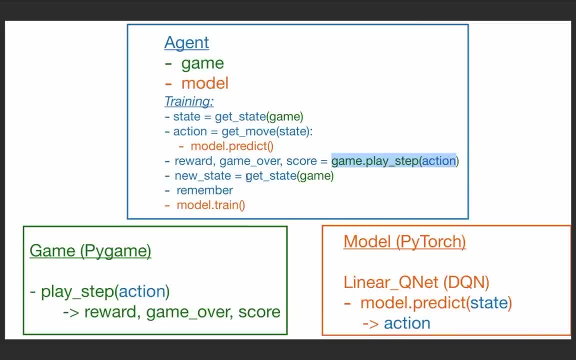 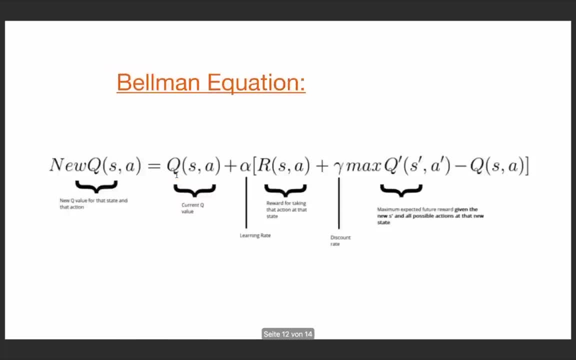 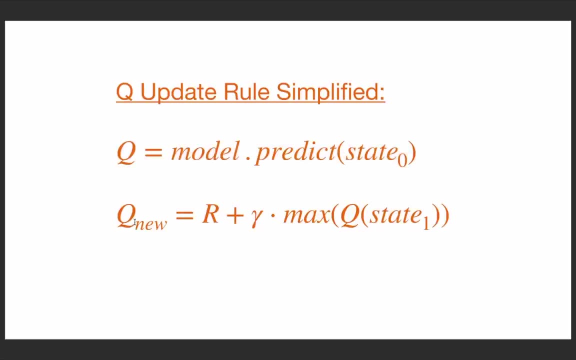 this play step, we again measure or calculate the next state. So this is then our state one. So with this information again, our first queue is such just model predict with the old state, And then the new queue is the reward plus our gamma value times the maximum value of the queue state. So again, this is model. 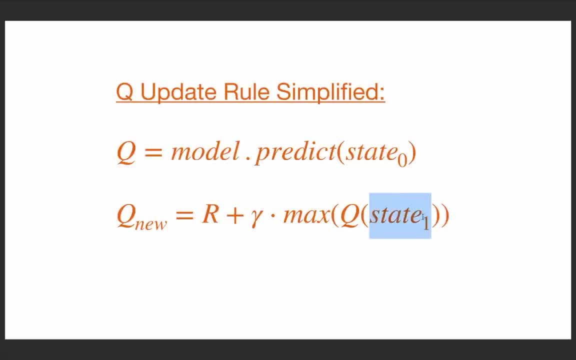 predict. But this time we take state one And then, with these two information, our loss is simply the queue new minus q, squared, And yeah, this is nothing else than the mean squared error. So that's a very simple error that we should already know about, And then this is what we must use in our optimization. So, yeah, 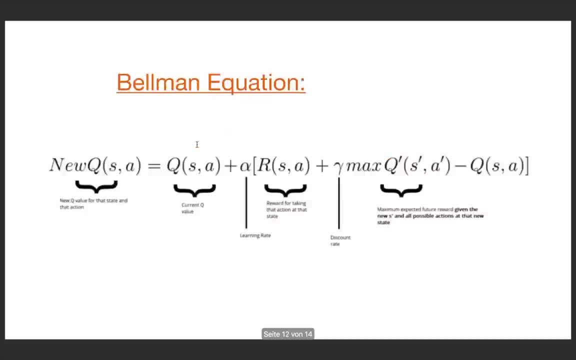 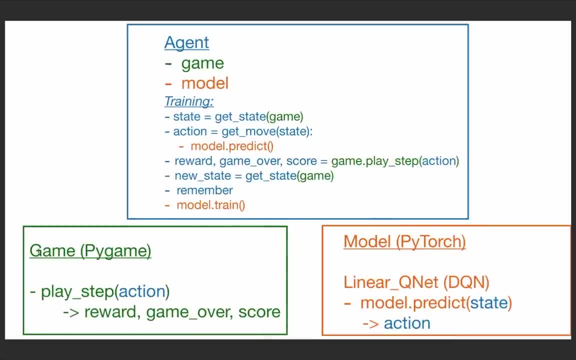 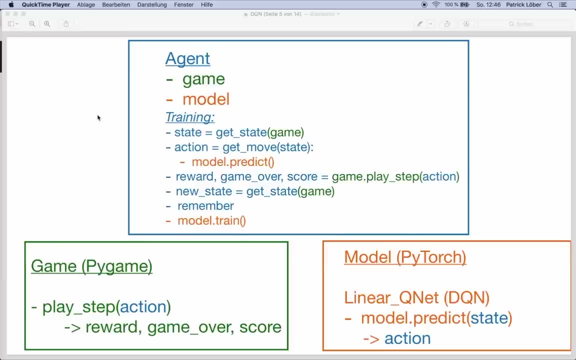 that's what we are going to use. So we have to implement all of these three classes And in the next video we start by implementing the game. In the last part, I showed you all the necessary theory that we need to know to get started with. 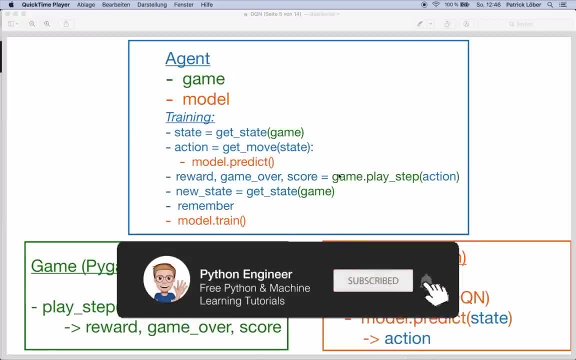 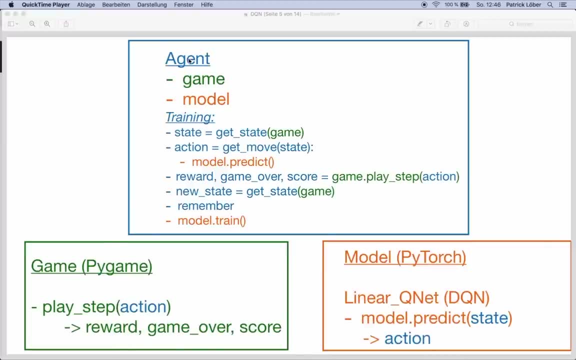 deep Q learning, And now we start implementing all of the parts. So, as I said, we need to have a game, so the environment, then we need an agent and we need a model. So in this part, we start by implementing the game and we use PyTorch for this. So let me actually start by creating a 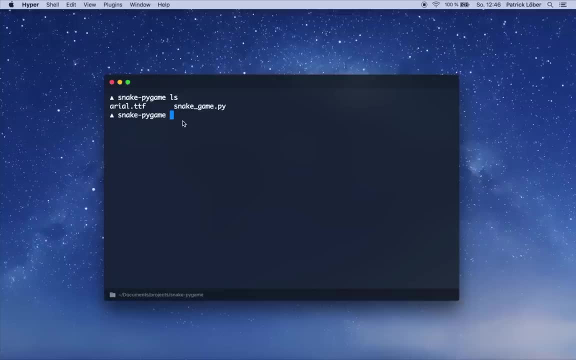 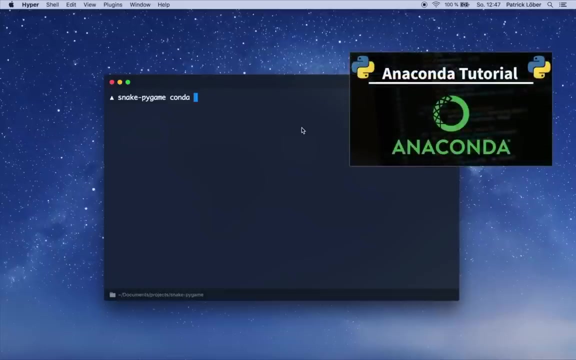 environment and we install all the necessary dependencies that we need. So in this case, I use conda to manage the environments, And if you don't know how to use conda, then I have a tutorial for you that I will link here. But yeah, if you don't want to use conda, you can also just use a normal. 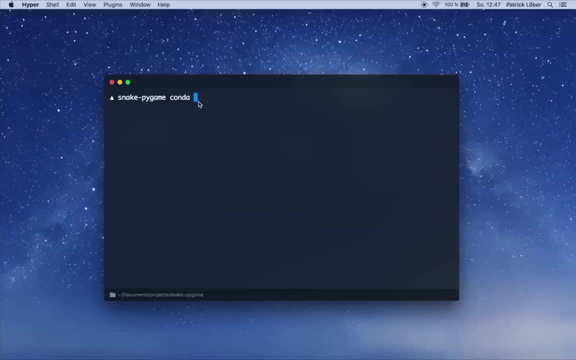 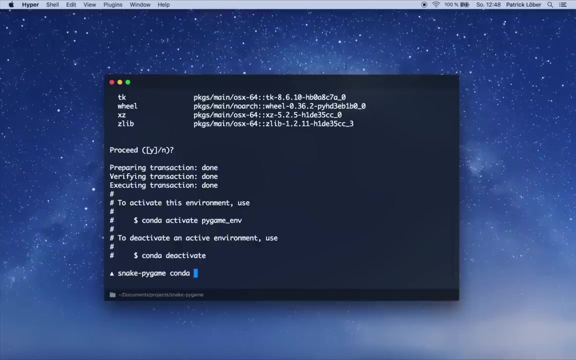 virtual env, But I recommend to use a virtual env. And now let's create a virtual env with conda, create minus n and then give it a name, for example pi game n. And I also say: I want Python equals 3.7.. Alright, so now this was created, So now we want to activate it with 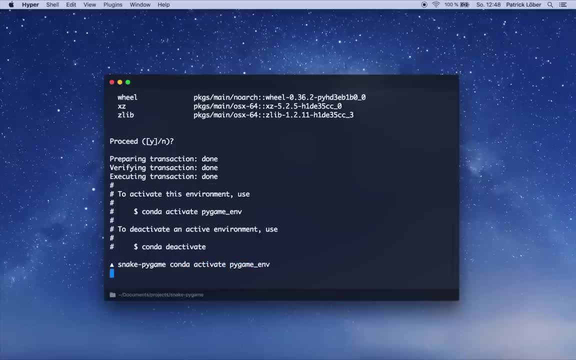 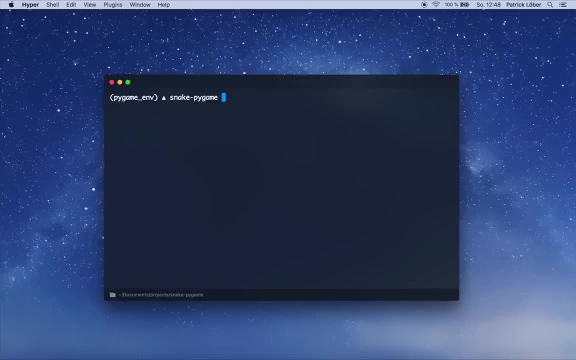 conda activate and then pi game n and hit enter And then we see the name of the environment in the front. So this means that we activated it successfully And now we can start installing all what we need. So the first thing we want to install is pi game for our game. So pip. 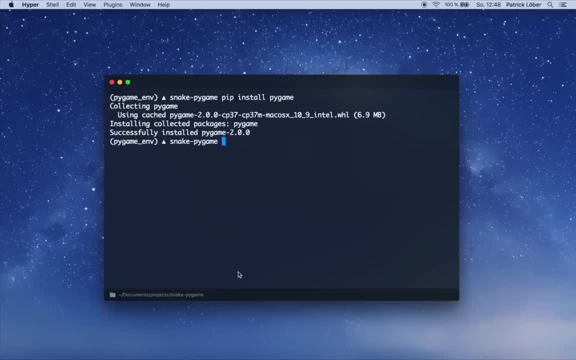 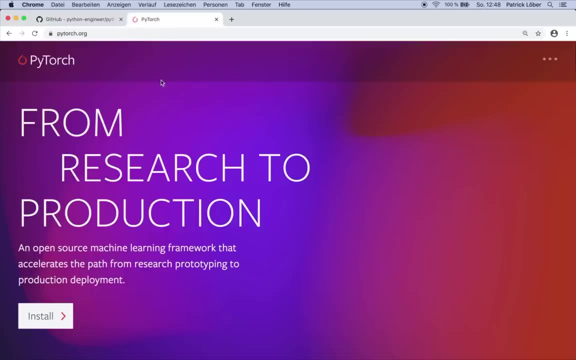 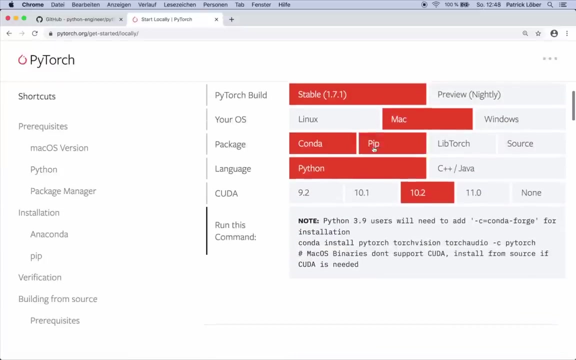 install pi game and hit enter. So this is done. The next thing we need is pi torch for our model later. So for this we can go to the official homepage and on install, And then here you can select your operating system. So I use Mac. 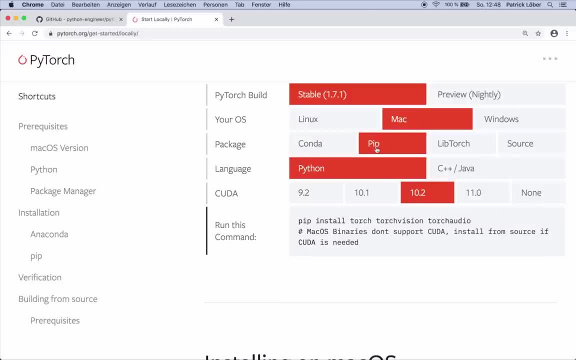 And I actually I want to say pip install and we don't need CUDA support, So only a CPU is fine. And we don't need torch audio because we don't work with audio files. So we can only grab this pip install, torch, torch vision and then paste that in here and hit enter, And now this installs. 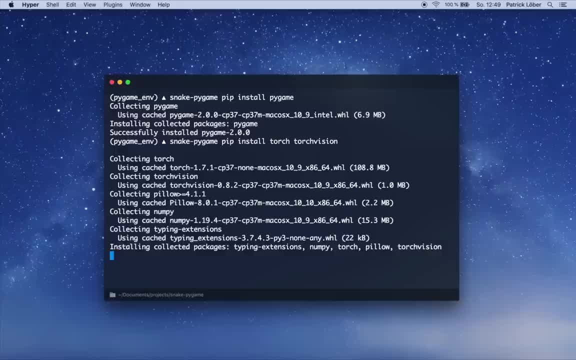 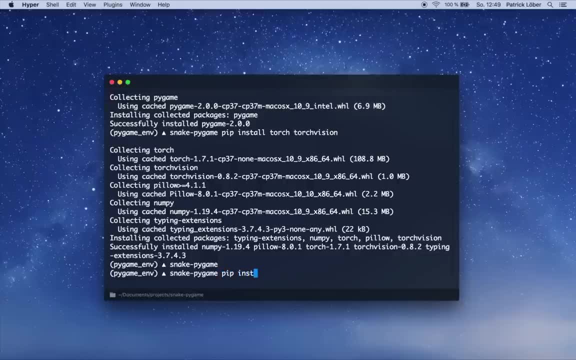 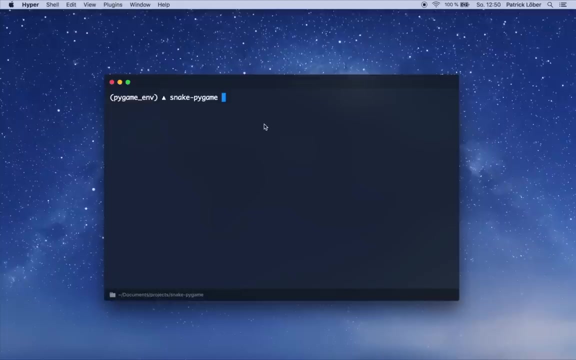 pi torch and all the dependencies. Alright, so this is done, And then we need to install the mod plot lib, And we also want I Python and then hit enter. Alright, so this was successful as well, And now we have everything we need. So now we can start implementing all the codes And, as a 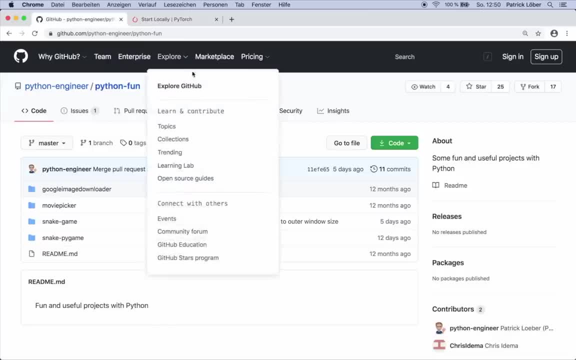 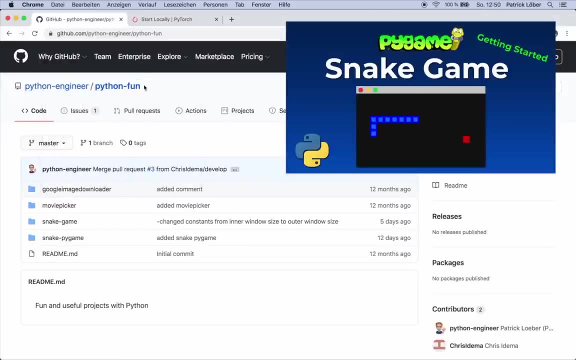 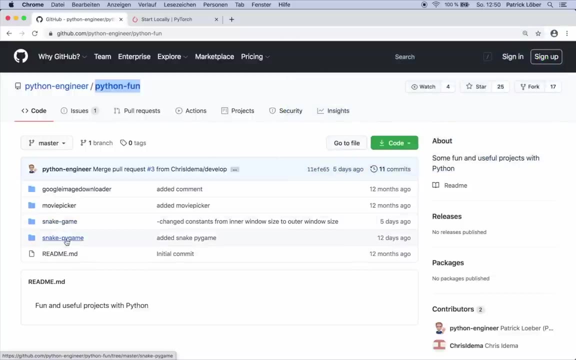 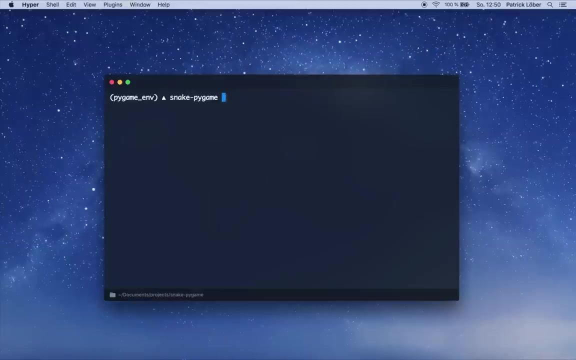 starting point. I want to grab the code from another tutorial that I did, So you can find this on GitHub And then on my account and then in the repo Python fun, And here I actually have two snake games, So, and then we need this one snake pi game and download this. So you can do this, And I already did this. 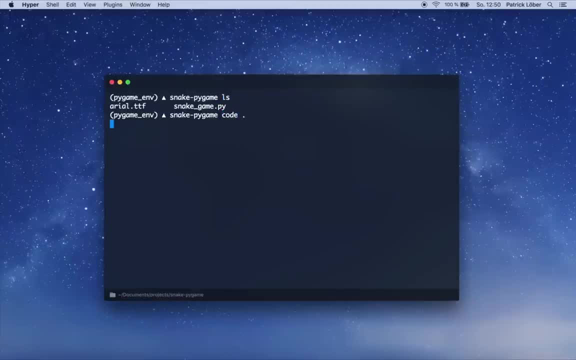 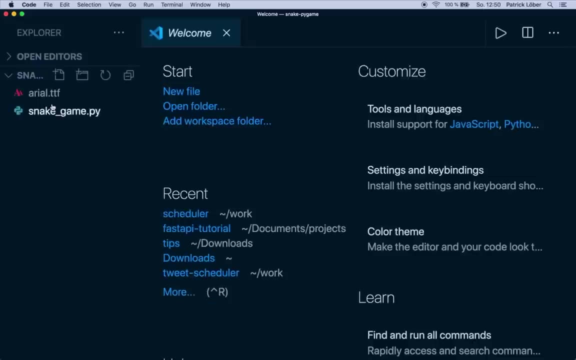 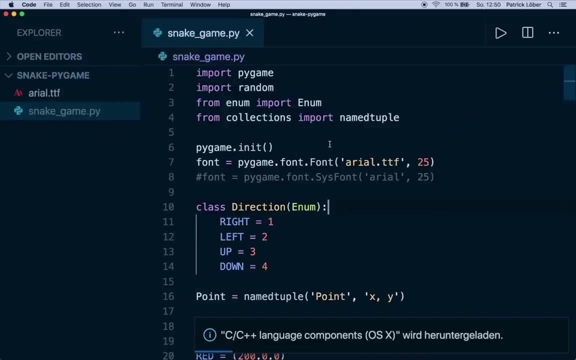 and have this here. So if we open up the editor- here I'm visuals, using Visual Studio code- then we can see we have exactly those two files. And then the first thing I want to do is I want to run this file and test if this is actually. 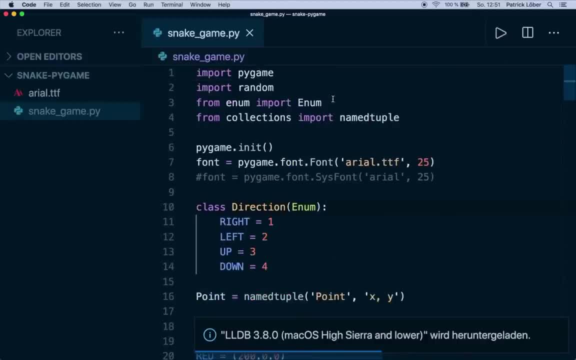 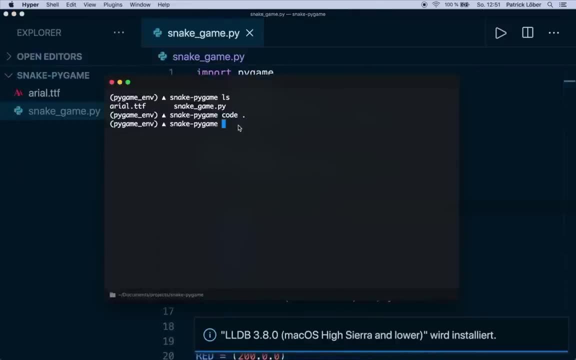 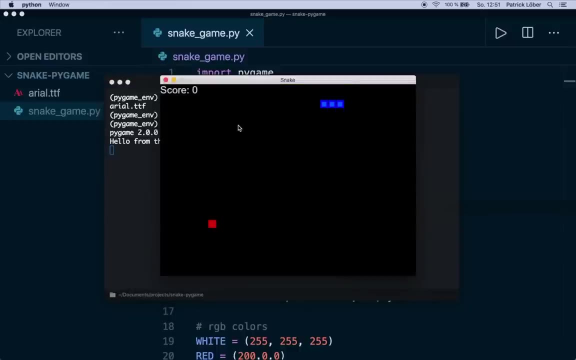 working. So right now, this is just a normal snake game that you have to control yourself, So you have to use the arrow keys. So let's say Python snake game, dot, pi, and then let's hope that this is working. So yeah, so now I. 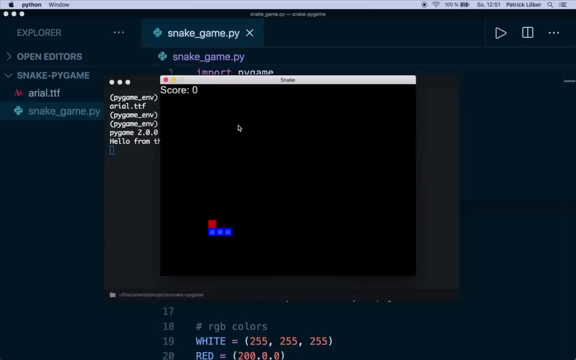 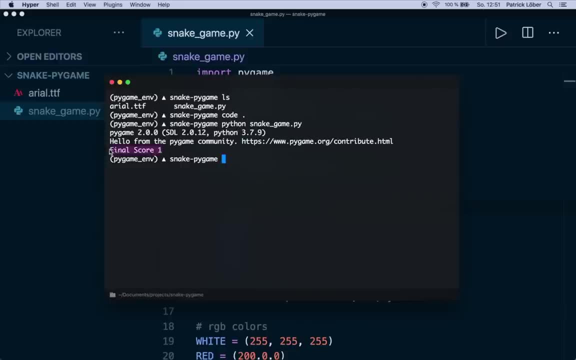 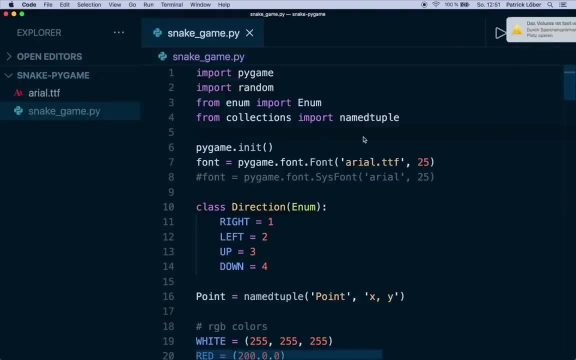 can control. this can control the snake, And I hope that I can eat the food, Yes, And now if I hit the boundary, then we are game over. So this is working, our environment is set up And now we can start implementing our code So we can change this so that we can use this as a AI controlled. 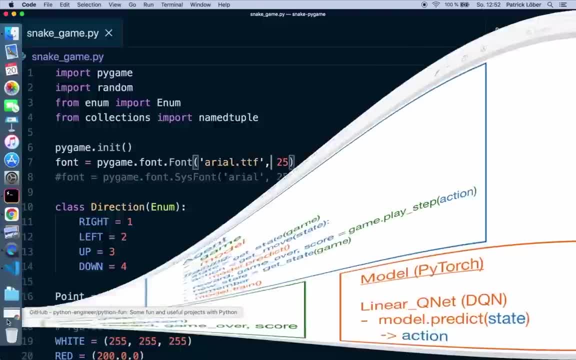 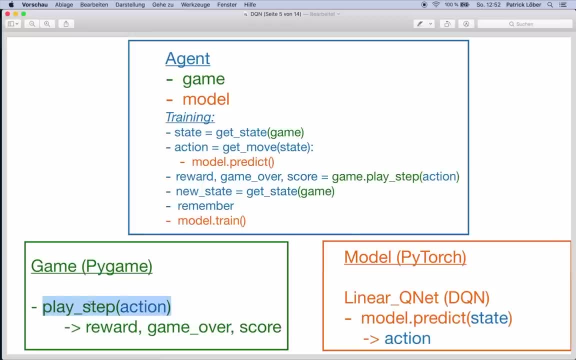 game. So let me show you the overview from last time. So last time I told you that we need a play step in our game And this gets an action And based on this action, we then take a move and then we must return a reward. the game overstate and the current score. 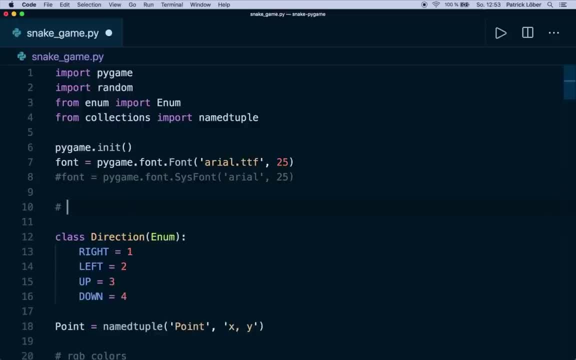 So first let's write down all the things that we need to change here. So first we want to have a reset function, So after each game our agent should be able to reset the game and start with a new game. then we need to implement the reward that. 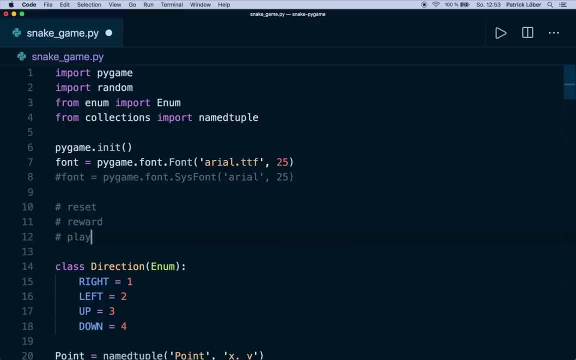 our agent gets, then we need to change the play function so that it takes, takes an action and then returns a or computes the direction. then we also want to keep track of the current frame, or let's call this game iteration, And for later we also need to have a change. 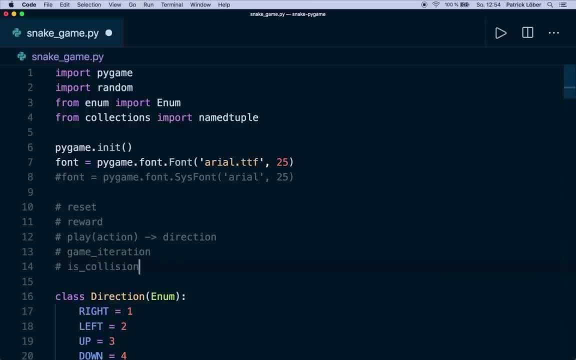 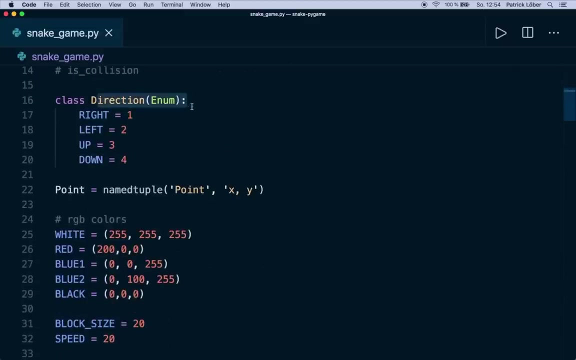 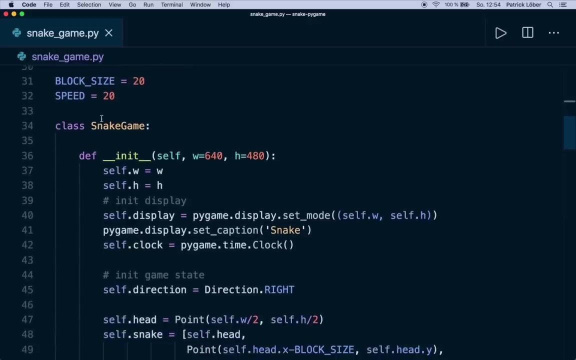 in the if is collision function to check if this is a collision. So first let's let me go over over this code quickly. So what we do here is we use pi game, then for the direction we use an enum, then for the point we use a named tuple, And then here I created a class snake. 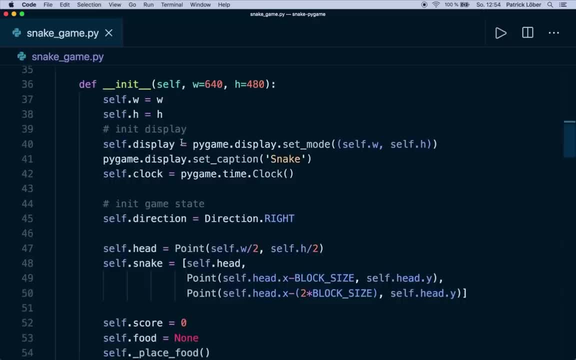 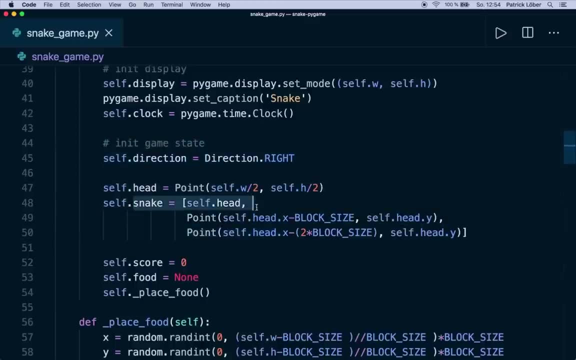 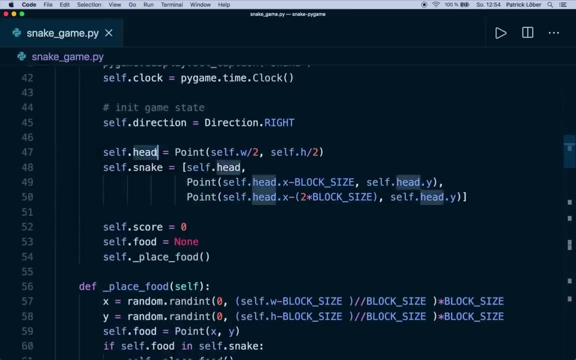 game, And here we initialize the things we need for the game. So here we initialize the game state. for example, for the snake we use a list with three initial values And the head is always the front of this list. then we keep track. 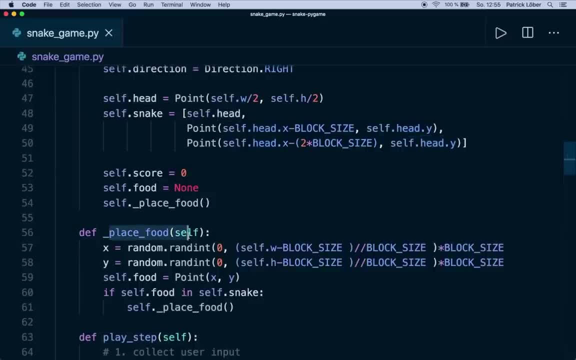 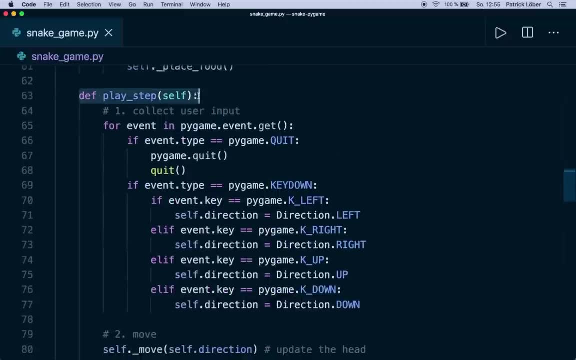 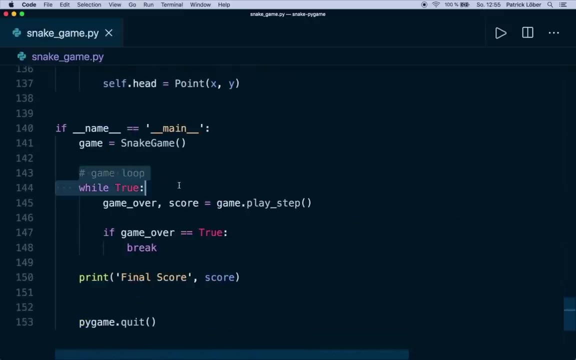 of the score. And here we have a helper function to place the food And, yeah, and we already have a function that is called play step, And then, if we go down to the very end, so here we have our game loop. So, while this is true, we take a game or a play step And 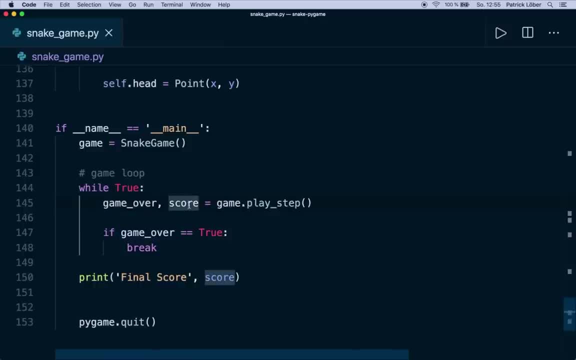 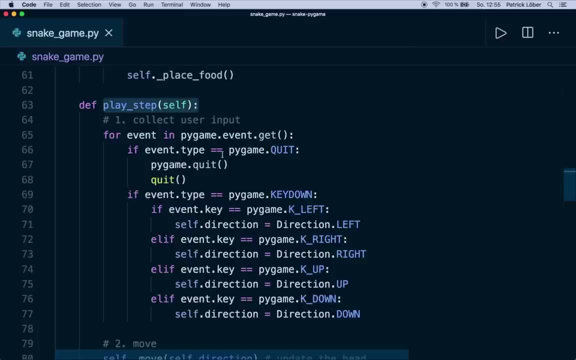 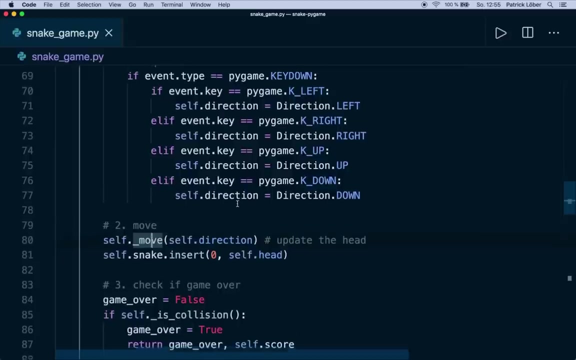 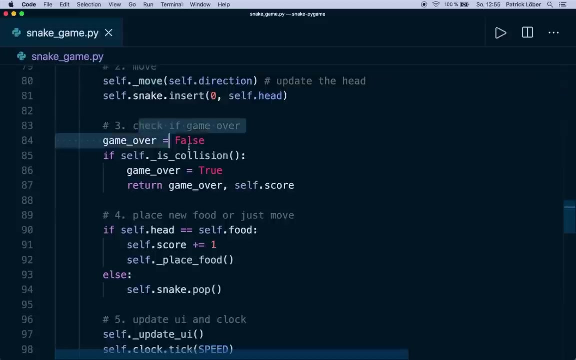 we get the game over state and the score. So this place, the function, is the most important one. So here, first we, right now we grab the user input, So the key we press, then we calculate a move based on this key And then we update our snake and check if we are game over And 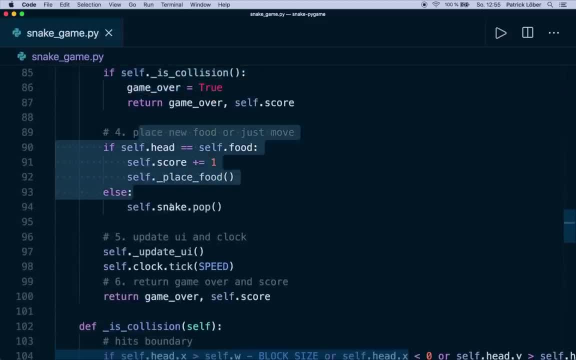 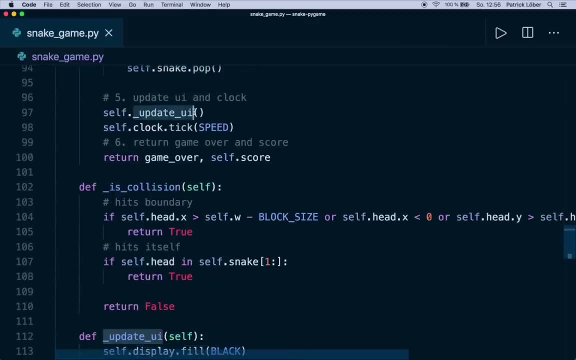 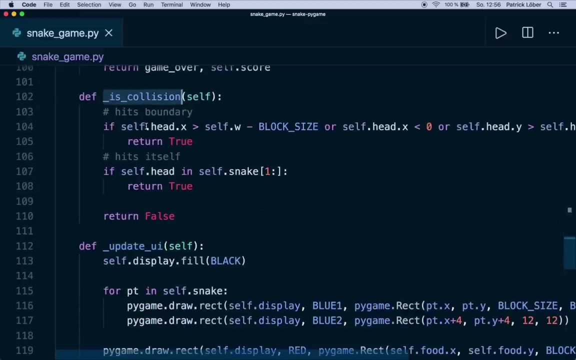 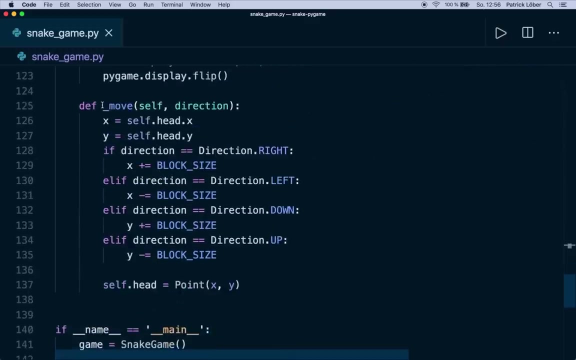 if we can continue. we place the new food or check if we eat the food, And we update our UI with this helper function- update UI. then here we have: this helper function is collision, where we check if we either hit the boundary or we run into ourself. And then we also have this helper function, move, where we get the 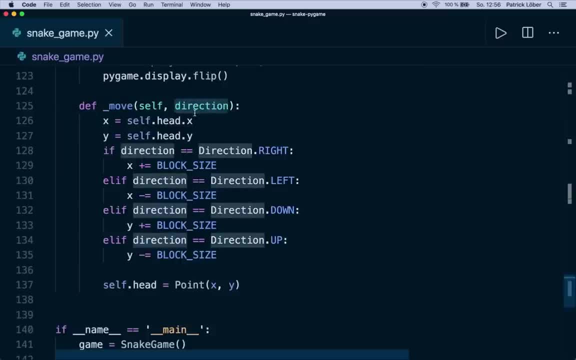 current direction And then, based on this direction, we simply add a move based on the current direction And then, based on this direction, we simply add a move based on the current direction And then, based on this direction, we simply add a move based on the current direction And then, based on this direction, we simply. 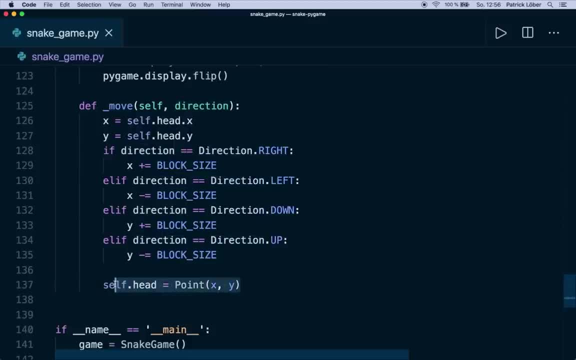 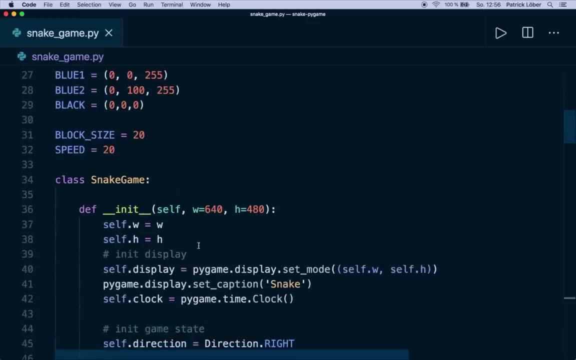 change, keeping the current direction, Running the need for the new properties for, however you put it, if the further It is, I would say, smallest when you add of when you add all the different types of properties in the previous drive and then, after you do, your additional management for. 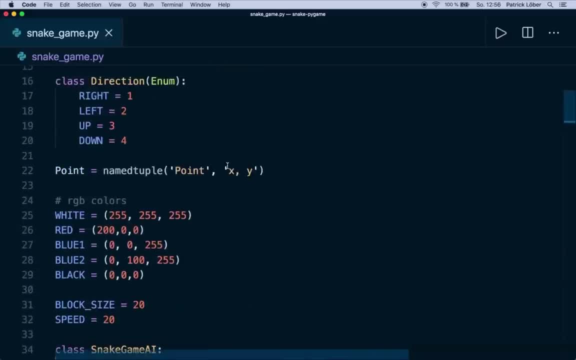 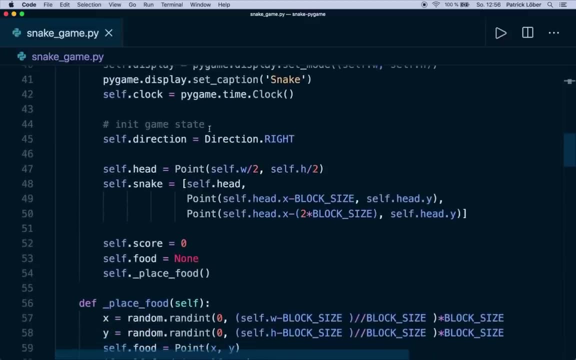 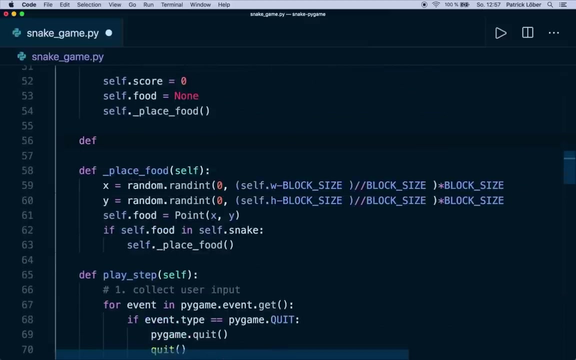 the initial drive. you change the number of wäh біль Otterp enrollment to is data. it won't change anything here. I already have this comment where we in it the game state. So now we want to refactor all of this into a reset function. So we create a new function, define, And then let's call. 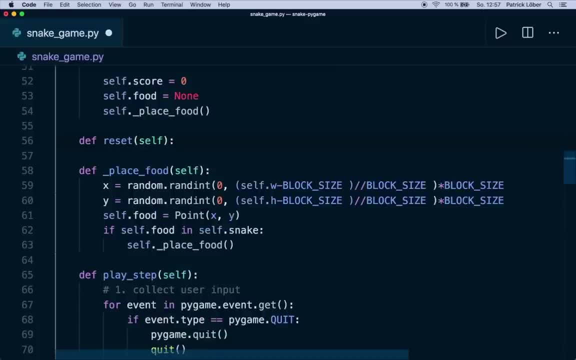 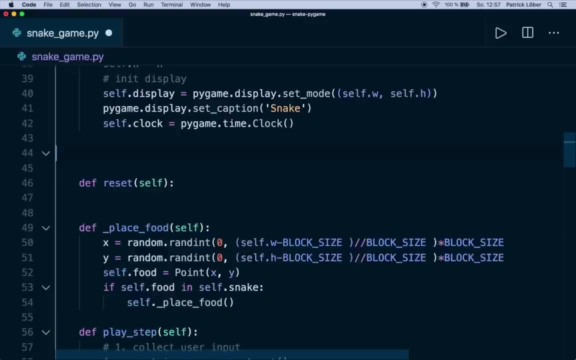 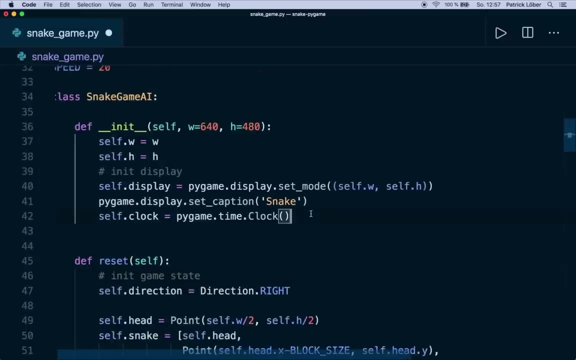 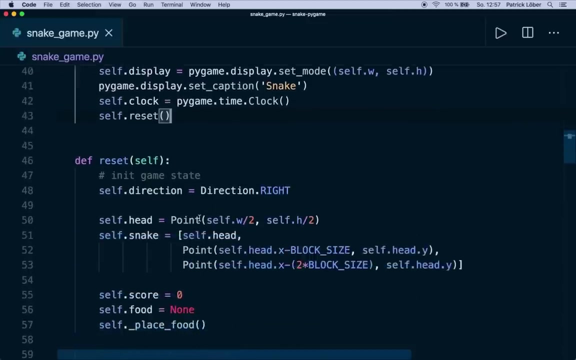 this reset and it only gets self and no other arguments. And here we can grab all of this code and then simply paste it in here And in our initializer. we then call self dot reset. So this is the first thing we need. Additionally, we want to keep track of the. 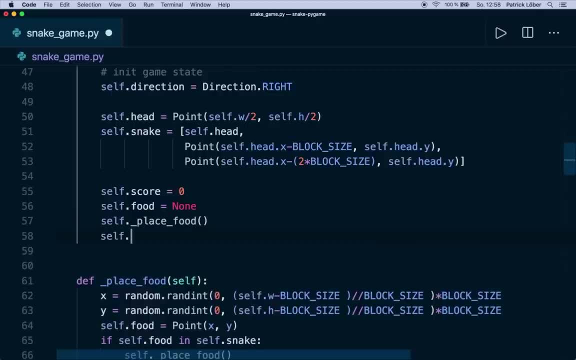 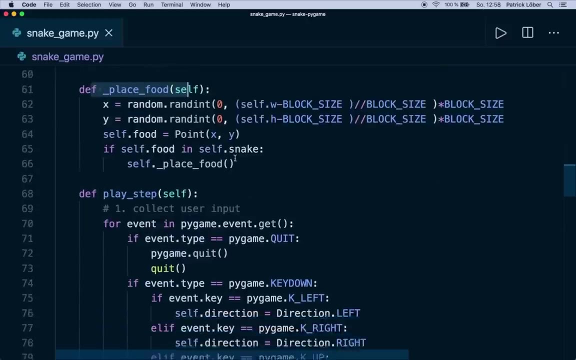 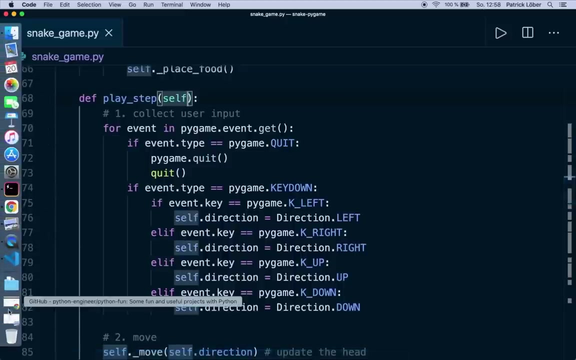 game iteration or frame iterations. So let's call this self dot frame iteration iteration. and in the Big, The big one beginning, this is just zero. then there's the fine place: food can stay as it is. And now we need to change the place that function. So first of all, if we have a look at the 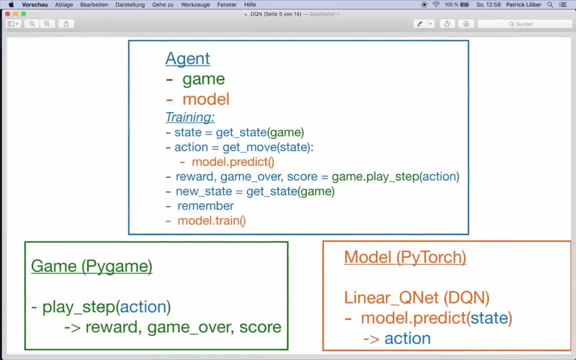 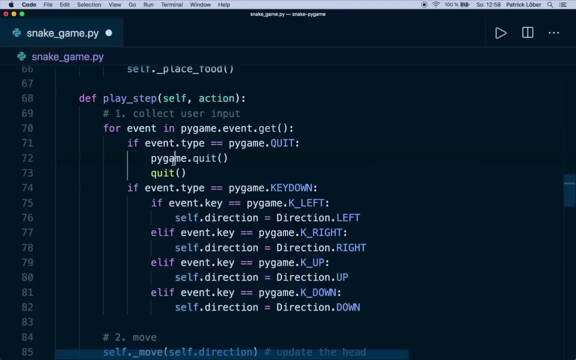 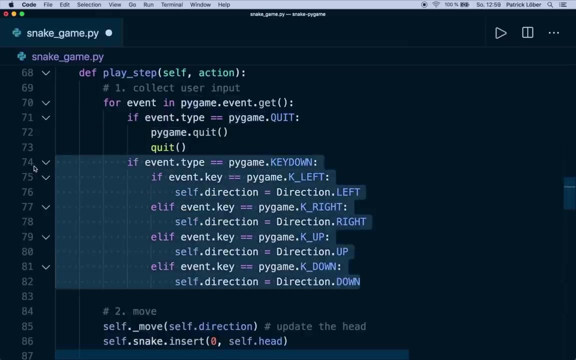 overview here. I already told you that now we need to give this the action from the agent and we need to return a reward. So let's start by using this action parameter And here we grab the user input. So actually, right now we can get rid of this. So the only thing- 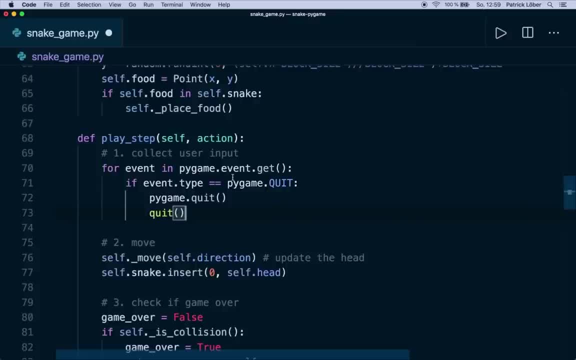 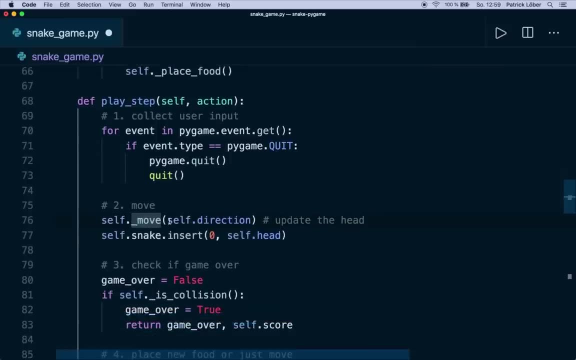 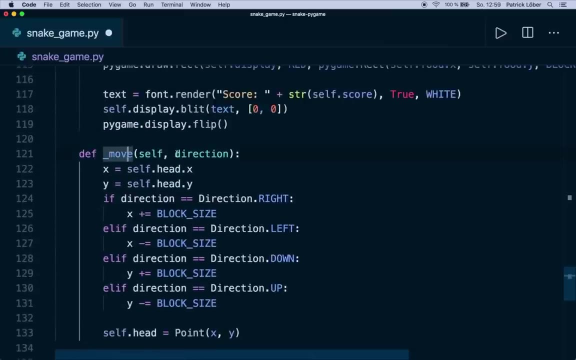 we still check if we want to quit the game. And now here we already have this helper function where we move in the current style direction. So actually, what we change here? now, this move function doesn't get the direction from the user input. So now here it gets the action, and then we have to determine. 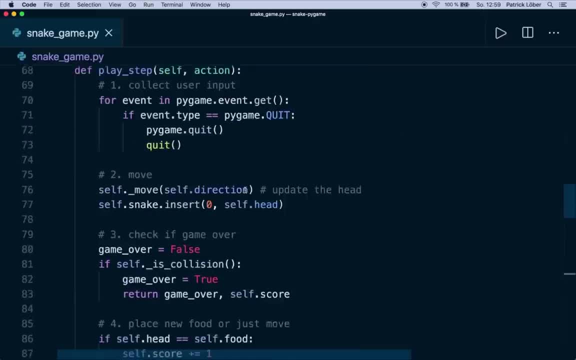 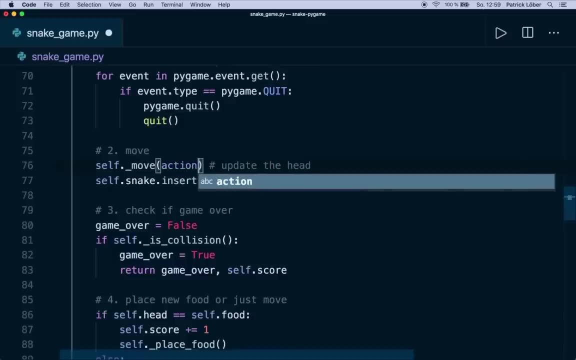 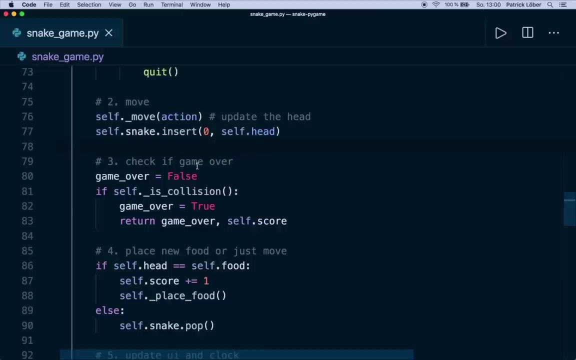 the new direction. So we do this in a second, But first let's only change this, And then here we call the self dot move with the action, And then we update the hat, then we check if we are game over or not, And we actually now we also need the reward. So we simply say: 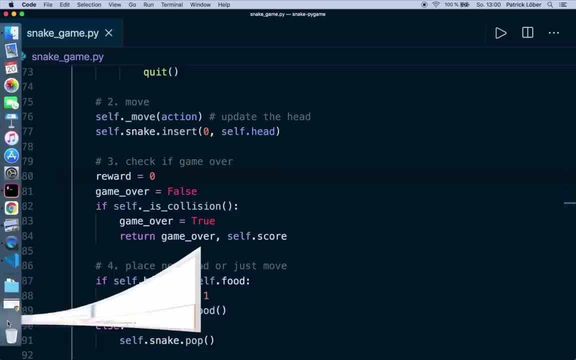 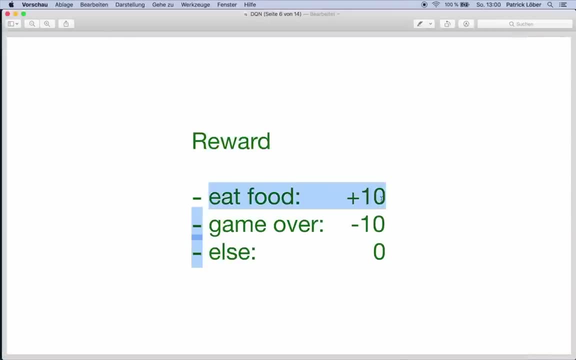 reward equals zero. And let's go back to the slides from last time. So the reward is really simple. Whenever we eat a food, we say plus 10,. when we lose or when we die, then we say our reward is minus 10.. And for everything else we just stay at zero. So we initialize: 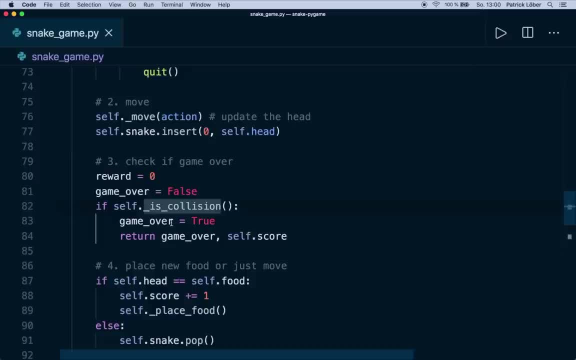 the reward with zero, Then if we have a collision and game over, then we say our reward equals to minus 10.. And we want to return this as well. So return the reward game over and self dot score. And here we check only if we have a collision. So here I actually want to do another check. 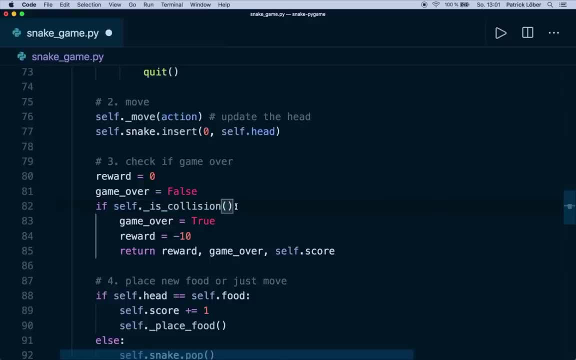 So if nothing happens for a long time, So if our snake doesn't improve and doesn't eat the food but also doesn't die, then we also want to check this, And if this happens for a too long time, then we also break here. 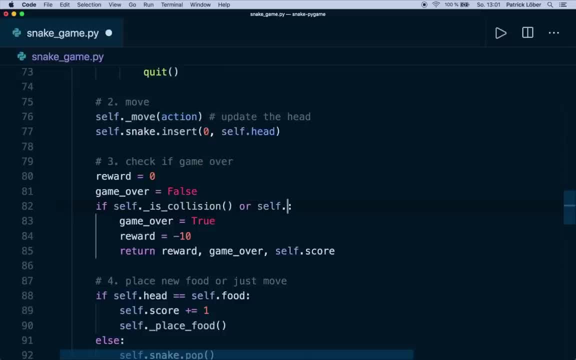 So we can say or. and then here we say: if self dot frame iteration, and if that this gets too large with out anything happening, then we stop here. So here I use this little formula: if this is greater than 100 times the length of our 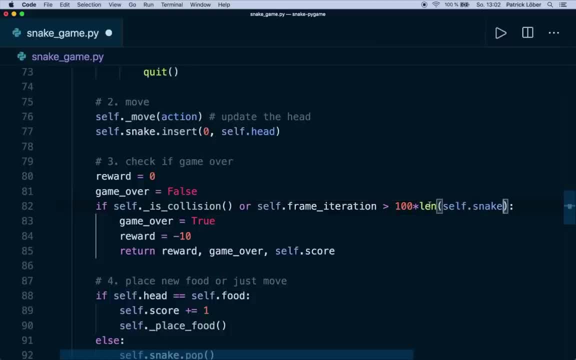 snake. so remember, this is a list- then we break. So this is also like this. then it's dependent on the length of the snake. So the longer our snake is, the more time it has. So but then if it gets larger than this value, then we break. 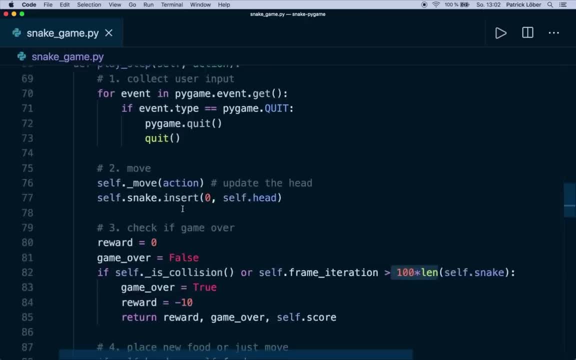 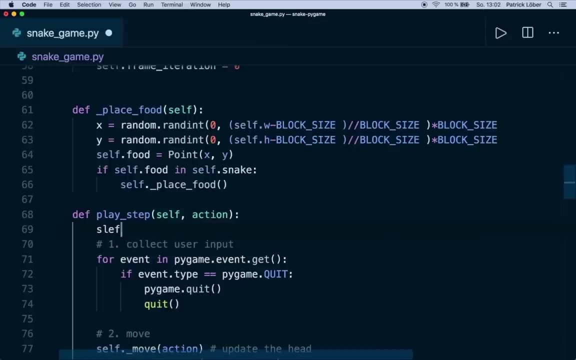 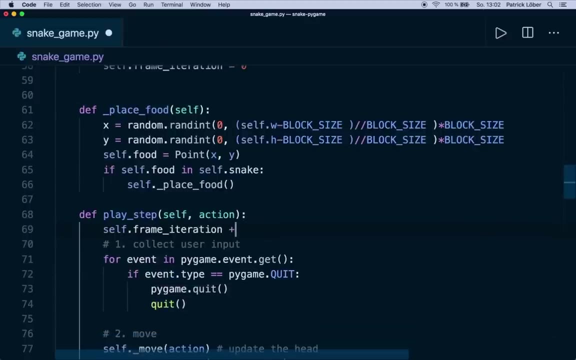 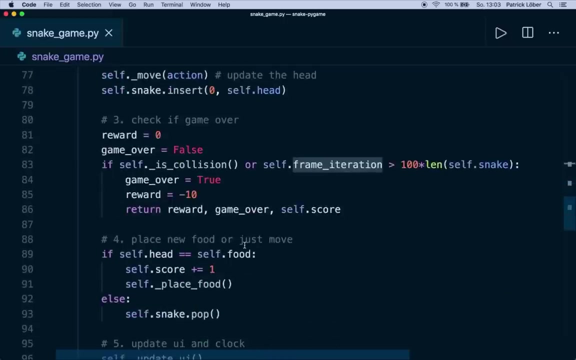 And of course we have to update the self dot frame iteration And we can simply do this here at the beginning. So for each place that we say self dot frame, iteration plus equals one, And when we reset it, then we reset it back to zero. So this is here, And 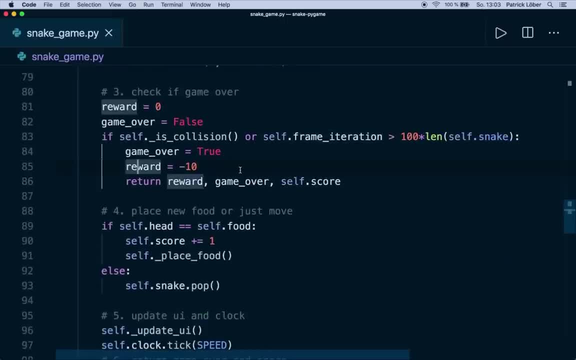 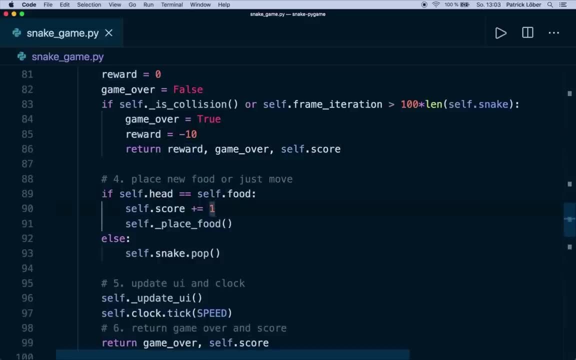 then yeah, if we stop, we have the reward minus 10, then here, if our hat hits the food, then we eat the food, So our score increases and our reward is set to plus 10.. Then we place a new food and say: otherwise we remove. 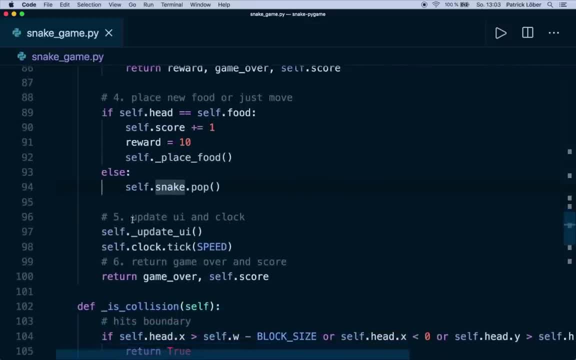 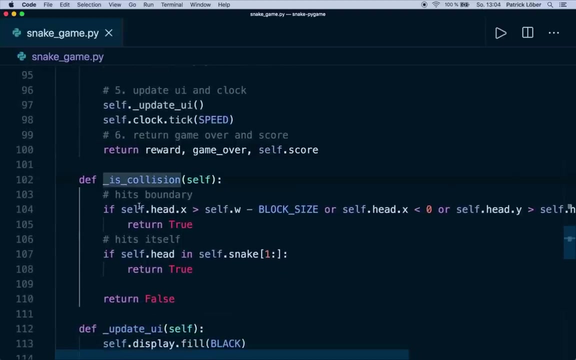 the last part, So we simply move here. then this can stay as it is, the update function, And at the very end we also want to return the reward. Then for the this collision function, we need a slight change. So here I only check for self dots. 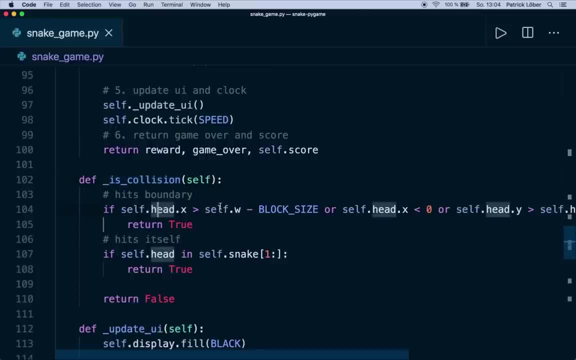 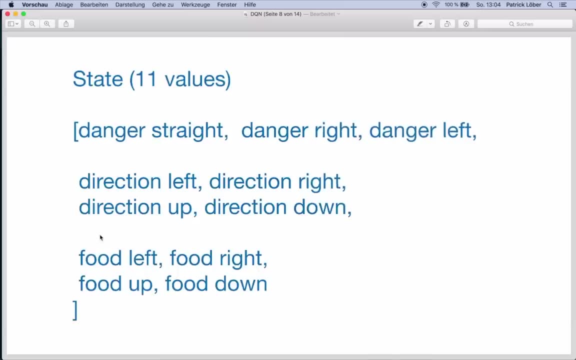 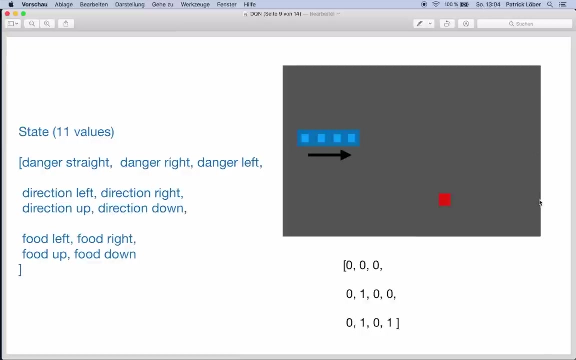 head, but later to calculate the state or the danger which I told you about. So if we have a look at the state, so here we calculate the danger. So if we are, for example, if we are here at the corner, then we have a danger at the right. 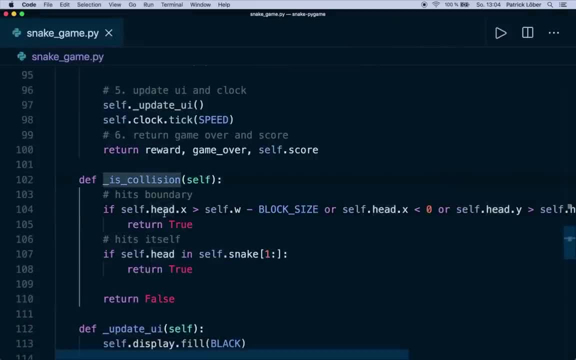 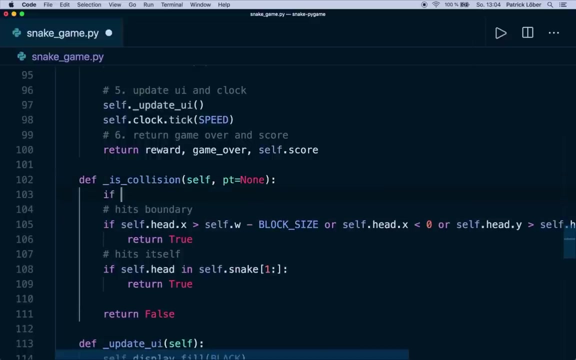 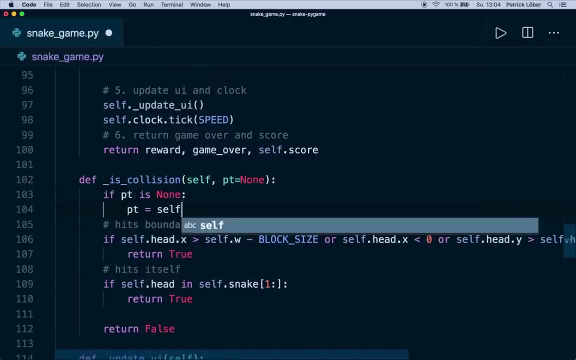 So for this it might be handy if we don't use self dot het inside here. But if we give this function a point, so this gets the point argument and let's say by default: this is none. And then here we simply check: if the point is none, then we set the point equals to self. 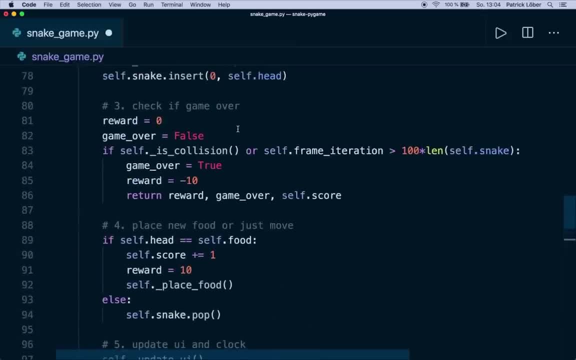 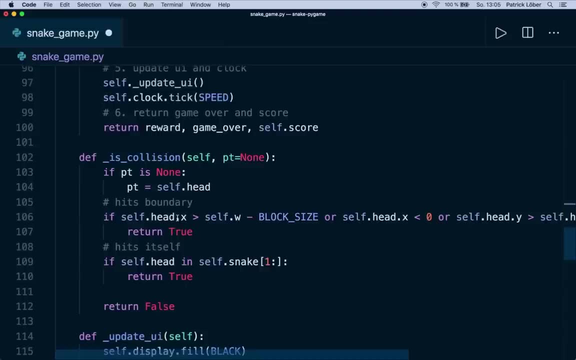 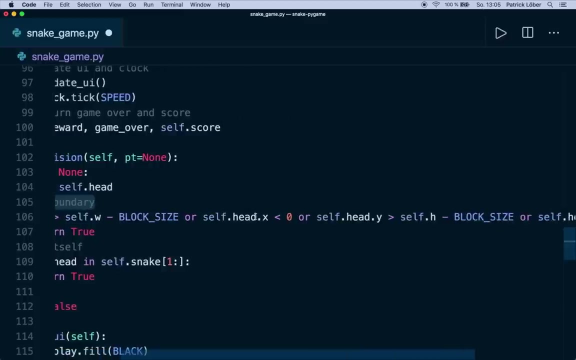 dot het. so inside this, where we call this with no argument, it can stay as it is. And then here, of course, we have to change self dot hat to. this is now our point. So here, if we hit the corner, point here and point here, 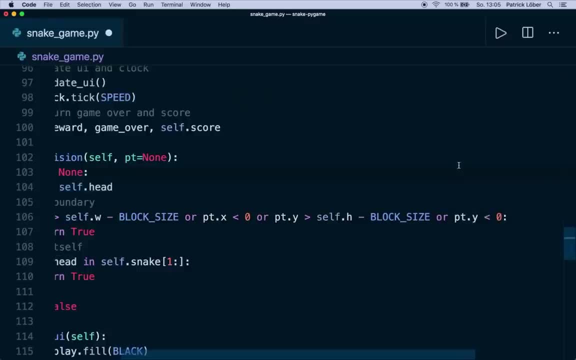 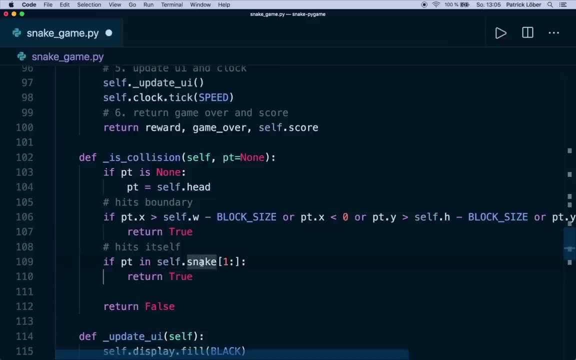 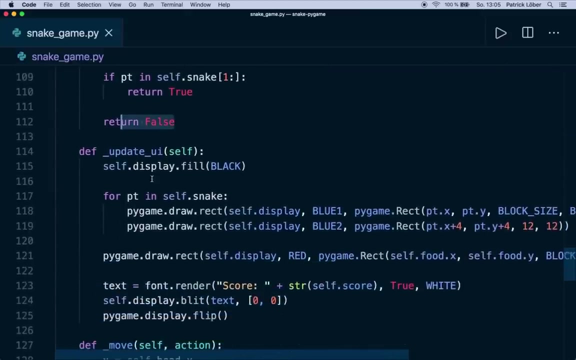 and point here, then we have a collision. And here, if our point is in the snake body, then we also have a collision, And otherwise we don't have a collision. Alright, so the update UI function can stay like this. And now for the move function. here we need to. 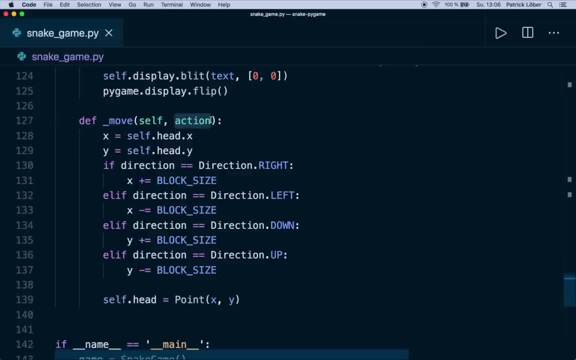 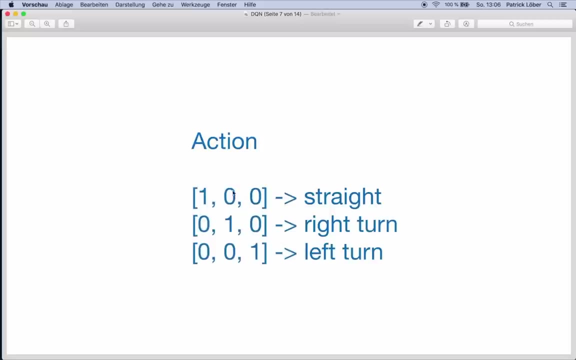 change some things. So now we get a action And now, based on this action, we want to determine the next move. So if we go back to the slides, so here, we designed the action like this, So it has three values: 100 means we keep the current direction and go straight. 010. 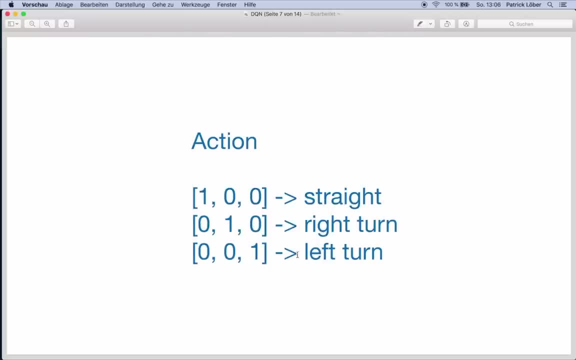 means we do a right turn and 001 means we do a left turn. So this is dependent on the current direction. So if we go right and do a right turn, then we go down Next. if we go down and do a right turn, then we go left next and so on, and left turn is the other. 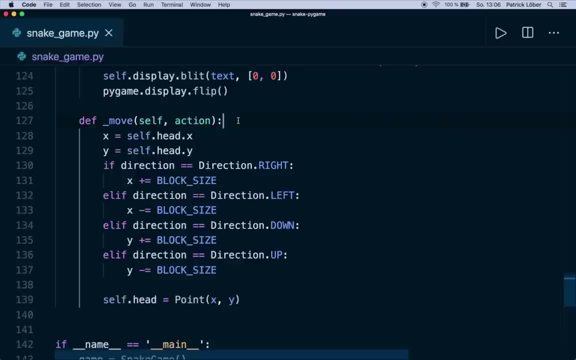 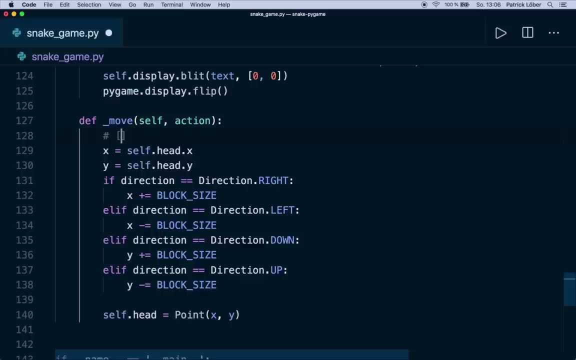 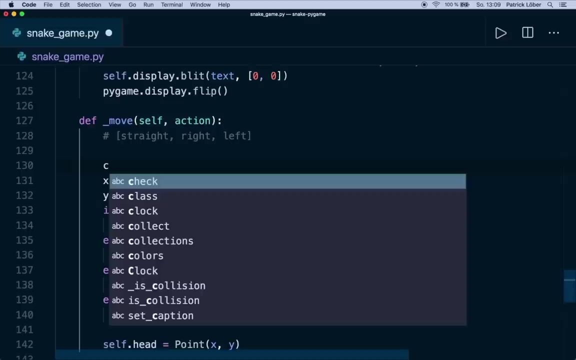 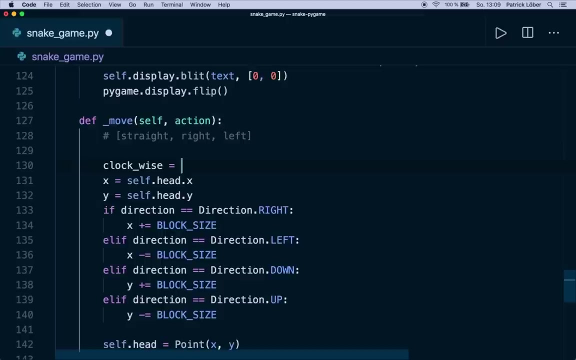 way around. So now we want to determine the direction based on the action. So let's write a quick comment here. we have straight right turn or left turn. So to get the next direction first I want to define all the possible directions in a clockwise order. So we say clockwise equals and then a list. And here 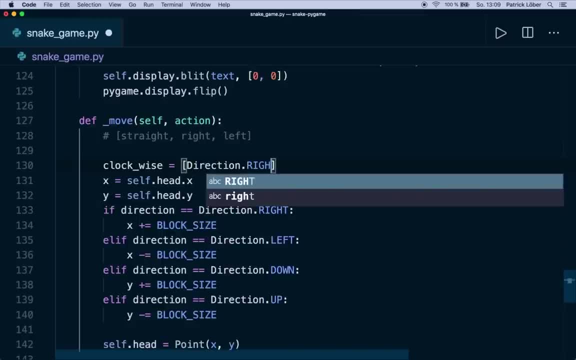 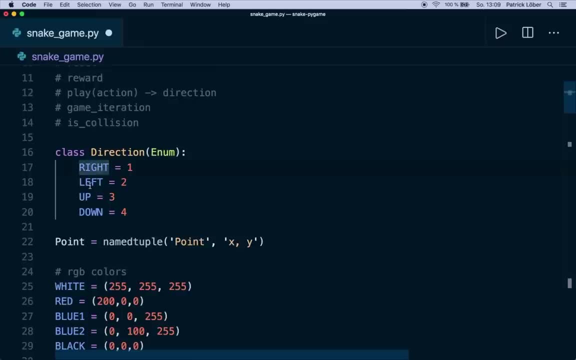 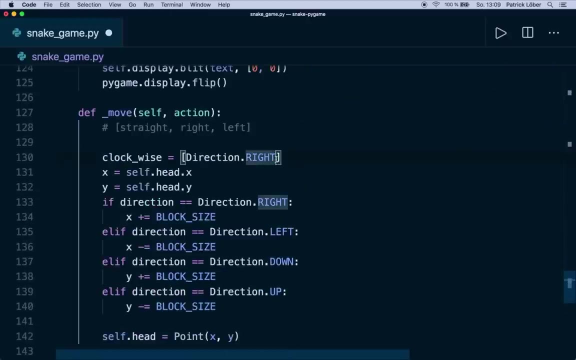 we start with direction dot right. So here remember for the direction we use this enum class, So it has to be one of those directions. So our clockwise directions should start with direction right, then form this on: the next one is direction dot down, then we have direction dot left. 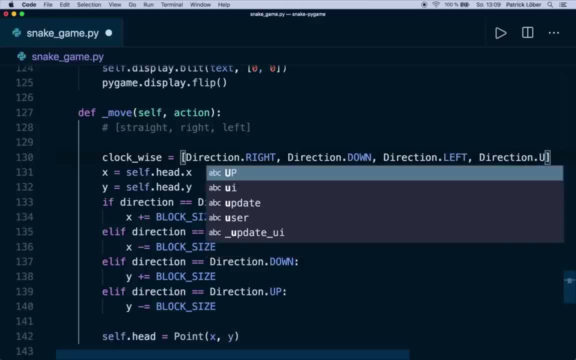 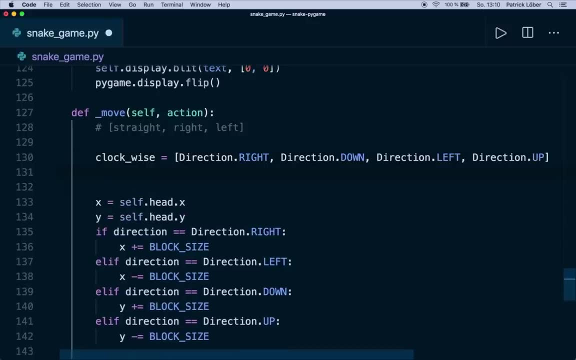 and as last thing, we have direction dot up. So right down, left up, this is clockwise And then to get the current direction or the current index of the current direction, we say index equals, and then we can say clockwise dot, index equals the up direction. So at the last one. now we're gonna talk, but we more on. So first we have index point left For the right one. puisque we have anenc on an educating, we say index equals and then we rick Stephens includes, but the direction, of course, because we have direction. thus, as the 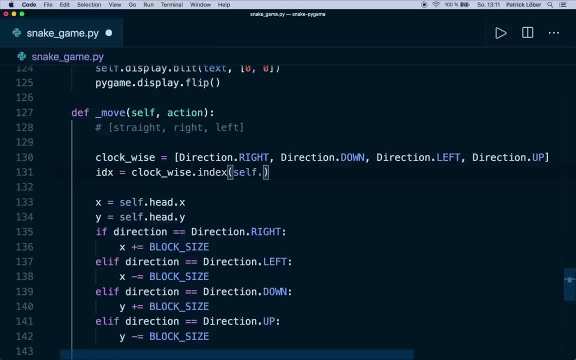 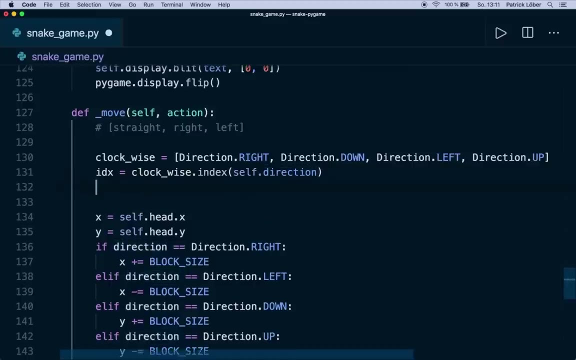 inch um behind us, house um. within that direction, we would write querting a search and then the index of the self dot direction. So we are sure that this has to be in this array, we, because the self direction must be one of those enum values. And then we check. 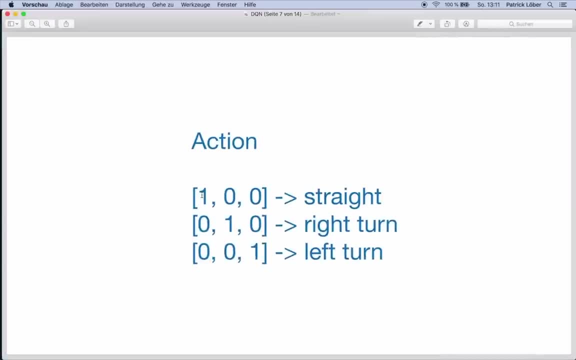 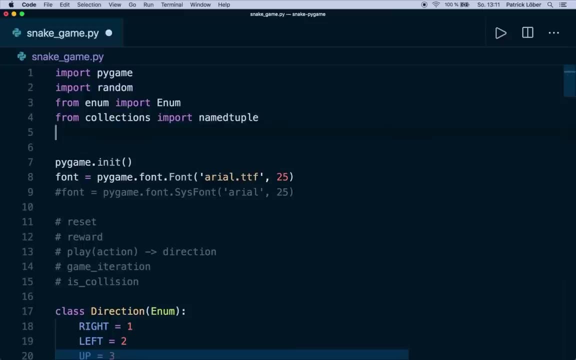 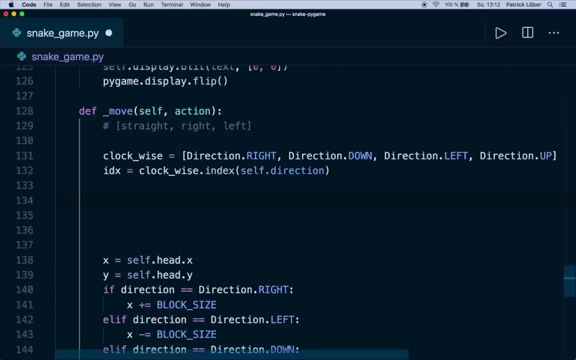 the different possible states, So these ones. So for this we can use numpy, And I guess we have to import numpy first as an P and then we can use it. Here we can say: if numpy, and then we use this function array equal, and then here we put in the action and the 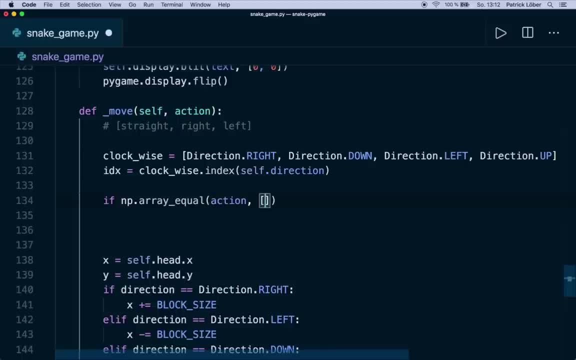 array that we want to compare. So if this is equal to 100, then we go straight or we keep the current direction. So we simply say our new direction equals, and then clockwise of the index, And then remember the index is just the index of the current direction. So here we basically. 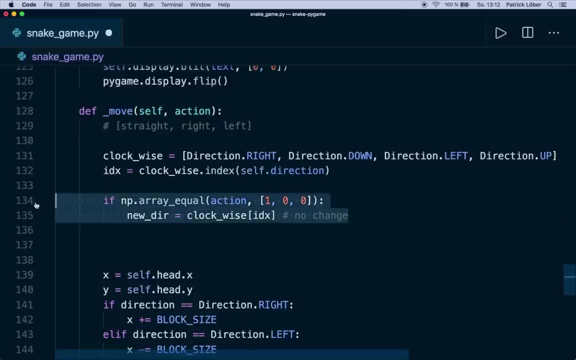 have no change, then we say l, if, if our array, if numpy array equal, if the action equals to 010, then we do a right turn. So this means we go clockwise. So if we go right then the next direction would be down. If we go down, then the next direction would: 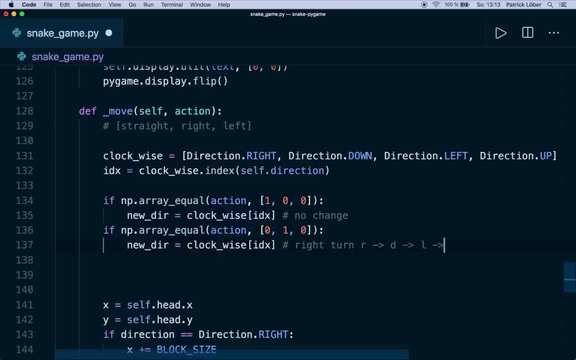 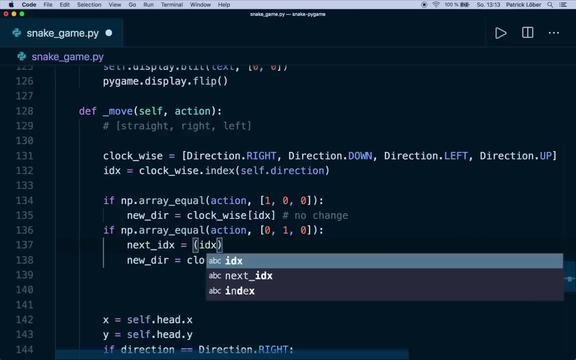 be left, And if we go left then the next direction would be up. So here we say index equals, or this is our next index Actually, and here we say this is the current index plus one, but then module four. So 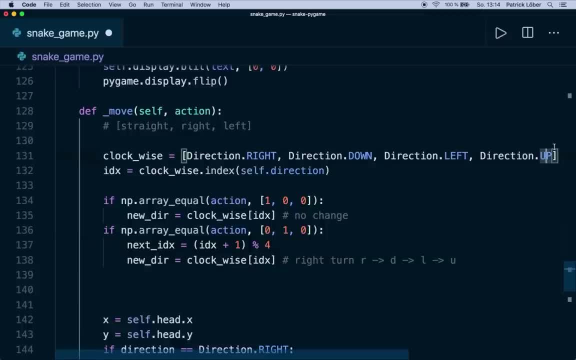 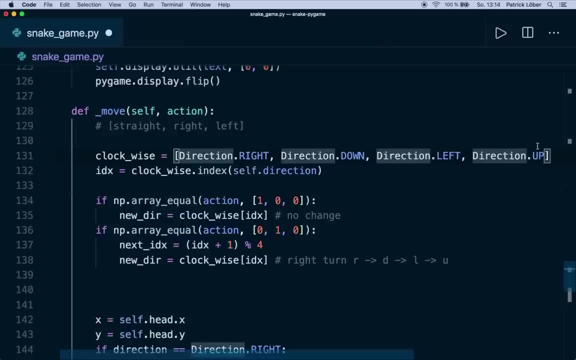 this means if we are at the end up and then do the next one, if we have index, so this is index 0123.. And then if we have index for module for is actually again index zero, again we do a turn and then come back at the front again. So this is our right turn. So now this: 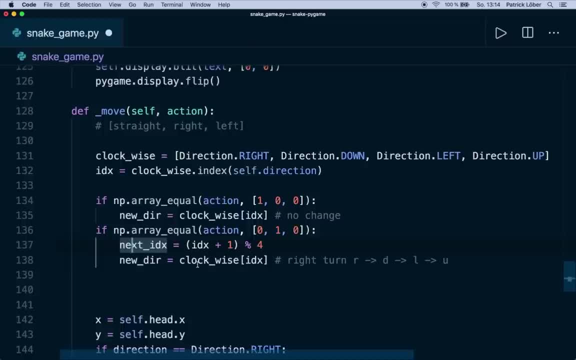 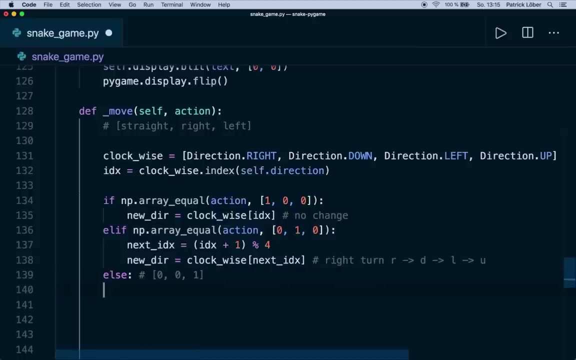 is the next index, And now our new direction is clockwise, of the next index And then otherwise we can simply use else here and actually change this to an L. if so, now this is the last case, So it has to be here, it has to be 001, and if this is the case, then let's copy and paste. 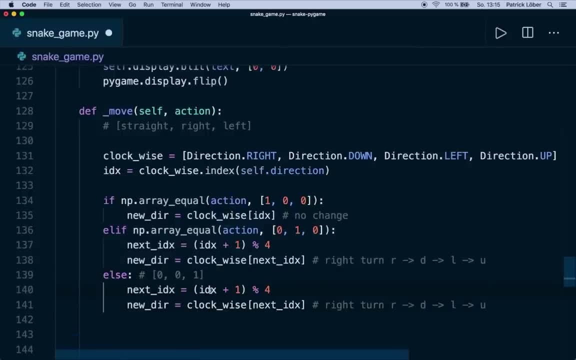 this in here. Then our next index is the current index minus one module of four. So this actually means we go counter clockwise, So we do a left turn. So if we start with right, then the next move would be up, And then the next would be left, and then the next would be down, and then right again, and so on. 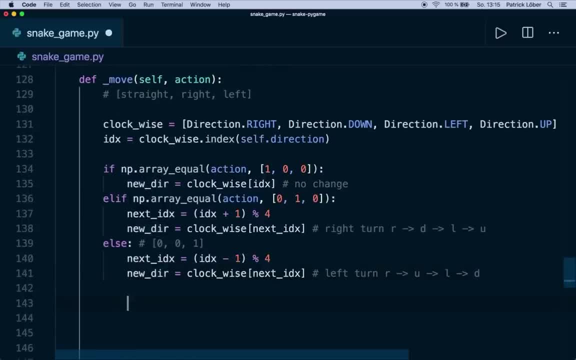 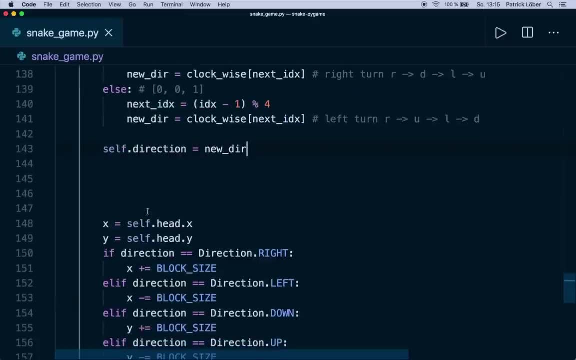 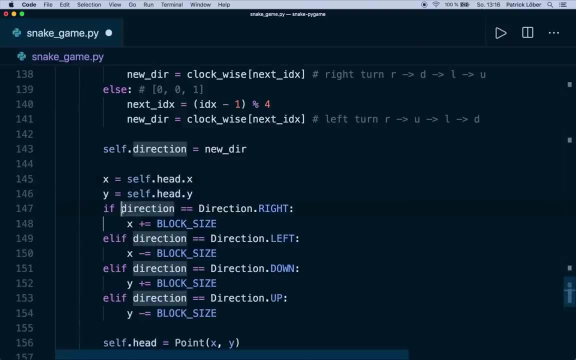 So now this is our new direction. And then simply we say self direction equals new direction, And then we go on. So here we extract the hat, And then here we have to check: if self dots direction now is right, then we increase the position of x, And so on. if we have the left direction, 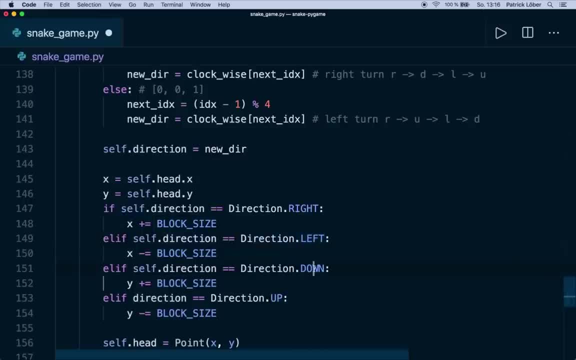 then we decrease x, And if we go down then we actually increase y. So for so the why starts at the top, at zero, and then increases if we go down. So if we go down then we have to increase y, And if we go up the y will stop. 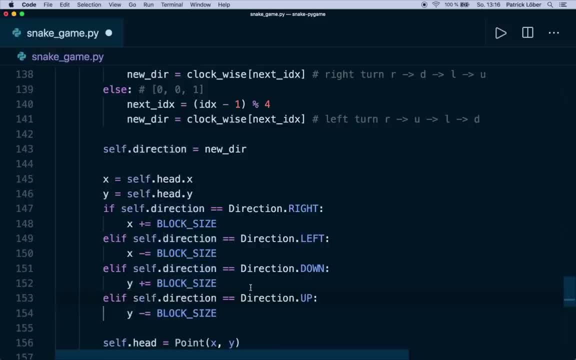 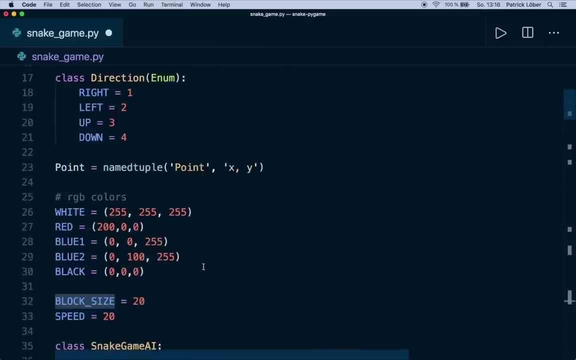 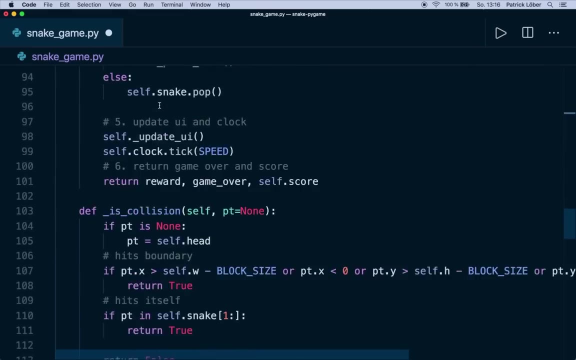 up, then we have to decrease y. So if self direction equals up, then y minus equals the block size And, by the way, the block size is just here, a constant value of 10.. So that's how big our one block of the snake should be in pixels. So yeah, this is everything. 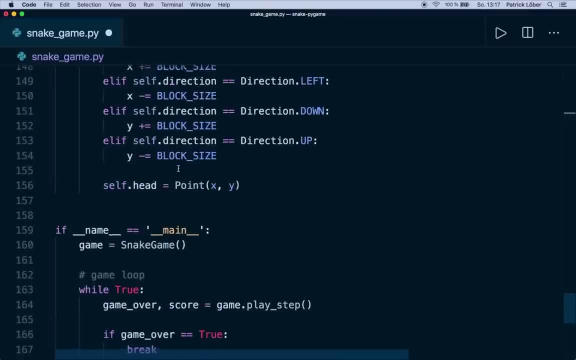 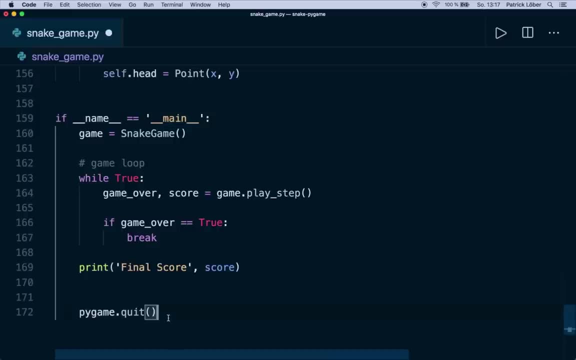 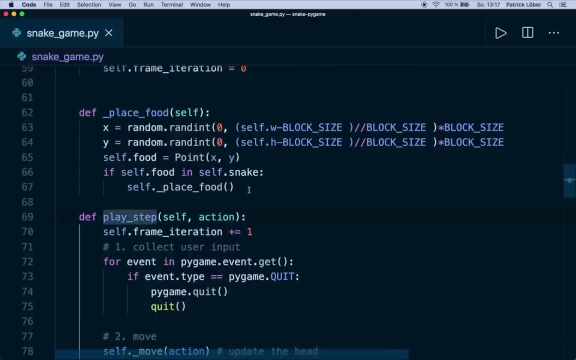 we need here in the move function, And now here we don't need this anymore. So this is actually no longer working with a user input. So you can just delete this And then later we control this class from the agent and call this play step function. So yeah, 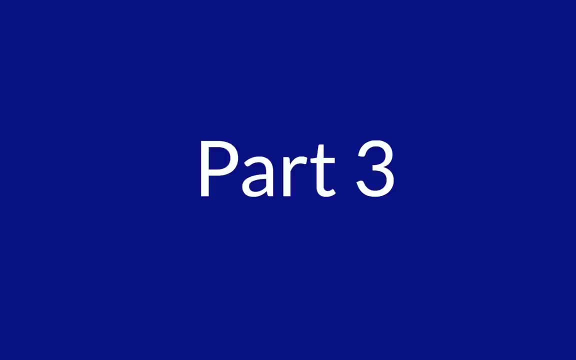 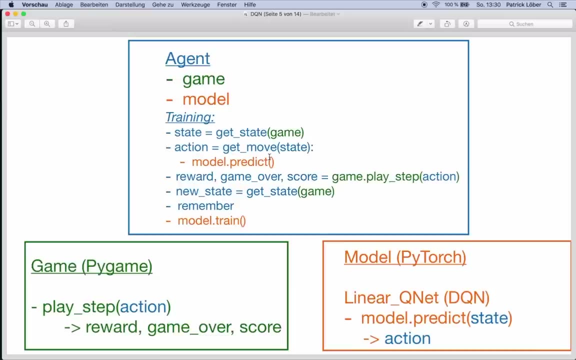 for now, this is all we need to implement the game. So I already talked about the theory of deep Q learning And the first part. in the last part, we implemented the pygame so that we can use it in our agent controlled environment. 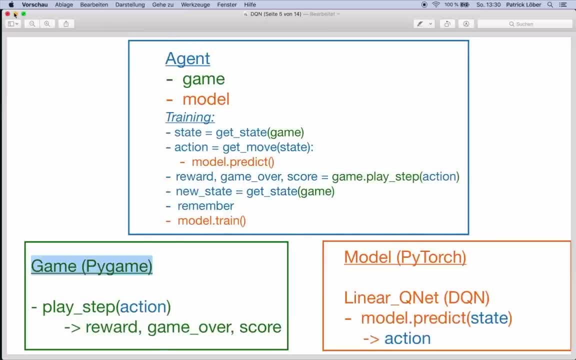 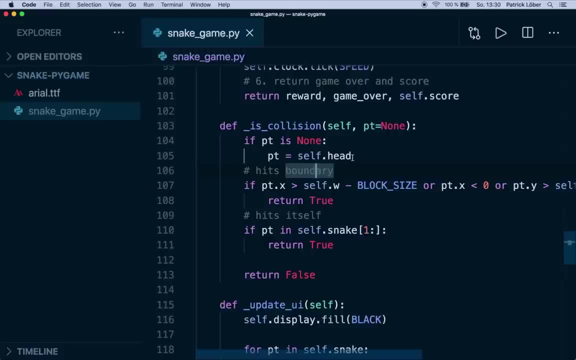 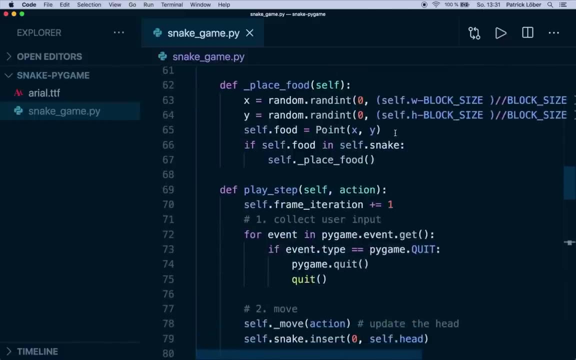 And now we need the agent. So let's start. And so here, if you haven't watched the first two parts, and I highly recommend to do so, So starting point from last time, and I actually want to make one more change that I forgot. 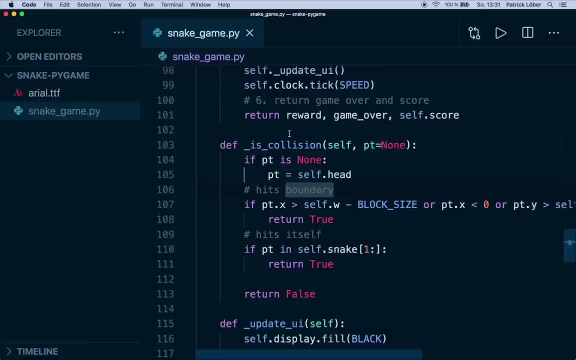 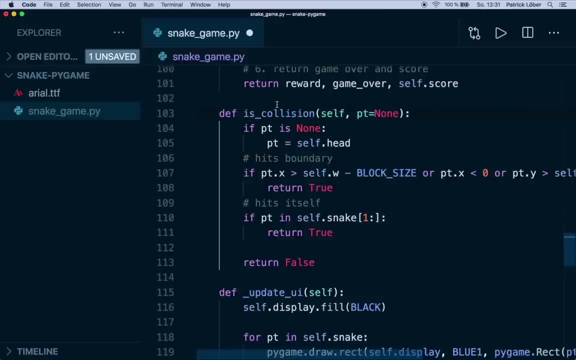 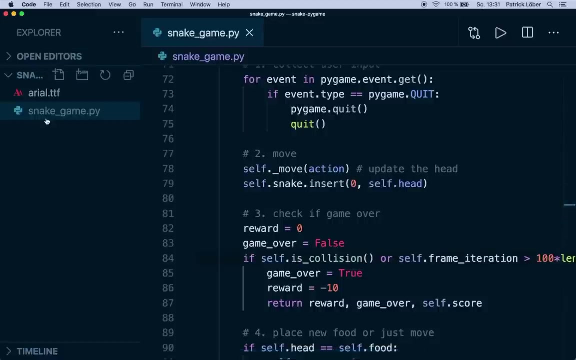 So here the is collision function should actually be public, because then our agent should use it. So just remove the underscore here and then also remove it in this class itself when we call this. So then we have our snake game, And I also want to rename. 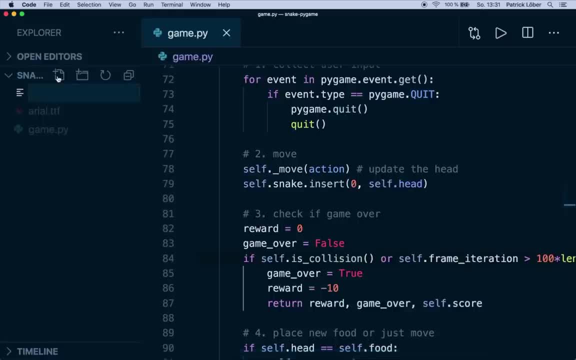 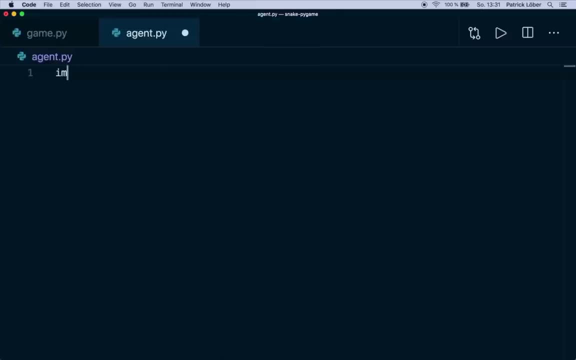 this to just be game, And now we create a new file agent, dot pi, and then start implementing this. So first here we import torch from pi torch, then we import random, because ran later we need this. then we also need import numpy as NP And from our implemented class. 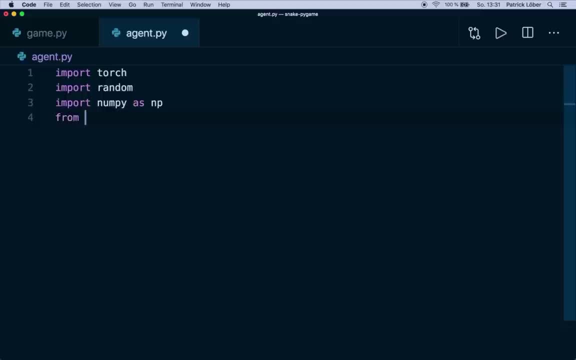 we need to the snake game. So we say from game import snake like snake game a I. So I think that's what we call this class: snake game a I. So yeah, that's the right name. Then we also. 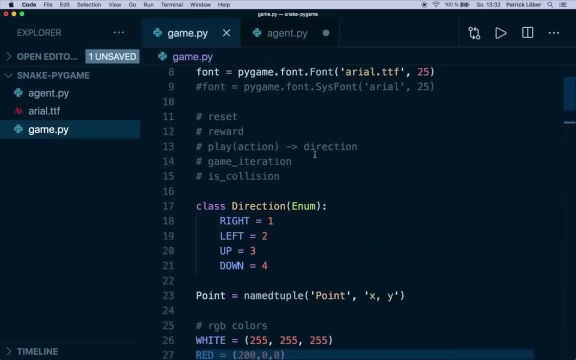 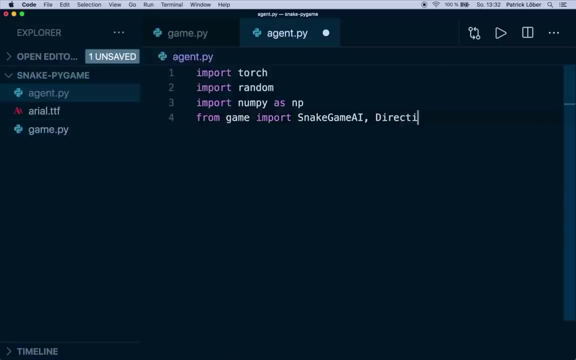 here at the beginning we defined this enum for the direction and this name tuple for the point, which has an x and a y attribute. So we also want to import these two things. So we import direction and we import point. And then we also say from collections we 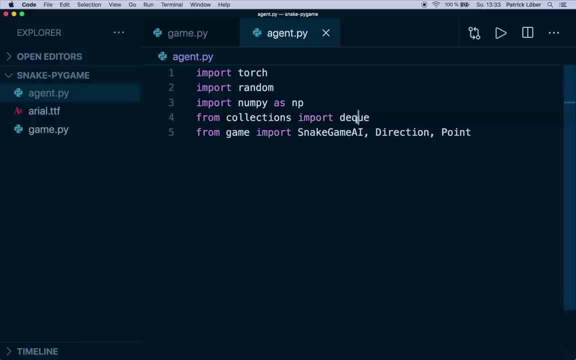 want to import deck. So this is a data structure where we want to store our memories. So if you don't know what a deck is, then you don't need to know what a deck is, And then we can sorry about that, But just know if we have a deck and we can store our memories in. 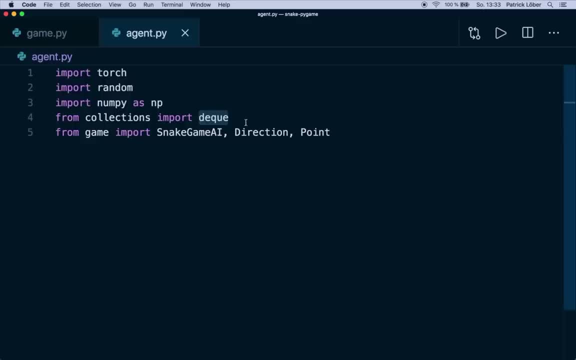 the future. use the, and then we can do an. I bet Let's say that it's a video class, it's a lecture class, And these are all the things I need, And then this way, it's going to be useful in this. 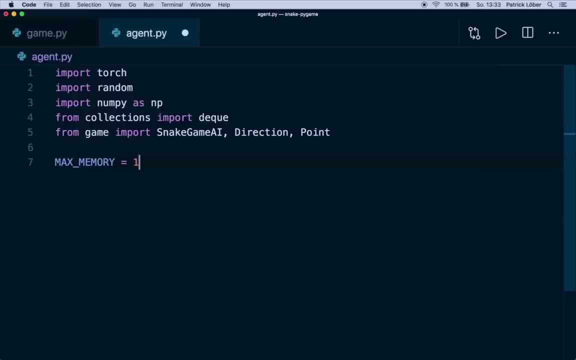 case, And then I will put a link in the description below. So this is really handy in this case, And you will see why this is the case later. And then here I want to define some parameters. then we also want to use a batch size- that you will see later- And here I will set this. 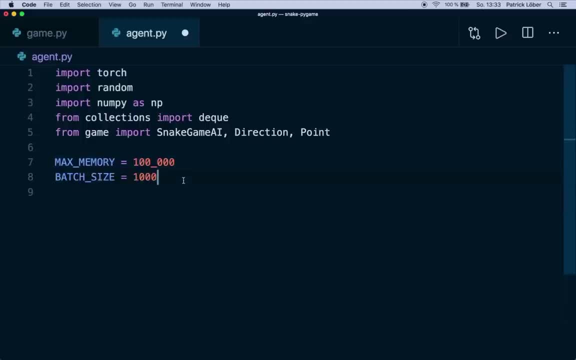 to 1000.. So you can play around with these parameters And I also want a learning rate later And I want to set this to 001.. And yeah, feel free to change this. And then we start creating our class agent And it gets, of course, an init function with self and 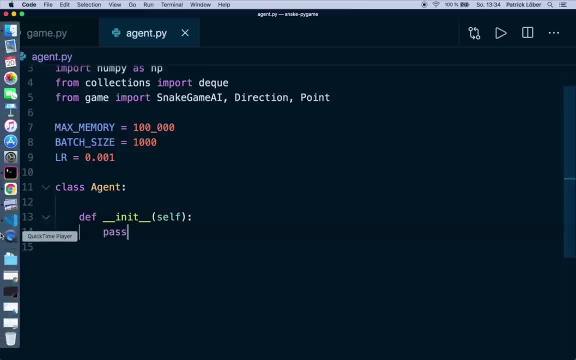 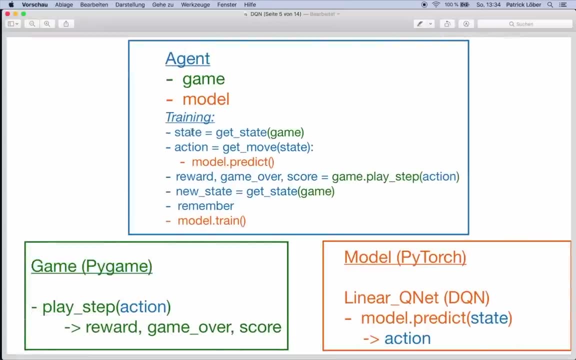 no other arguments. And then let's have a look at the slides from the first part where I explained the training. So we want to create a training function where we do all of this. so we need to get the states calculate the state where we are. 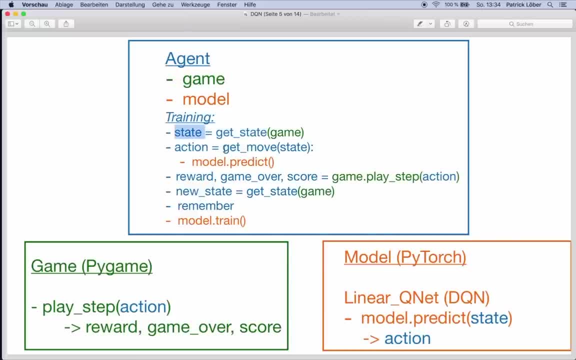 aware of the current environments, then we need to calculate the next move from the state, And we need to. then we want to update or do the next step and call game dot play step and then calculate the new state again. then we want to store everything in memory And 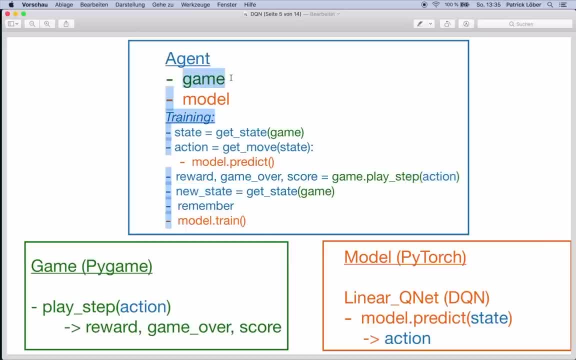 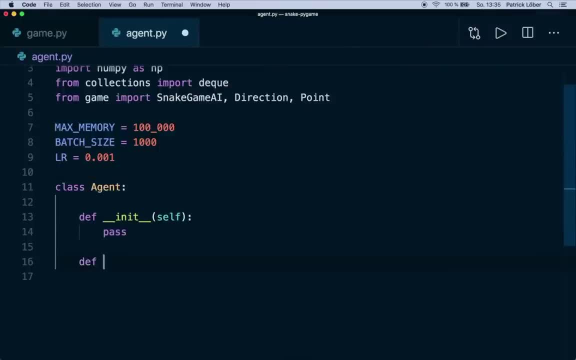 then we also want to train our model, So we need to store the game and the model in this class. So first of all, let me create the functions that we need first. So we need a function, get state, which gets self, and that's this gets the game, And then we calculate. 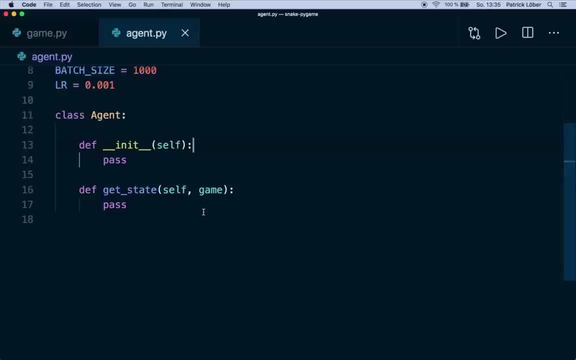 the state that I showed you with these 11 different variables. then we want to have a function that we call remember. remember, and it has self. And here we want to put in the state, then the action, then we want to remember the reward for this action, And 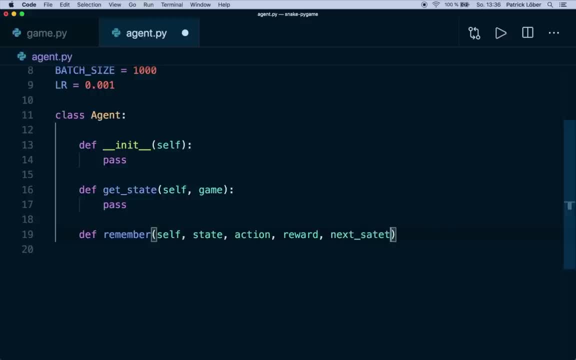 we want to calculate or we want to store the next state, next state, And we also want to store done or bait, or you can also call this game over. So this is the current game over state. then we need two different functions to train. 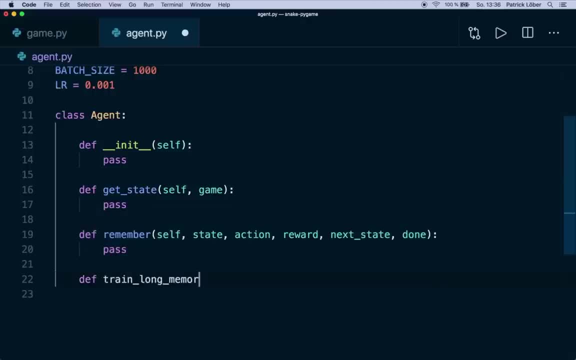 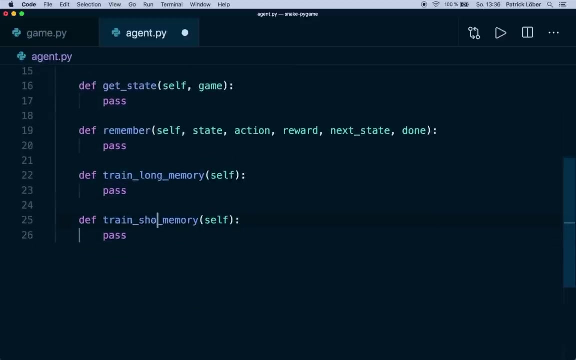 So we need a function defined train on the long memory and it only needs self. So I will explain this later And we also- let's copy and paste this- I also have a function defined train on short memory. So this is only with one step. you will see this later. 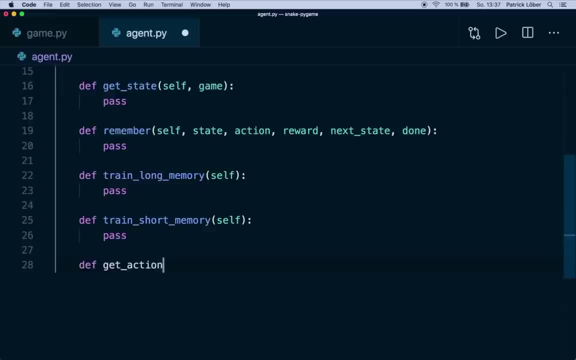 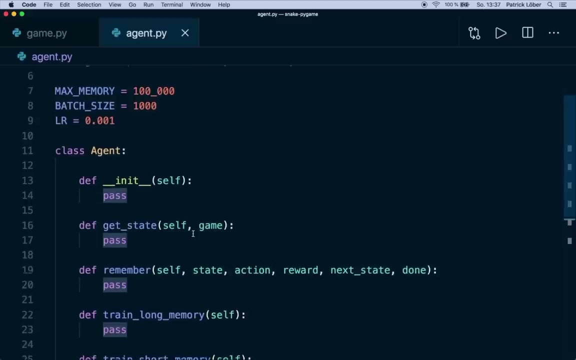 then we need a function And we call this get action, to get the action based on the state. So it gets self and the state And first we only say pass. And these are all the functions we need, I guess. And then I want to have a global function that 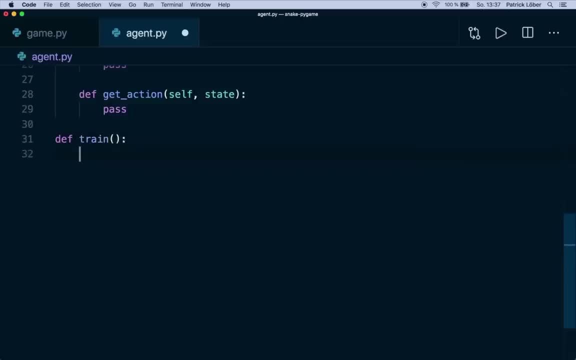 I call simply train And here we say pass, And then when we start this module, agent dot pi. so we say if name underscore equals equals main, then we simply call this train function And then we can start the script by saying Python agent dot pi, like I did in the very first tutorial. So let's start. 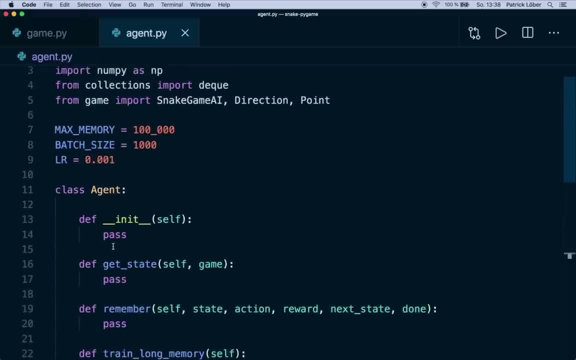 implementing the agent and the training function. So let's start with the init function of the agent. So here, what I want to store is: first I want to store some more parameters, So self dot, number of games. so I want to keep track of this. So this is zero in the beginning. 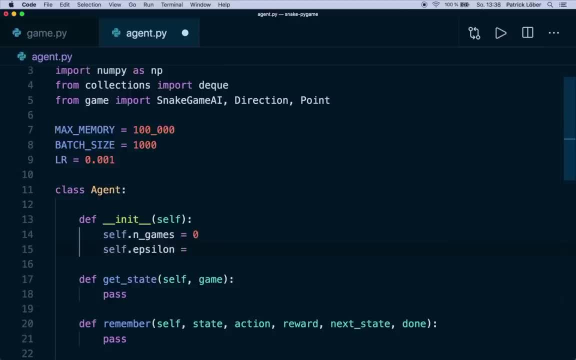 then self dot epsilon equals zero. in the beginning, this is a parameter to control the randomness, So you will see this later. then we also need self dot gamma equals zero. So this is, this is the so called this count rate, which I briefly showed in the first tutorial. I will explain this a. 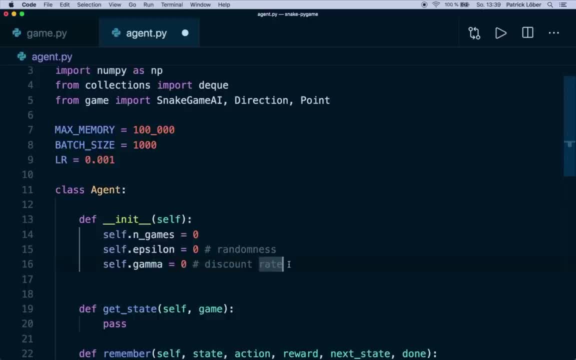 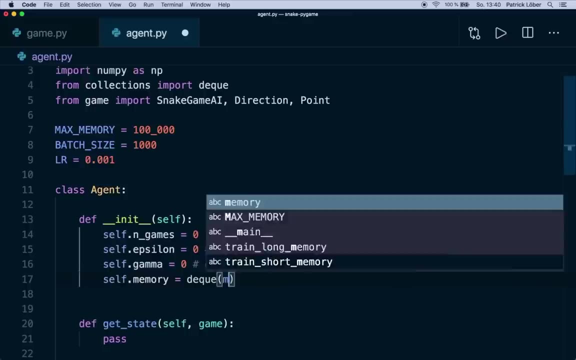 little bit more in the next tutorial where we implement the model and the actual deep Q learning algorithm. then we want to have a memory. So we say self dot memory equals, And for this we use this deck. And this can have a argument: max length equals. And here 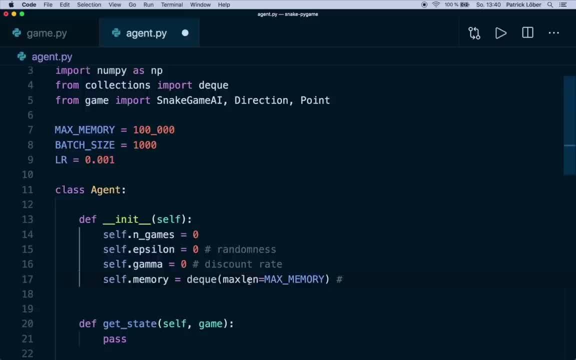 we say max memory, And what then happens? if we exceed this memory, then it will automatically remove elements from the left, so then it will call pop left for us, And that's why this deck is really handy here, And then later here we also want to have our model and the trainers, So I will 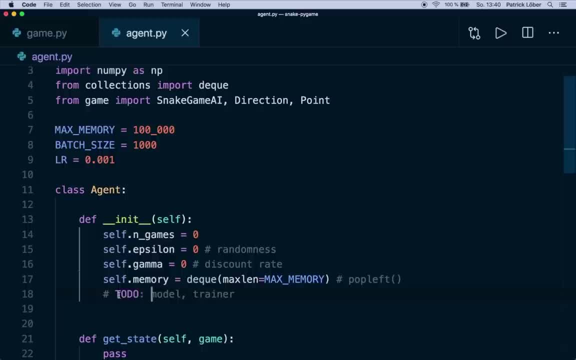 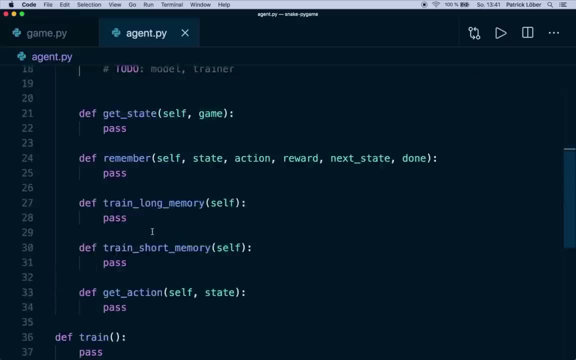 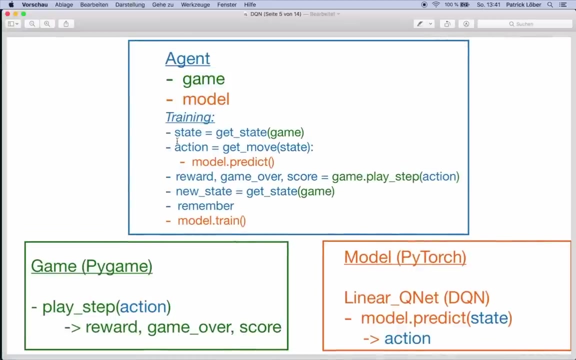 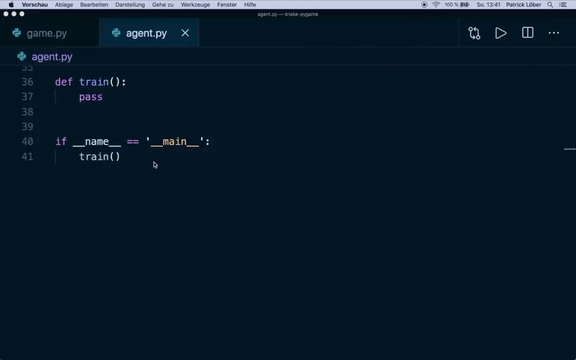 leave this for a or as to do for the last part in the next video. And now, this is all for the init function function. And now we can go back. And now let's do the training function next. So again, let's have a look at the slides. So we need these functions in this order. So let's first. 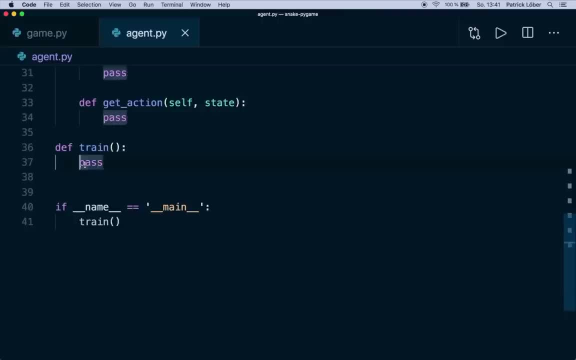 let's write some comments, Or for first, let's create some lists to keep track of the scores. So this is an empty list in the beginning and this is used for plotting later. So then we also want to keep track of the mean scores or average scores. So this is also an empty. 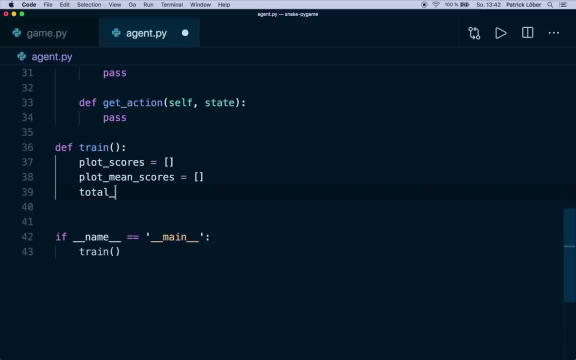 list in the beginning, then our total score equals zero in the beginning. our record, our best score is zero in the beginning. then we set up a agent, So agent equals zero And this equals an agent, And we also need to create a game, So the game is a snake game. 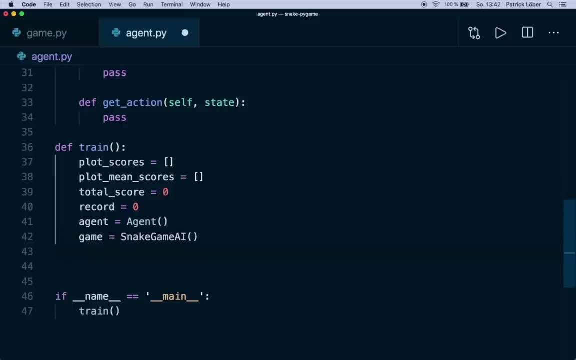 a I object. And then here we create our training loop. So we say, while true, so this should basically run forever until we quit the script. And now here let's write some comments. So we want to get get the old state. 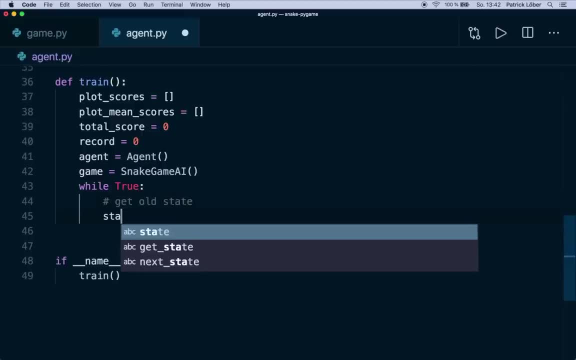 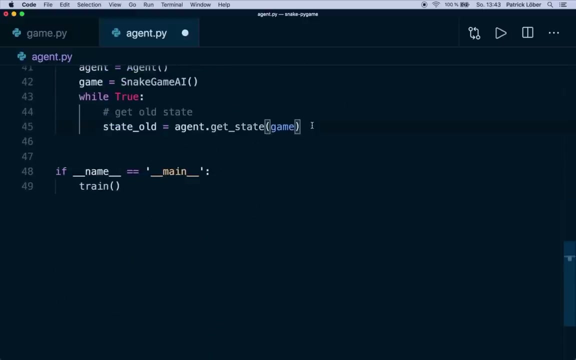 Okay, Or the current state. So here let's say state old equals, and then we call agents dot, get states And this gets the game. So we already set this up correctly, we only have to implement it then. Then, after this, we want to get the move based on this current state. So we say: 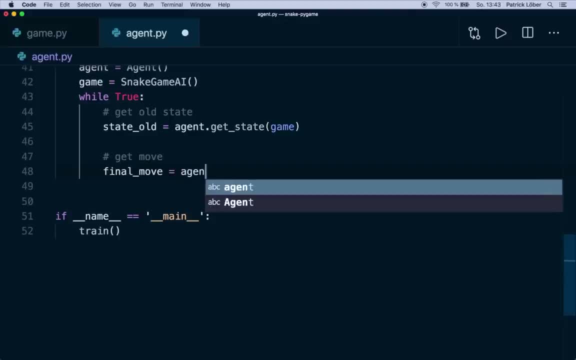 the final move equals agents dot get action. So we actually call this action And the action is based on the state. then with this move we want to perform the move and then and get new state. So for this we say rewards. 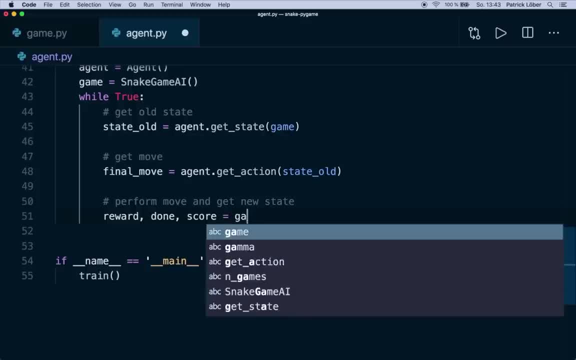 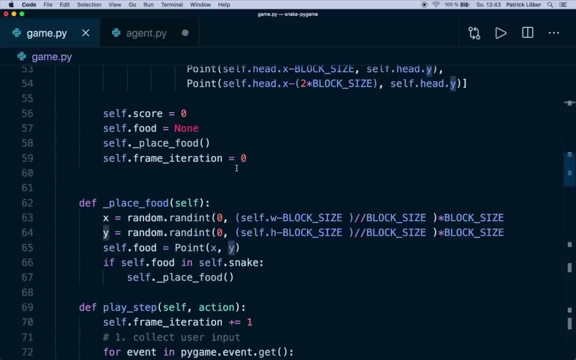 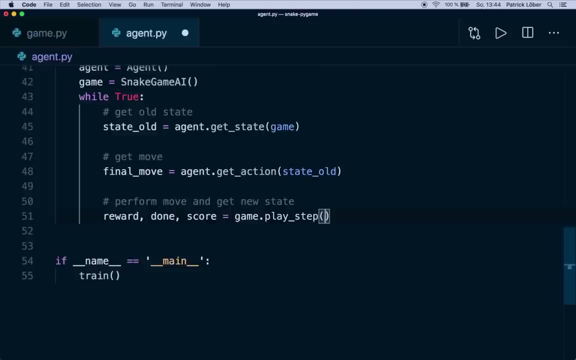 done and score equals, and here we call game dot play step from last time. So I think game dot play step with the action, Yes, game dot play step. And this gets the final move. And then we get the states- old or the new, now the new state, state, new state, new equals agent, and again get state, now with the new game. then after that we want to train the. 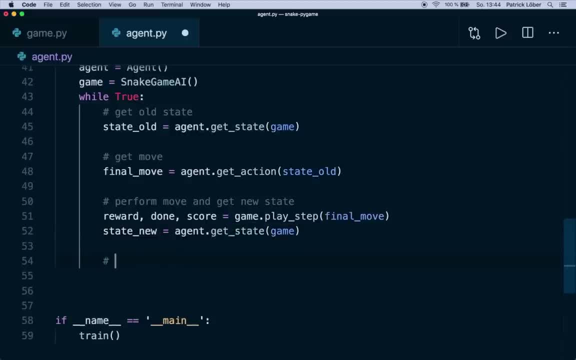 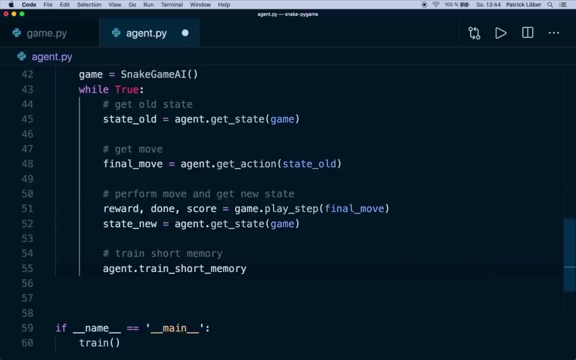 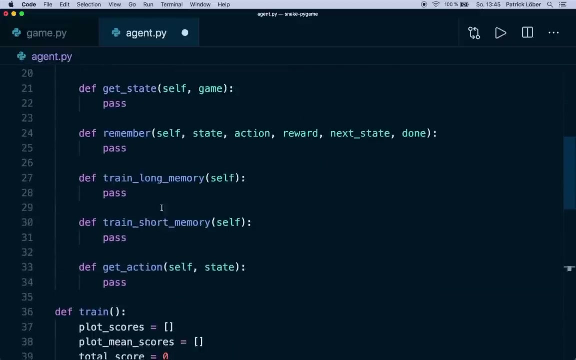 state new equals agent And again get state now with the new game. then after that we want to train the shot short memory of the agent. So only for one step. So for this we say agent, agent, dot, train short memory And this gets, if we have a look here, actually this short memory should. 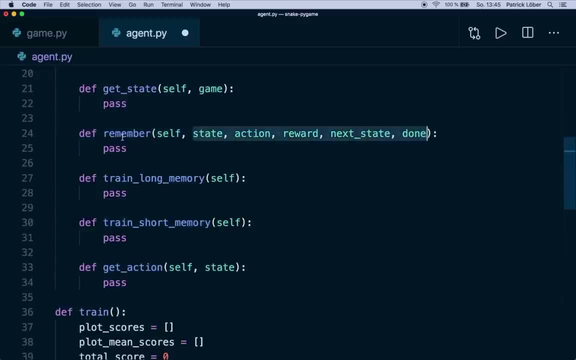 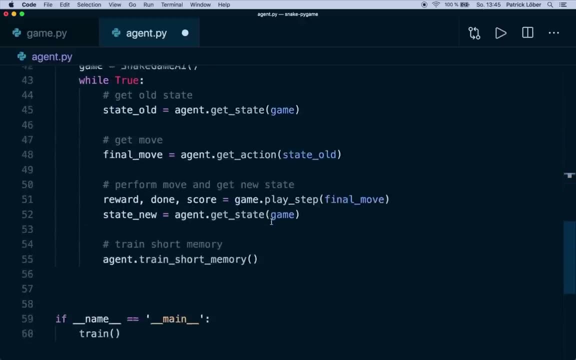 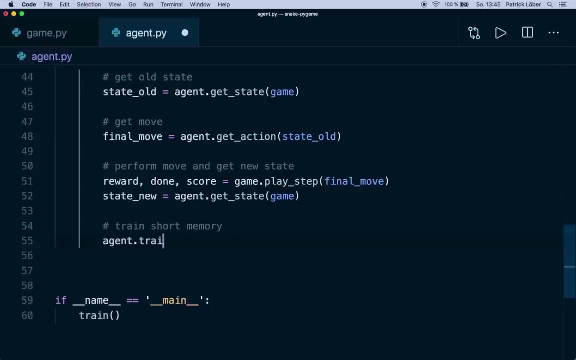 get some parameters. So exactly the same as we put in the remember function. So train short memory gets all of those variables And then here when we call this now we should get some hints: train, Or let's save this file and then say agent dot train short memory. 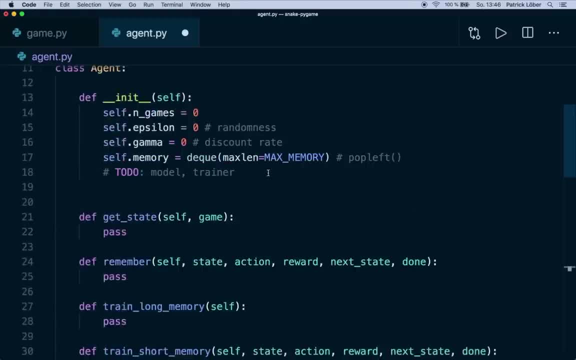 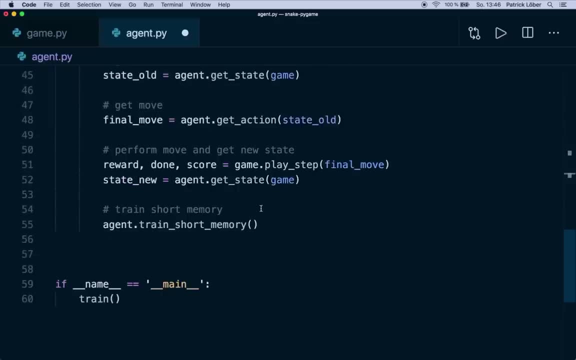 And now we should get the hints. No, we don't get this, But actually we want to have the state action, reward, next state, and done So here, let's do this, So set, let's say state old, then the action, which was the final move, then the reward. 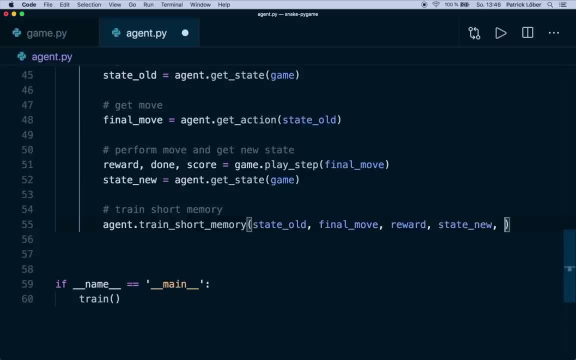 then the state new And as last thing, the done or game over state variable. So now we have this, then we want to remember all of these and store this in the memory. So we say, agent dot remember. and then here it gets the same. 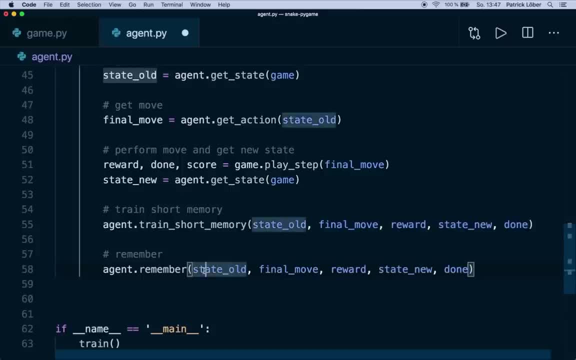 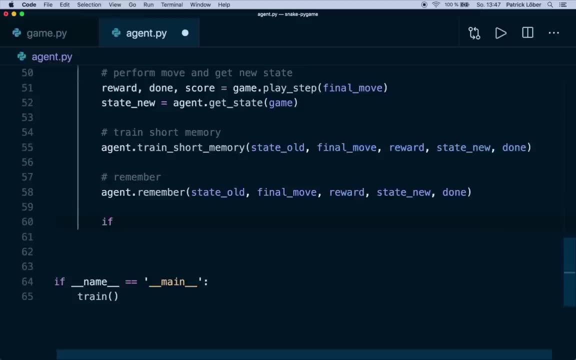 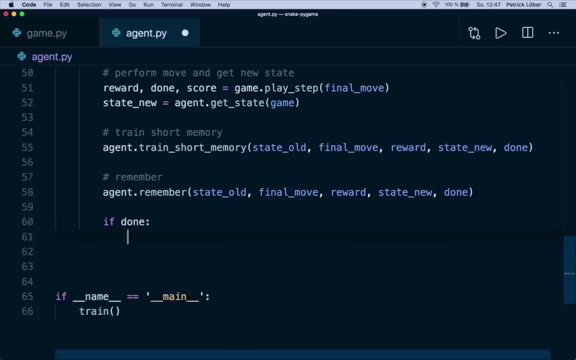 Variables. So we want to store all of this in our deck And then this is all we need. So now we check if done or if game over. then, if this is true, then what we want to do is we want to- let's write a comment- train the long memory, And this is also called replay. 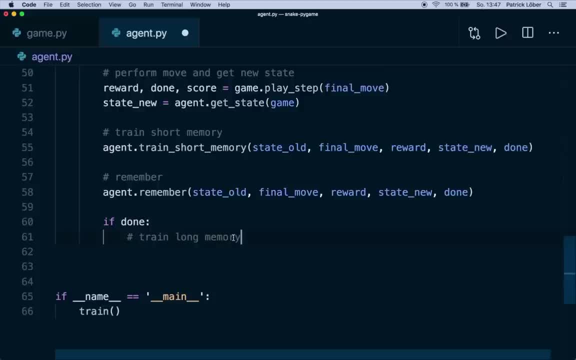 memory or experience replay, And this is very important for our agents. So now it's trains again on all the previous moves and games that it played, And this tremendously helps him to improve itself. And we also here want to plot the results. So first of all we want to reset the game. 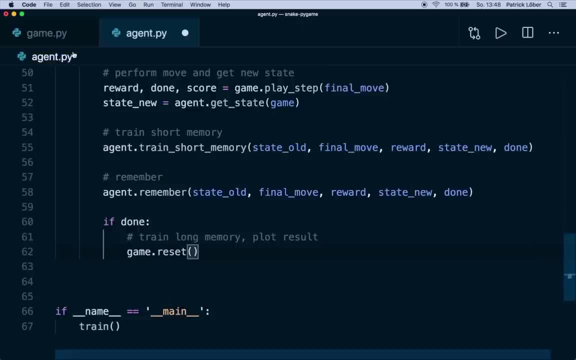 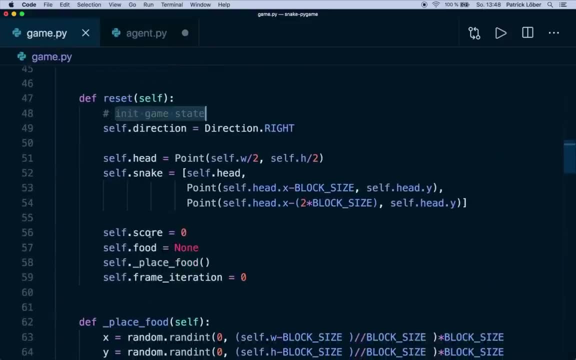 So we can simply do this by saying game dot- reset. we already have this function Here, So this initializes the game state and resets everything, So the score, the snake, the frame, iteration and places the initial snake and the food. So now we have this. then 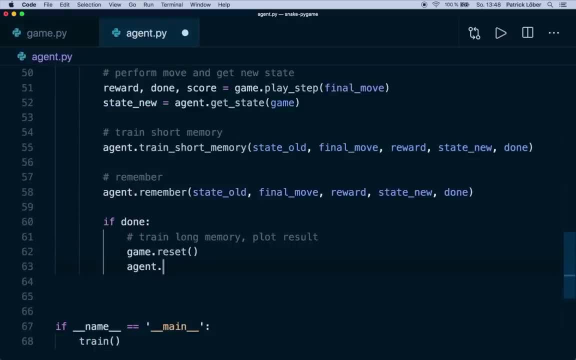 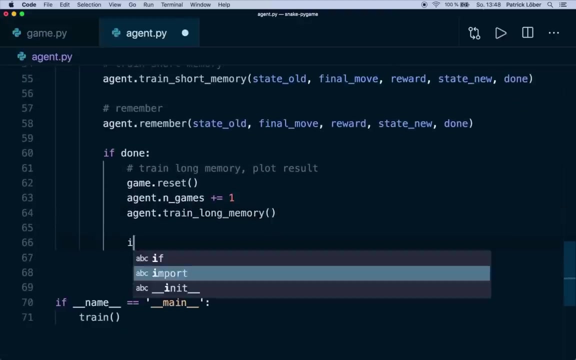 we want to increase agents dot number of games, So this plus equals one. then we want to say agents dot train long memory, And this doesn't need any arguments. then we want to check if we have a new high score. So if score greater than the current record, then we say record equals our new score. And 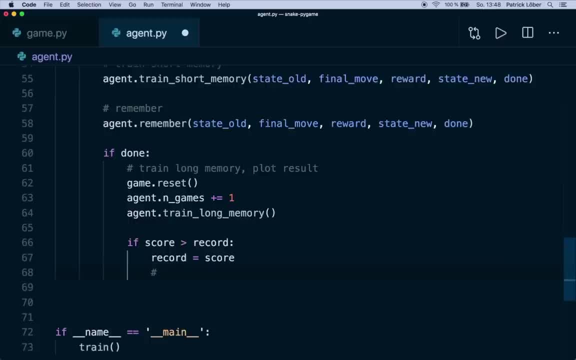 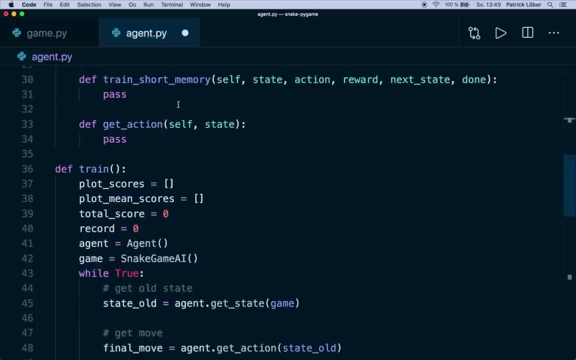 we will also want to leave this as a to do here. So here we want to say: agents dot model, dot, save later when we have the model. And so here in the here we want to store this as self dot model. And now what we also want: 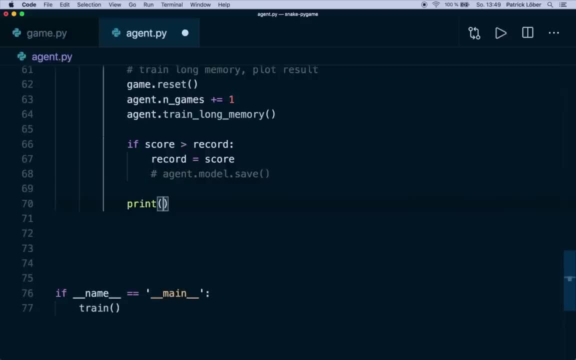 to do here? let's print some information, So print the game and then the current number and then the score and the record. So here let's say: our game is agents dot n games, then we also want to plot the or print the score. So this is just the score And we want to print the current record. So 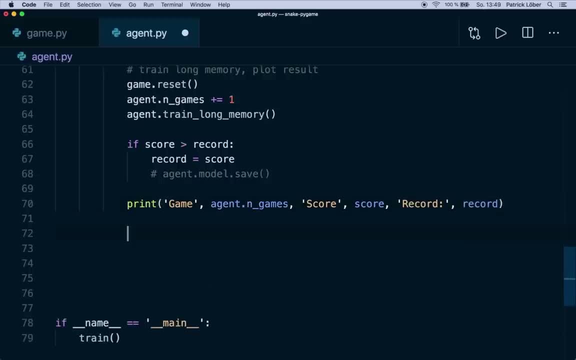 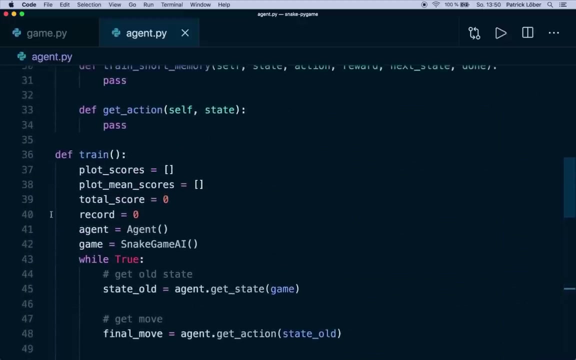 the record equals record. And then here we want to do some plotting, So I will implement this in the next tutorial, So I will leave this as a to do. So this is all for our training function. So what I showed in the slides, and now of course we have to implement those. 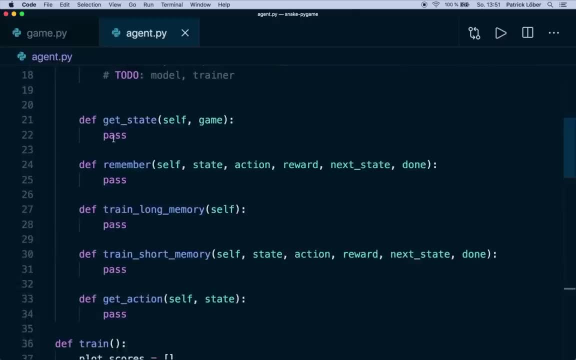 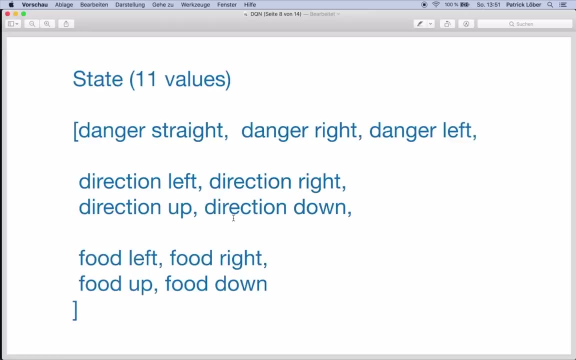 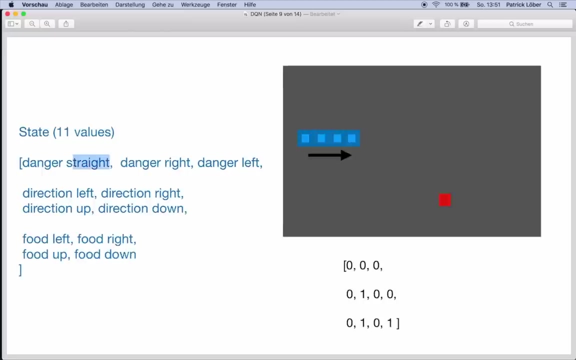 functions. So for the get state function, let's go back to this overview And here, as I said, we store 11 values. So if the danger is straight, right or left, then the current direction, so only one of these is one- And then the position of the food if it's left. 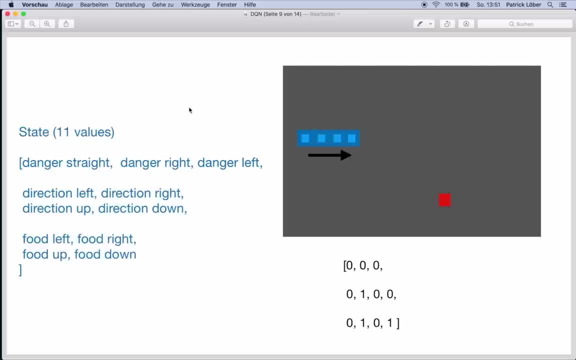 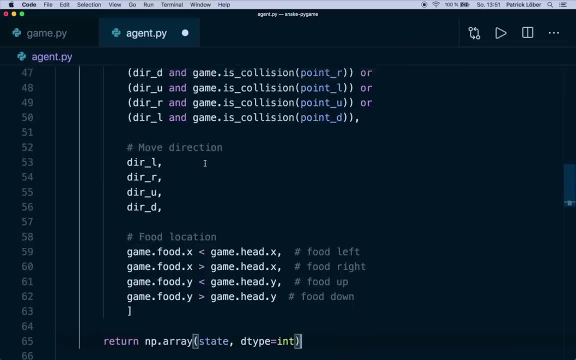 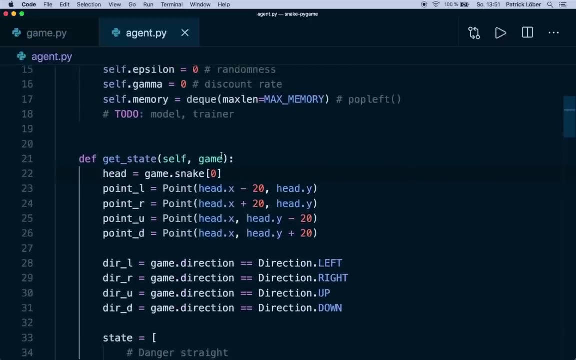 of the snake, right of the snake, up or down of the snake. So these are the 11 states. And now let me actually copy and paste the code in here so that I don't make any mistakes. But we will go over this. So first let's grab the head from this: 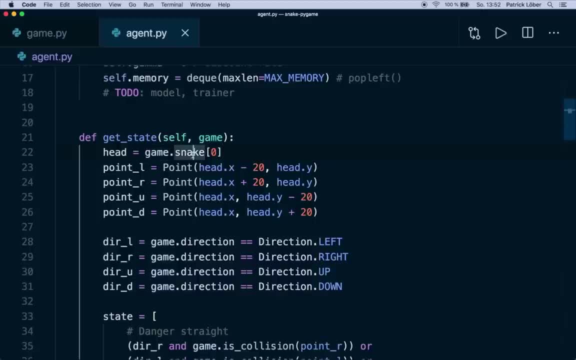 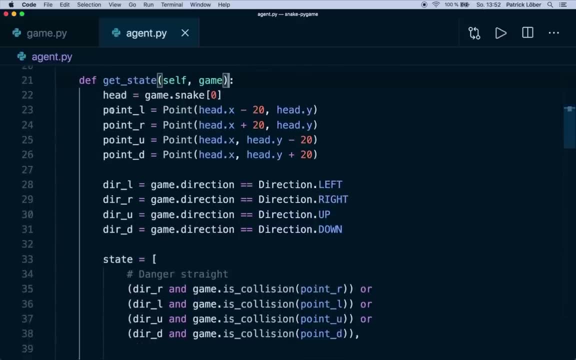 game. So we can do this by calling game dot, snake zero. So this is a list And the first item is our hat. Then let's create some points next to this hat in all directions that we need to check if this hits the boundary and if this is a danger. So for this we can use 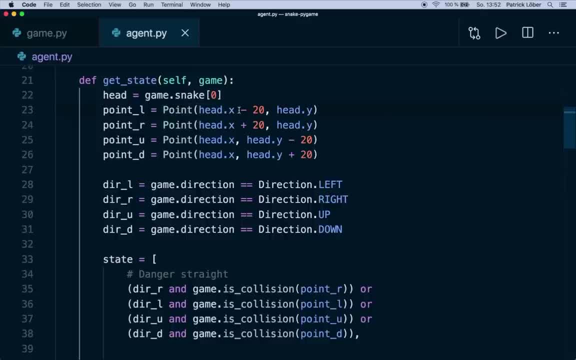 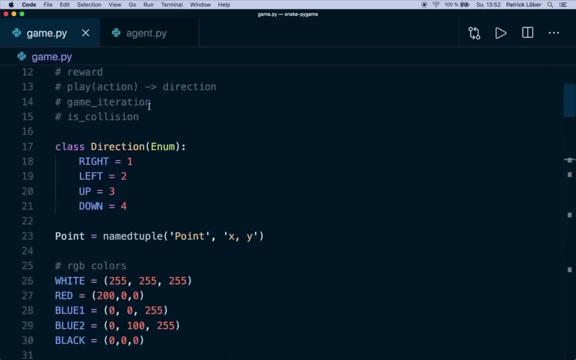 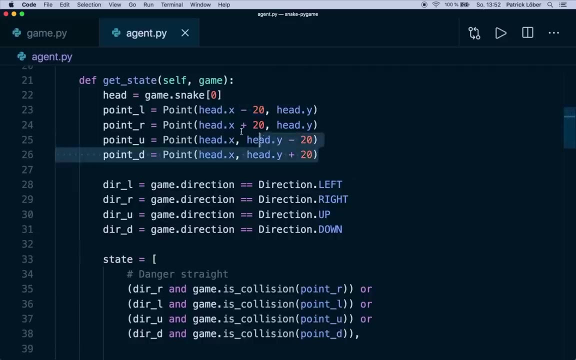 this named tuple, So we can create a point with this location, But minus 20. So the 20 is hard coded here. So this is the number that I used for the block size. So like this we create four points around the head, then the current direction. 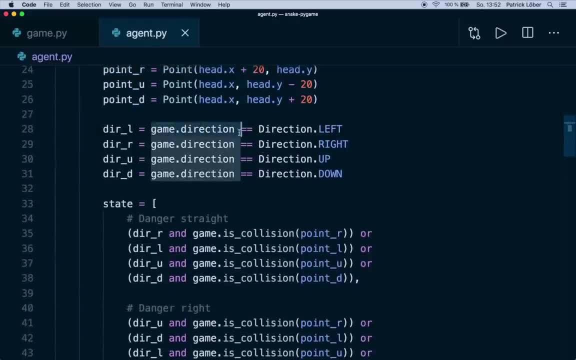 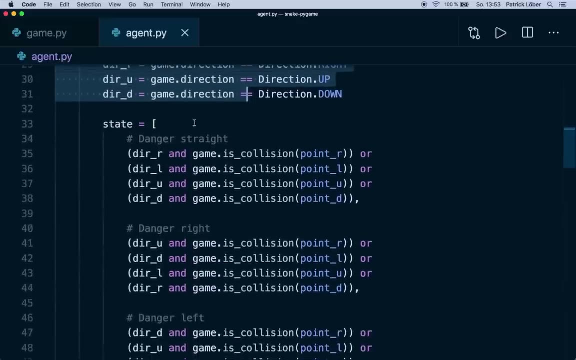 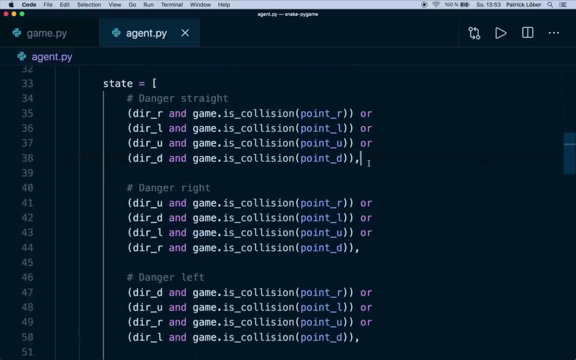 is simply a Boolean where we check if the current game direction equals to one of those. So only one of those is one and the other one is two- Zero or false, And then we create this array, or this list, with this 11 states. So here: 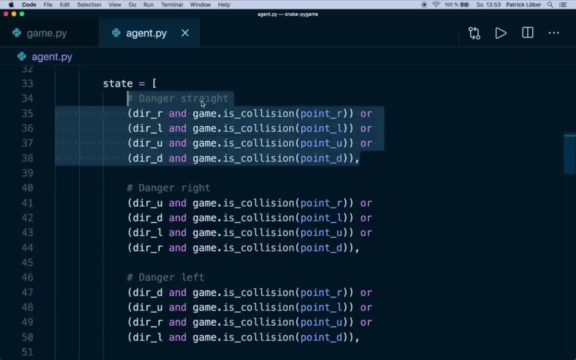 we check that if the danger is straight or a hat, and this is dependent on the current directions. So if we are going right and the point right of us gives us a collision, then we have a danger the same. or or if we go left and our left point gets a collision. 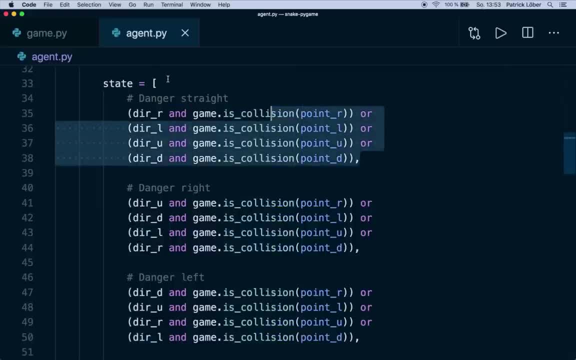 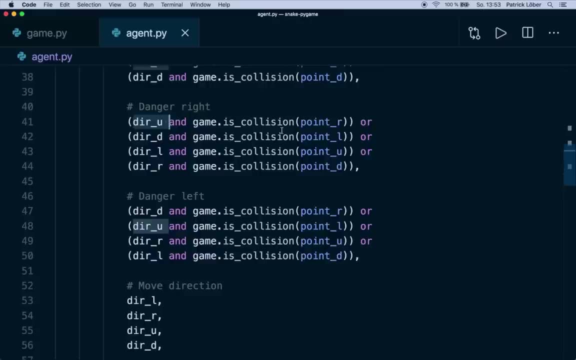 then we also have a danger here, and so on. So this is dangerous straight. And then danger right means if we go up and the point right of us would give a collision, then we have a danger for a right turn, basically, And so on. 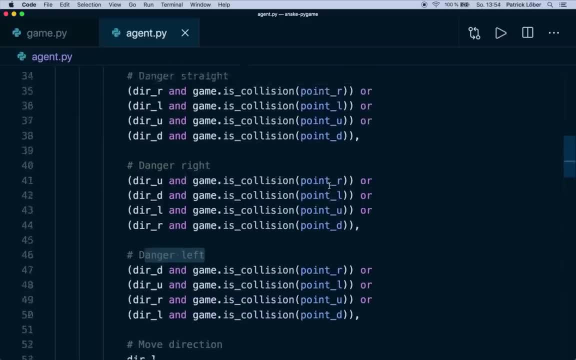 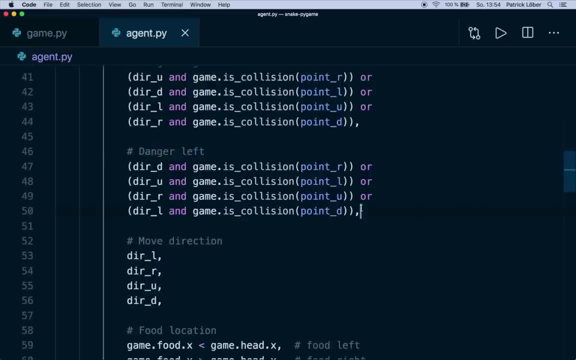 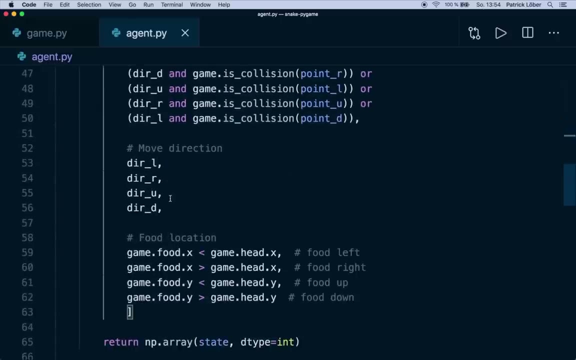 and the same for the left. So this might be a little bit tricky, So I recommend that you pause here and go over this logic for yourself again. So yeah, these only have give us three values in our state so far. then we have the move direction, where only one of them is true. 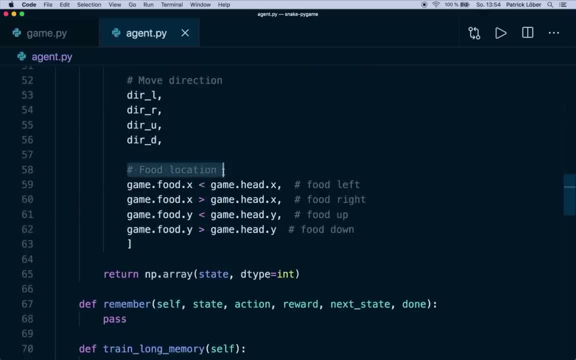 and the other one is false. And for the food location we simply check if food, if game food x is smaller than game head x, then we have food is left of us. And the same way we check for right up and down. And then we convert our list to a numpy array and say the data type is in. So 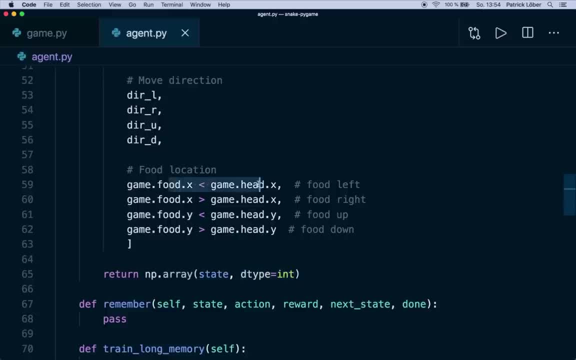 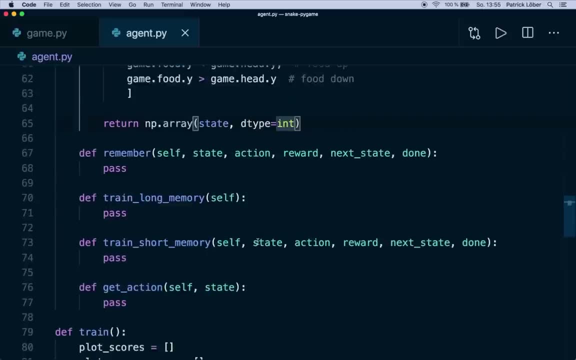 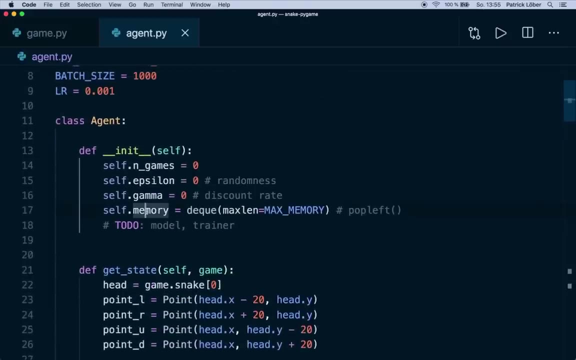 this is a nice little trick to convert this true or false Buelian to a zero or one. So yeah, now this is the get state method. Now let's move on to the remember function. So here we want to remember all of this in our 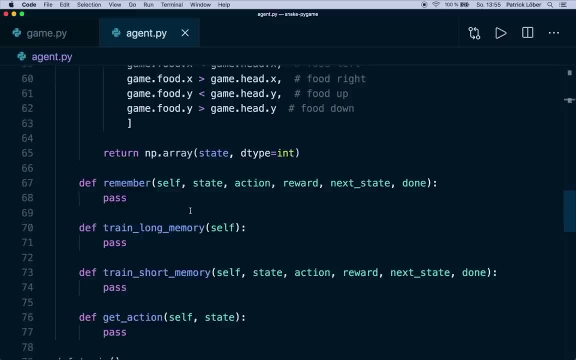 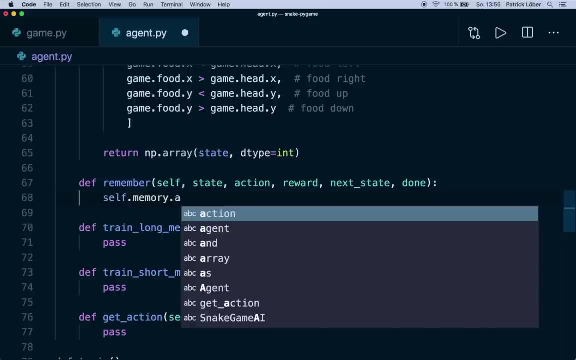 memory. So this is a deck And this is very simple. So here we say self dot memory and then the deck has also the append function where we want to append all these things right here. So we convert this as state And then this adds itself to the memory effort. 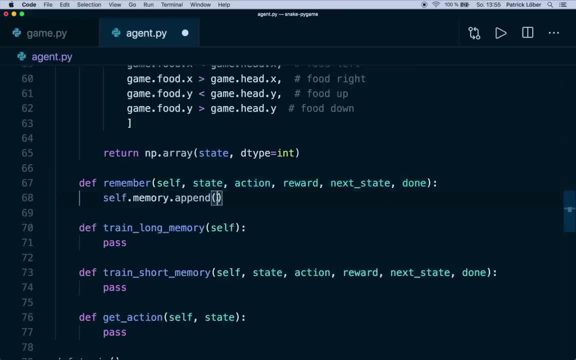 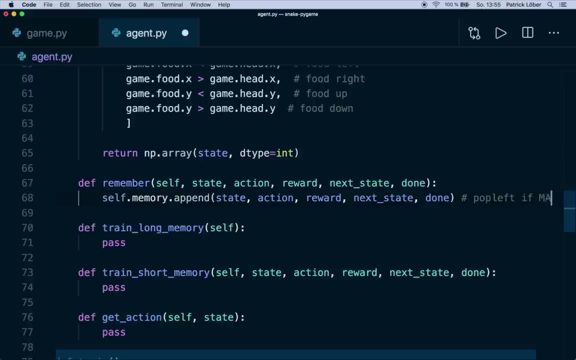 purpass and this is what we want. excellent as we go. Yeah, Of course, like I said, I can all of this in this order. So the state, the action, the reward, the next state and the game over state. And, as I said, if this exceeds the maximum memory, then pop left if max mem. 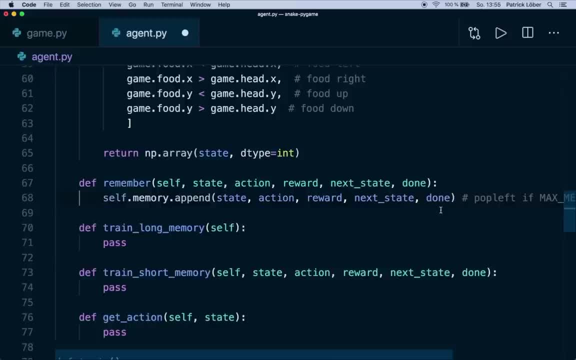 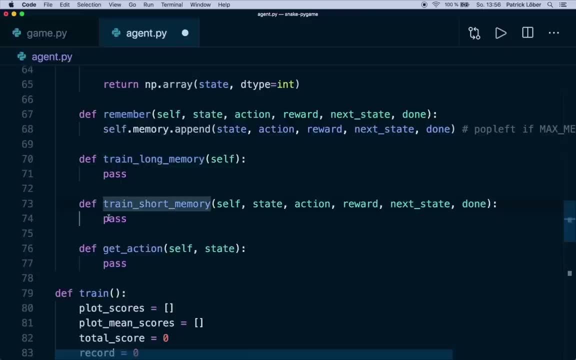 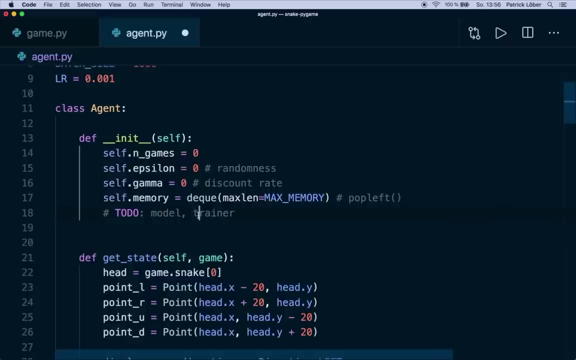 memory is reached, And yeah, this is the remember function, then let's start implementing the train long and short memory functions. So for this, so we actually we store a model and a trainer in here. So let's actually say self dot, model equals. let's say this is only 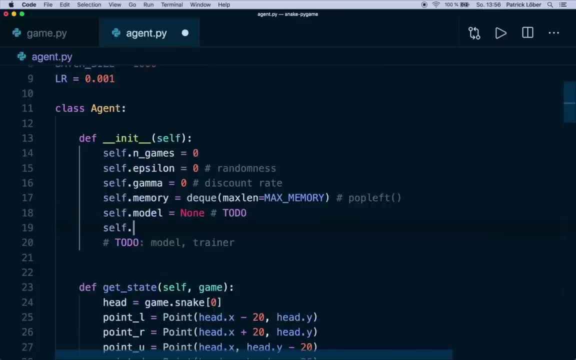 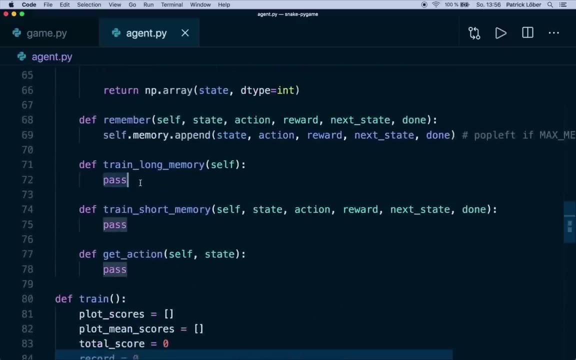 none in the beginning and leave a to do. and self dot trainer equals none in the beginning And this is a to do. So these are objects that we create in the next tutorial, And then here we call this trainer to actually do the optimization. So 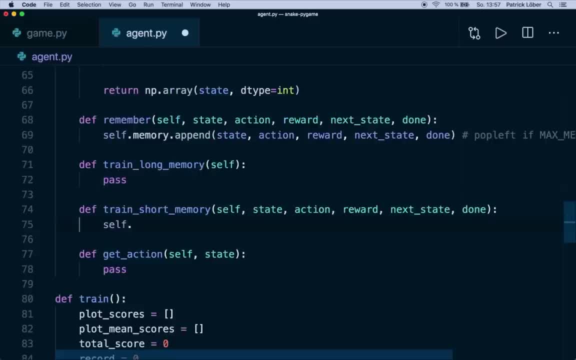 let's start here. So for only one step we say self dot trainer, and then this should get a function that we call. let's call this train step, And then it gets all of these variables. So the state, the action, the reward, the next state and the game over state. And 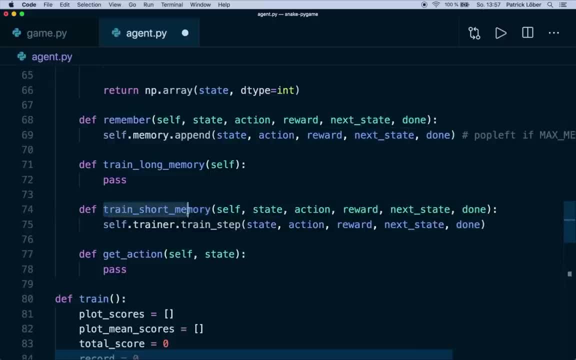 this is all that. we need to train it for only one game step, And we design this function So that it takes either only one state like this, But it can also take a whole tensor or a numpy array and then uses multiple as a so called batch. So let's do this. 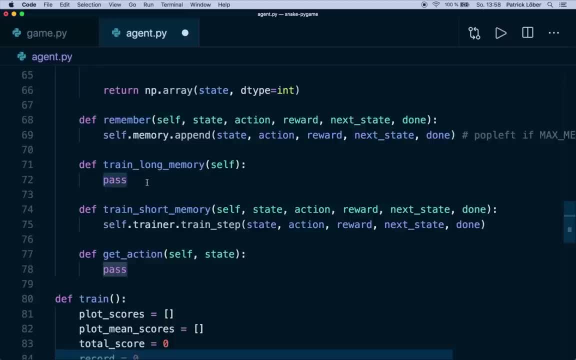 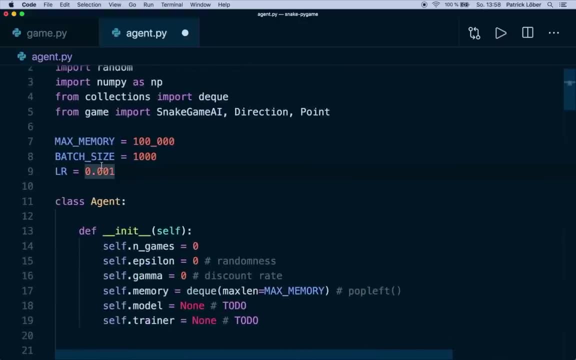 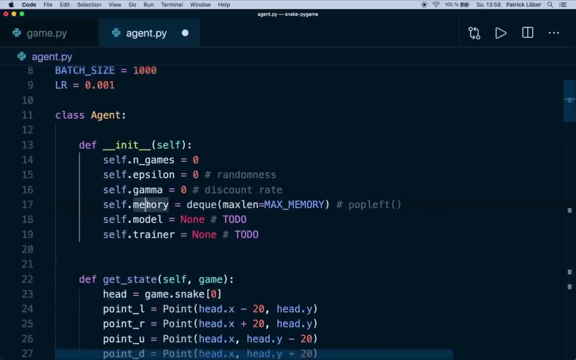 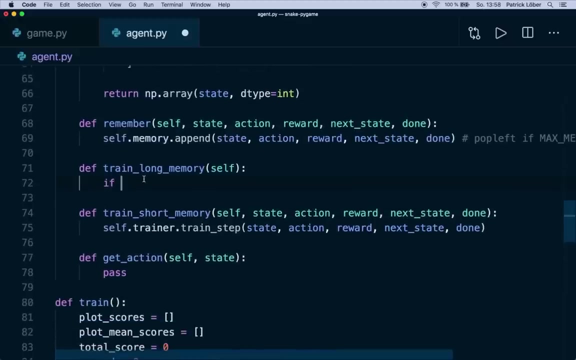 Here. So for this we take the variables from our memory. So here we want to grab a batch, And so in the beginning we defined the batch size is 1000.. So we want to grab 1000 samples from our memory. But first we check if we already have 1000 samples in our 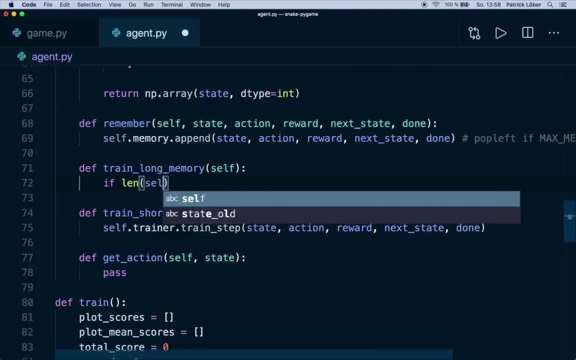 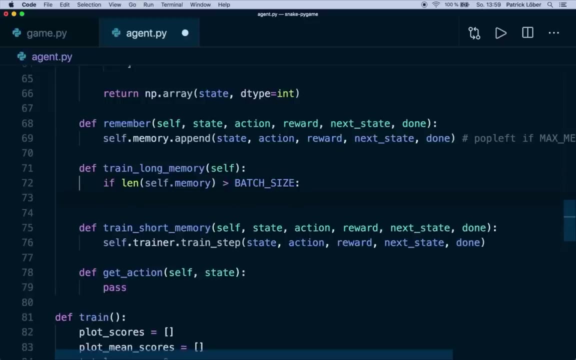 memory. So we say if lang and self dot memory, if this is smaller than the batch size, then we simply, or actually let's say if this is greater. so if this is greater, then we want to have a random sample and say mini sample. 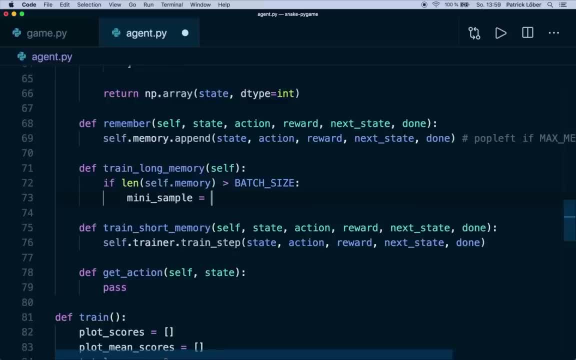 equals. and then we want to get a random sample So we can use random dot sample. So we already imported the random dot sample from self dot memory And as a size it should have the batch size. So this will return a list of tuples. And this is because here I forgot one important thing. 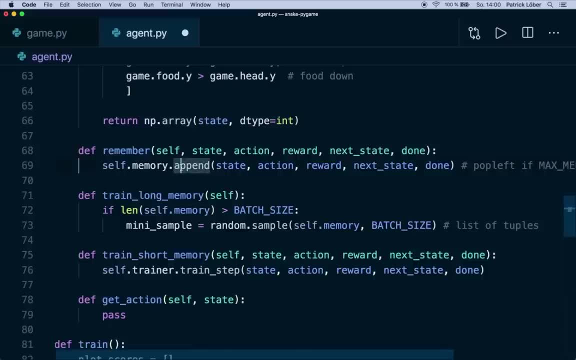 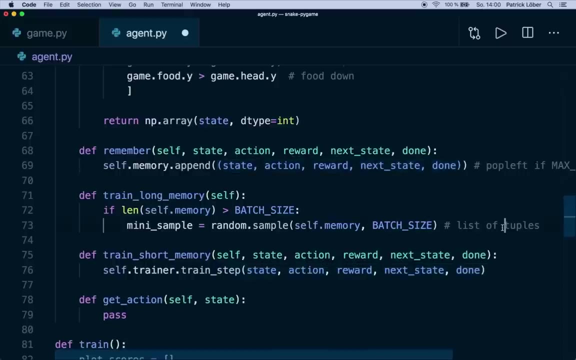 So when we want to store this and append this, we want to append this as only one element, So only one tuple. So we need extra parentheses here. So this is one tuple that we store, And then here we get the batch size, number of tuples And otherwise else. if we don't have 1000 elements yet, then 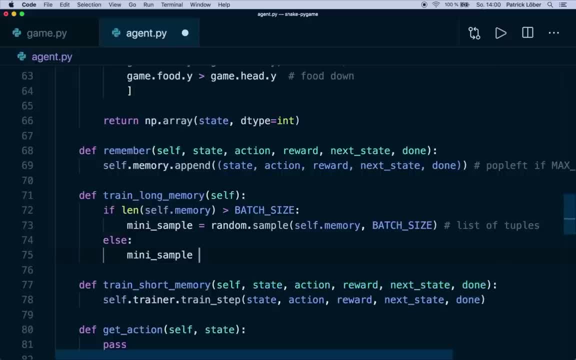 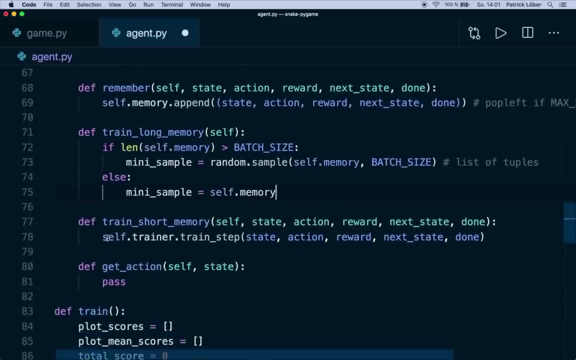 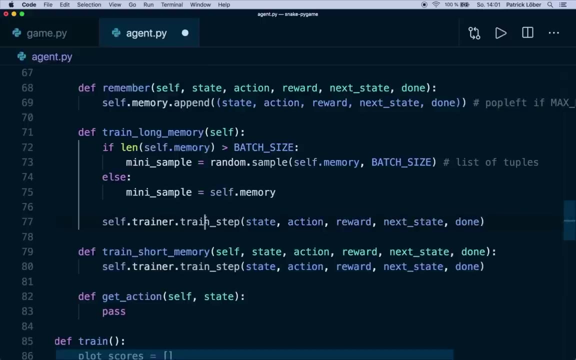 we simply take the whole memory, So we say mini sample equals self dot memory. And then we again want to call this training step. And for this, so let's call this here again, self dot trainer, dot train step. But here we have multiple states, So let's call this: 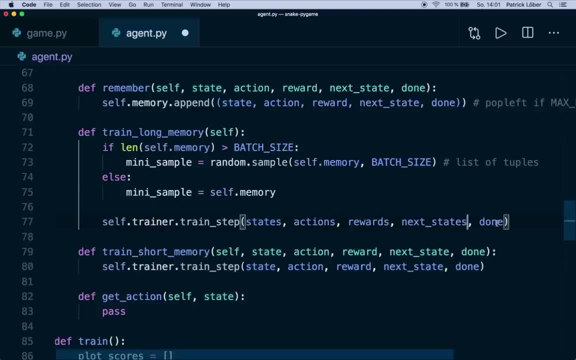 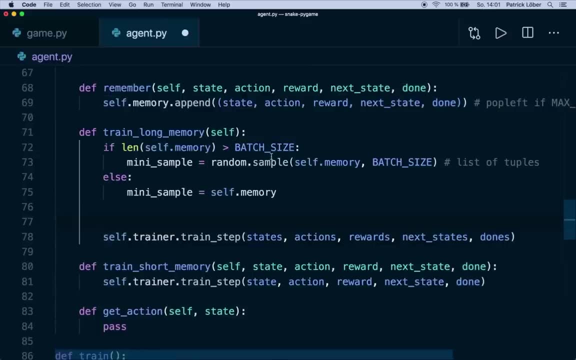 states, actions, rewards. next states and done, And right now. so now we have it in this format, that we have one tuple after another, And now we want to extract this from the mini sample and then put every states together, every action together, every reward to together. 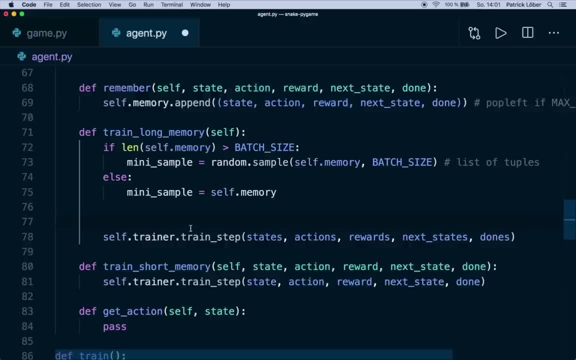 and so on, And this is actually a really simple with Python. So we can say: we want to extract the states, the actions, the rewards, the next state, So let's call this here. and then we can call this here And right now. so let's call this: 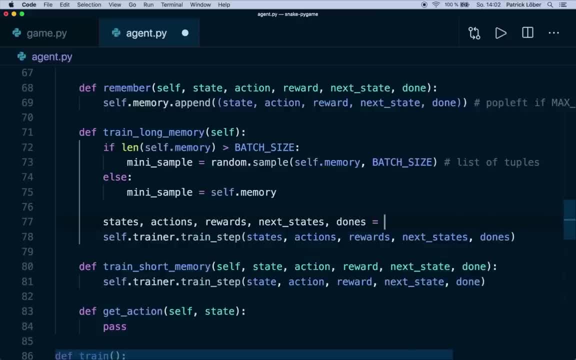 states and the dance game overs. And here we simply use the built in zip function and have to use one asterisk and then the mini sample argument. So yeah, check that for yourself if you don't know how the zip function works. But again it now it puts every states together. 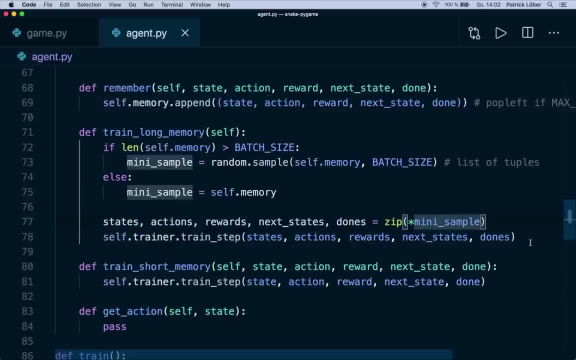 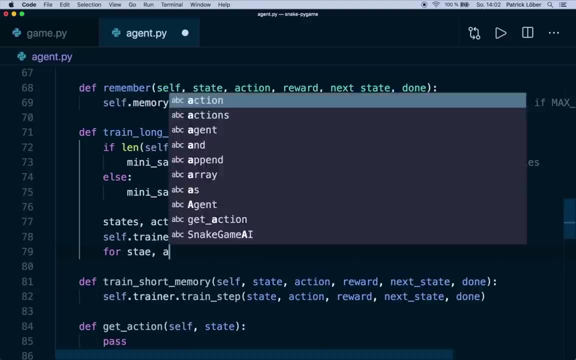 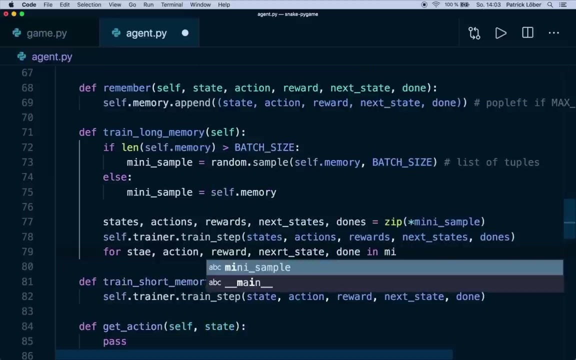 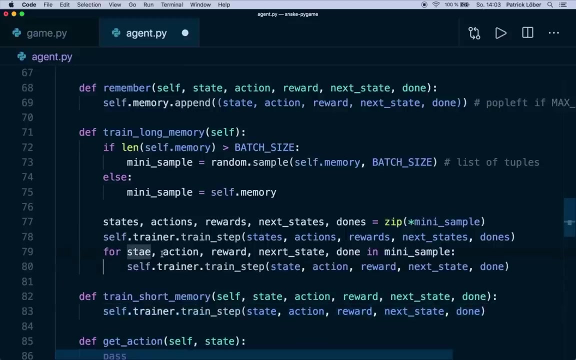 every actions and so on. If this is too complicated for you, then you can also just do a for loop, So you can iterate over this mini sample and basically say: for action or for states, action rewards, next states, and done in one mini sample, And then again you call this year for only one, for only one argument. 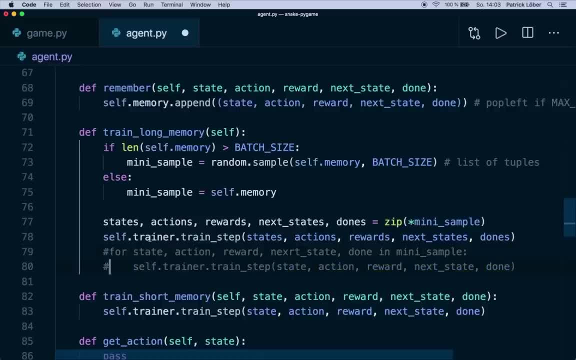 then you just want to do one argument in order to get the actual result. So if you already have the segment and you already know what you want to call it, you can just create your argument for the single segment for each state. So this is a really simple. 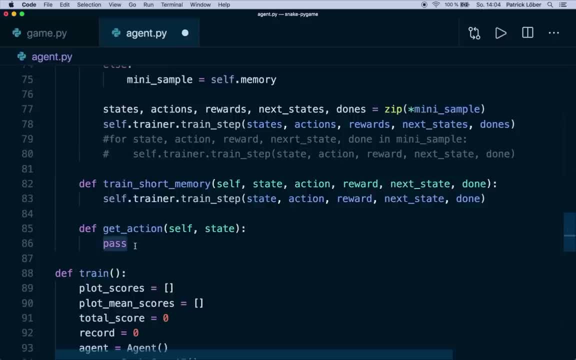 way to do it And it has a lot of criteria, as you can see here. for example, you can call this for every states and for each state, and then you can change the scale And then and exploitation in deep learning. So, at some point or in the beginning, one we want to make, 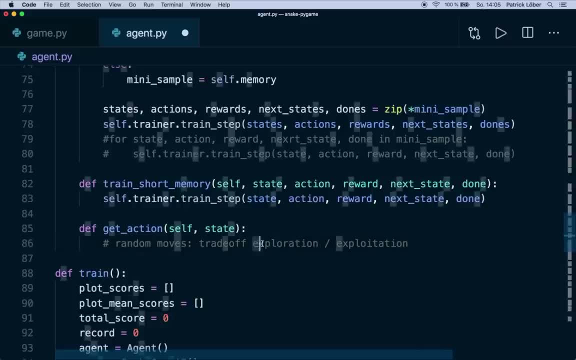 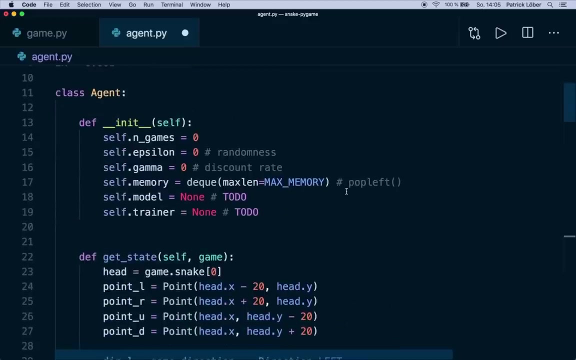 sure that we also make random moves and explore the environment, But then the better our model or our agent gets, the less random moves we want to have And the more we want to exploit our agent or our model. So, yeah, this is what we want to do here. So for this we use this epsilon parameter. 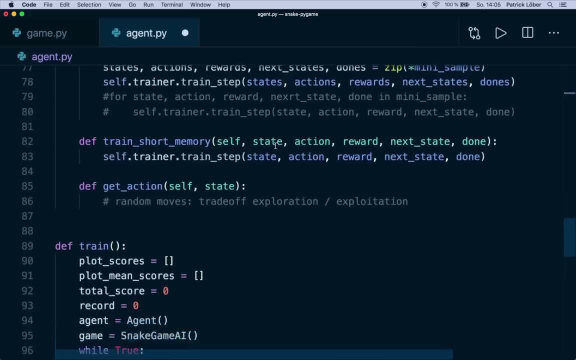 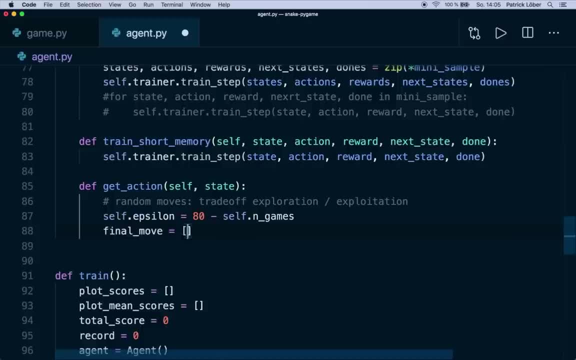 Let's get the final move. So in the beginning we say 000, and then one of those now has to be true. So here first let's check if random dot rent int, and here between zero and 200.. If this is smaller, 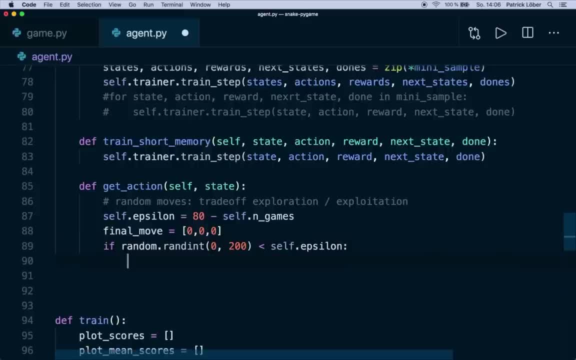 than self dots epsilon, then if this is less than self dot epsilon, then self dot epsilon equals. then we take a random move. So we say: move equals random dot rent int. And this must be between zero and two, So the two is actually included here And this will give us a random 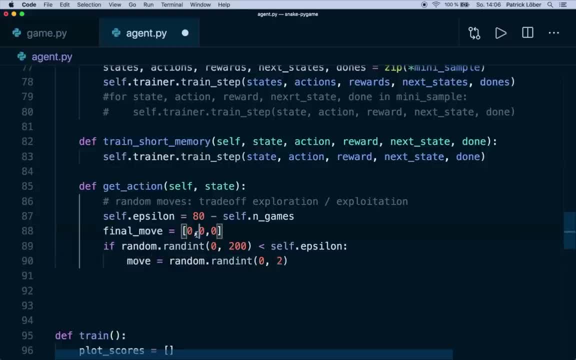 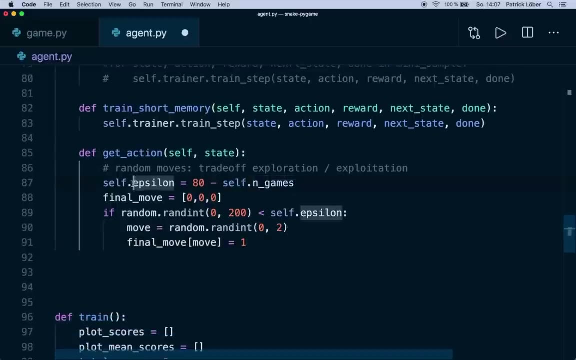 value 01 or two. And now this index must be set to one. So we say: final move of this move index equals one. And yeah so. so the more games we have, the smaller our epsilon will get. And the smaller the epsilon will get, the less frequent this will be less than the. 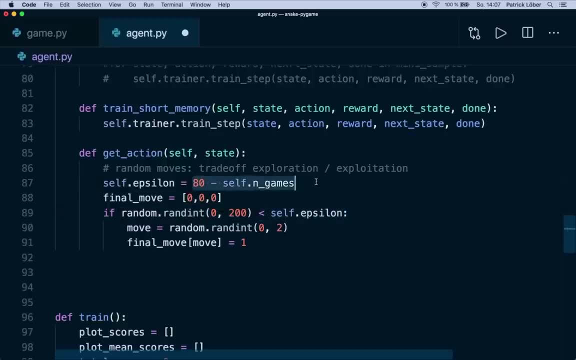 epsilon, And when this is even, this can even become negative, and then we don't longer have a random move. So again, if this was too fast here, then feel free to pause and think about this logic again. So now we have that and otherwise else. So here we actually. 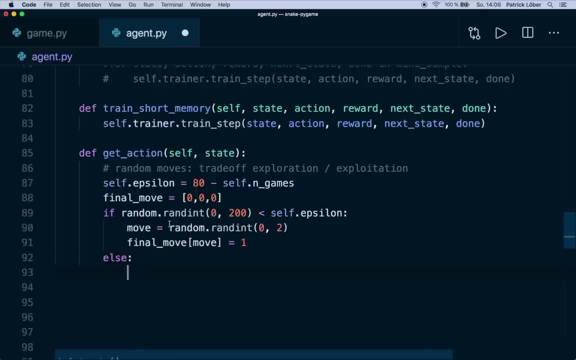 here we want to do a move that is based on our model, So we want to get a prediction- prediction equals self dot model, dot predict. And it wants to predict the action based on one state. So we call the state zero And we get this here. but we want to convert this to a tensor, So we say state zero equals. 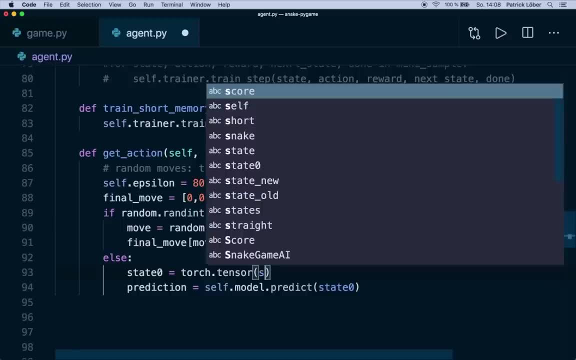 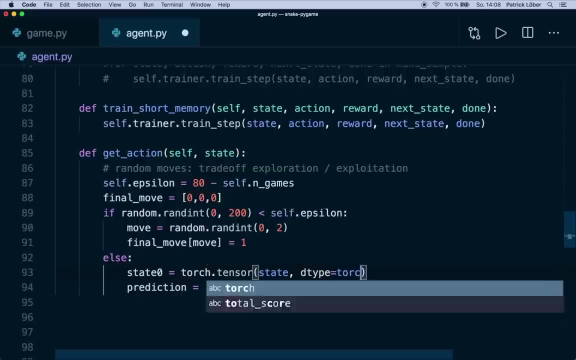 torch dot tensor And as an input it gets the state And we also give it a data type equals. let's use a torch dot float here. then we call self dot model, predict with the state. this will give us a prediction And this can be. 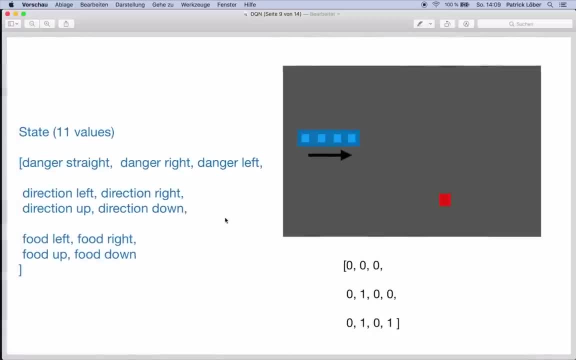 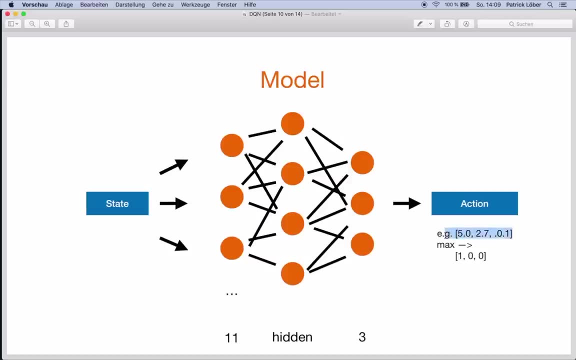 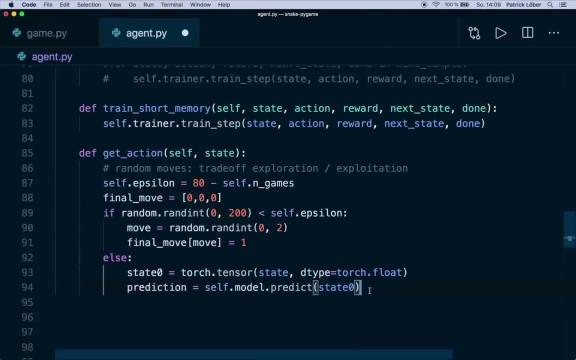 a raw value. So if we go back to this slide, so this can be a raw value, And then we take the maximum of this and set this index to a one. So here we say our move equals. and we get this by saying torch arc max and the arc max of the prediction, And this is a 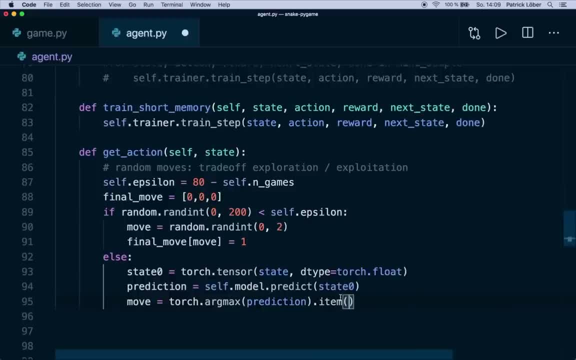 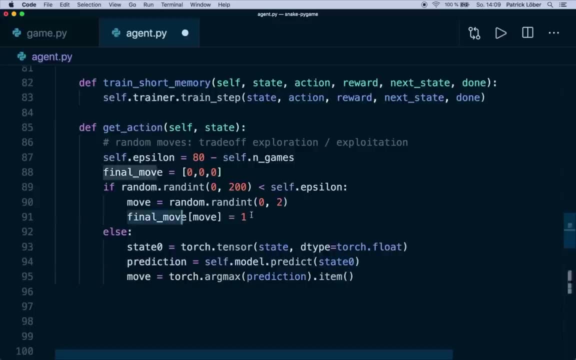 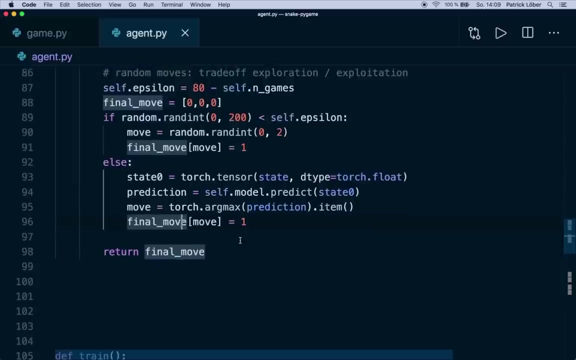 10s or again, and to convert this to only one number, we can call the item, And now this is an integer. And now again we can say: final move of this smooth index is one, And now we have this. So now we return the final move, your return, And yeah, this is all we need. So now we have this and can save it like this, And now we can save this, and now we can save it, And now we can save this And we get. this is what we have here. that's nice. So we might have an interconnection. okay And yeah, if, eventually, if you can update the conservative. 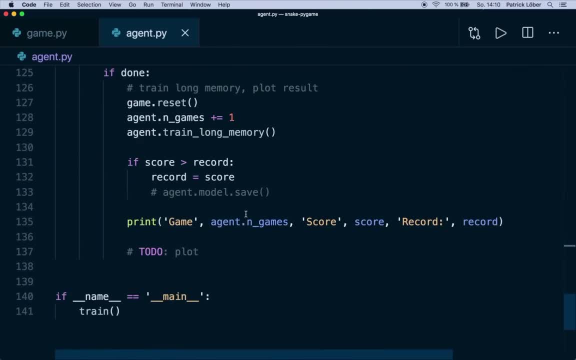 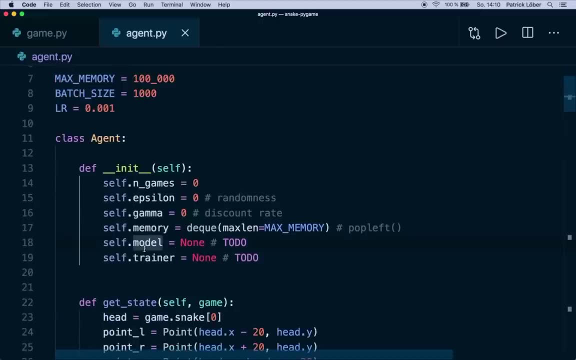 or that's going to work, then we can says: hey, great, Okay, this is it. so now we have a canceled And now we have all that we need for our agent class, And now in the next one. so what we must do here is implement the model and the trainer and then also the plotting. 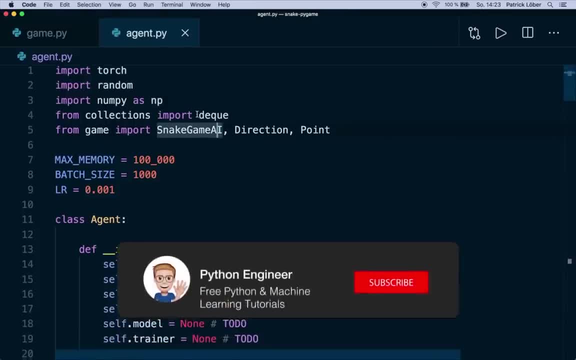 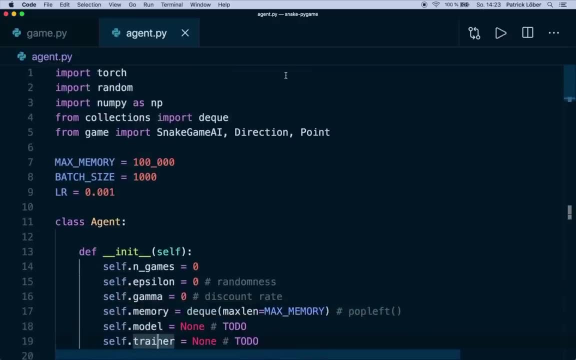 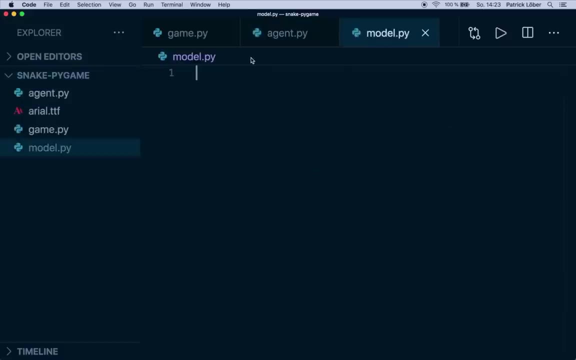 So let's go back to the code, And here I left this as a. to do so, we need a model and a trainer. So let's create a new file And let's call this model dot pi. And then here let's first import. 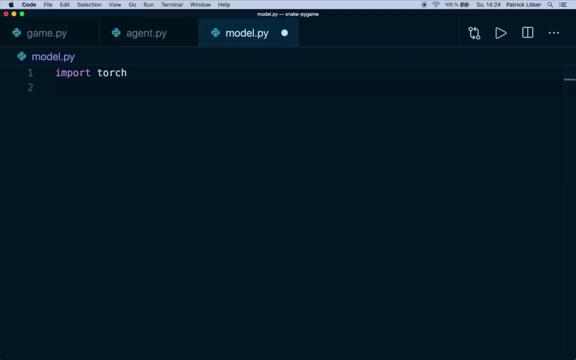 all the things we need. So we need import torch, then we want to import torch dot n n s n n, then we want to import torch dot optim s optim, and also import torch dot n n dot functional as capital F, And we also want to import OS to save our model. 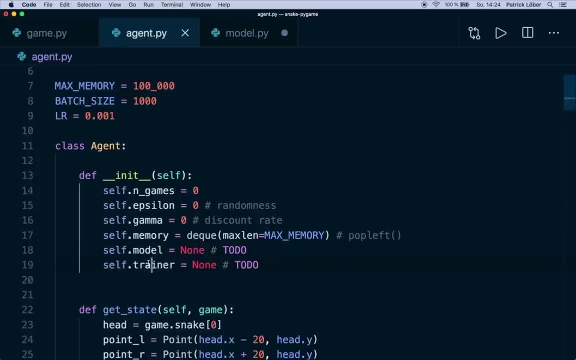 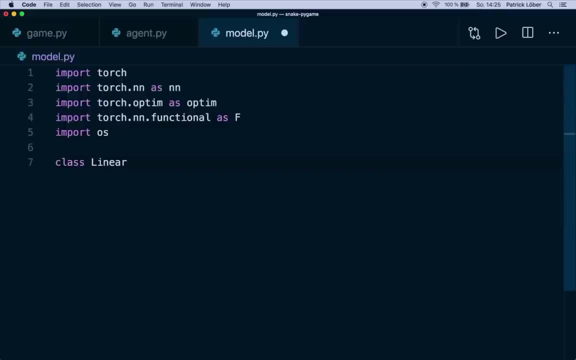 And now we want to implement two classes, one for the model and one for the trainer. So let's create a class And let's call this linear underscore q, net, And this has to inherit from n, n, dot, module, module. And, by the way, if you are not comfortable with pytorch and want to learn, 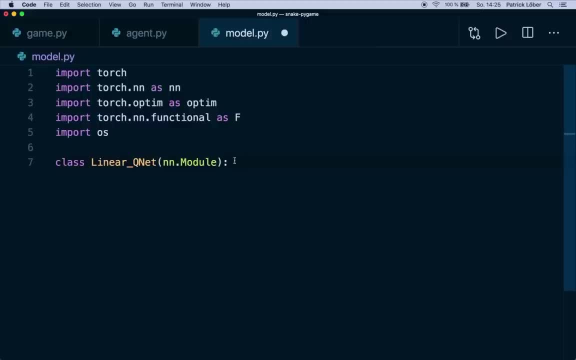 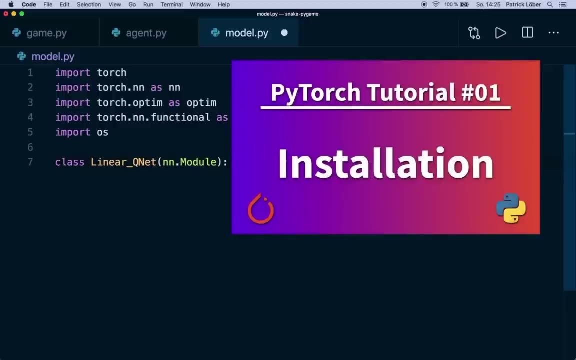 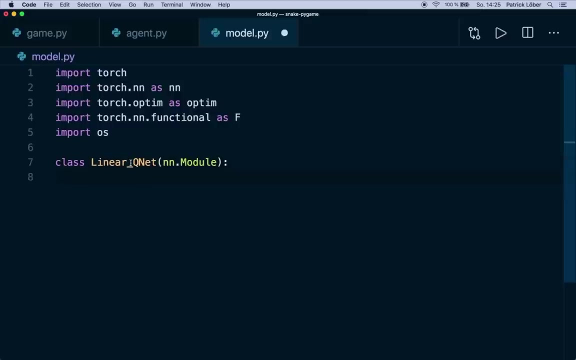 how to use this framework, then I have a beginner series here on this tutorial for free And I will put the link in the description. So this will teach you everything to need to get started with pytorch. So right now, let's start implementing this linear q net function. So we need the init. 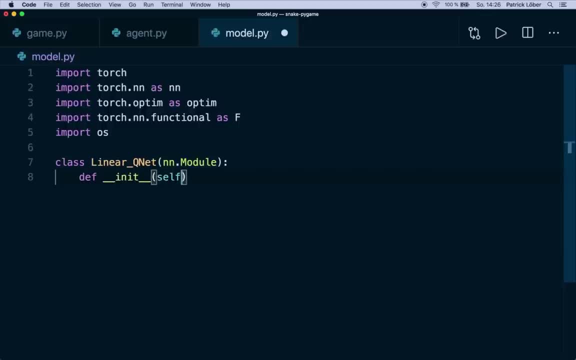 function defined init and we need to have self, And this gets an input size, input size, a hidden size and an output size. And then the first thing we want to do is to call this super initializer. So we call super in it, And here this is very simple. So if we have a look at this, 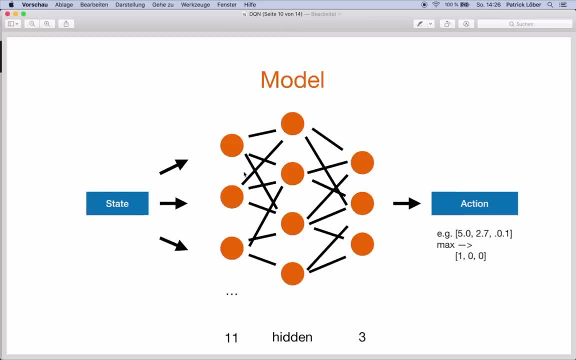 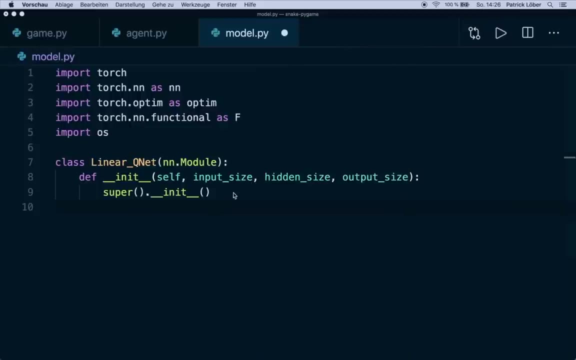 line, then our model should just be a feed forward neural net with a input layer, a hidden layer and an output layer. Feel free to extend this and improve this, but it works fine for this case And it's actually not that bad here. So let's create two linear layers. So let's call this self. 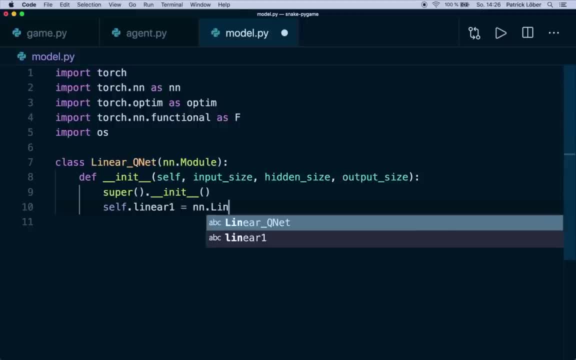 dot linear. one equals n n dot linear, And this gets the input size as an input and then the hidden size as the output size. then we have self dot linear. two equals n n dot linear, And now this gets the hidden size as the input and the output size as. 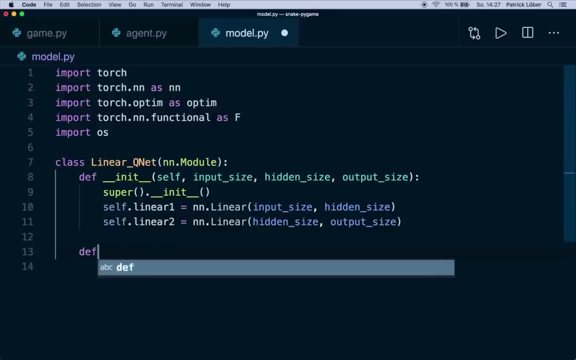 the output. then, as always in pytorch, we have to implement the forward function with self and it gets x, So the tensor. and here what we want to do is: first we want to apply the linear layer And we also use an activation function here. So again, if you don't know what this is, then check out my beginner. 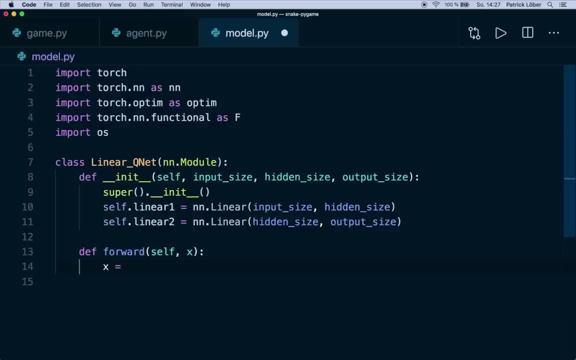 tutorial series. there I explain all of this. So we say x and then we can call f dot relu. So we use this directly from the functional module And here we say self dot, linear One, with our tensor x as the input. So first we do the linear layer, then we apply the. 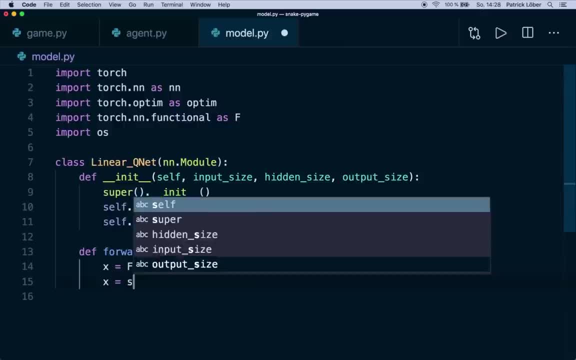 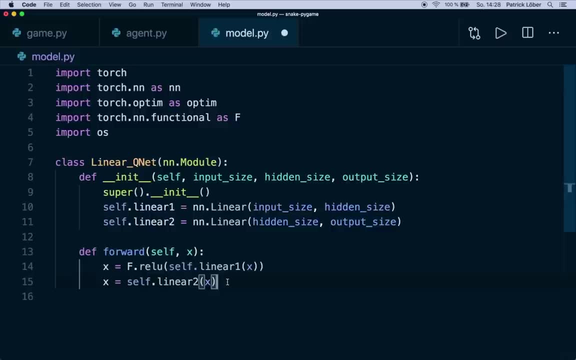 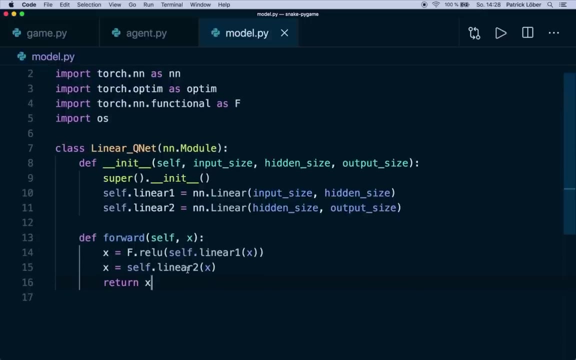 activation function. And then again we apply the second layer. So we call self dot linear two with x, And we don't need an activation function here at the end. we can simply use the raw numbers and return x. So this is our forward function. Then let's also implement a help. 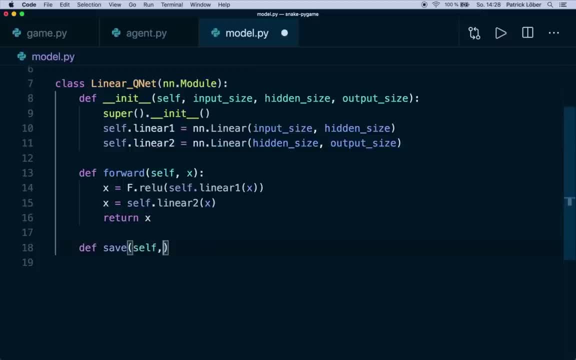 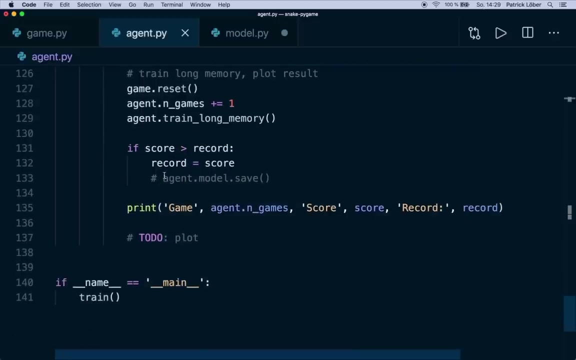 a function to save the model later. So let's call this self as safe. And this gets the file name as an input, And I use a default here. So we say model dot, p, th is simply the file name. And then the last time I think I already called this function, So not yet, But now we can comment this. 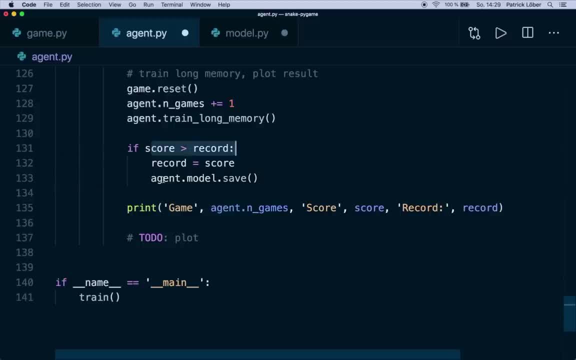 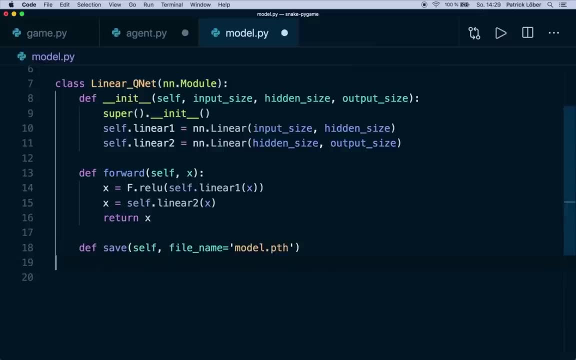 out. So if we have a new score, then we call agent dot, model dot, save, And here let's create a new folder in here. So let's say this is the model folder, path equals and let's create a new folder in the current directory and 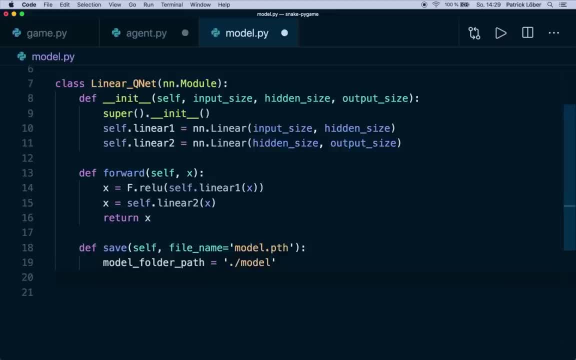 call this model, So dot slash model, And then we check if this already exists, So the file in this folder. We can say if not, o s dot path dot exists, and then we say our model folder path, then we create this. So we say o s dot make theirs and we want to make this model folder path. 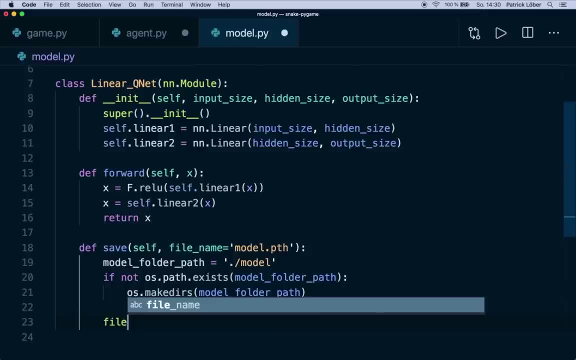 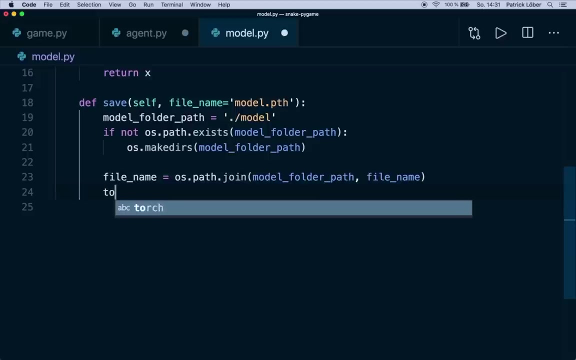 Then we create this final file name. So we say: file name equals: oh s, dot, path, dot join. And we want to join the model folder path and the file name that we use here as the input. Now this is the file name for saving, And then we want to save this And we can do this. 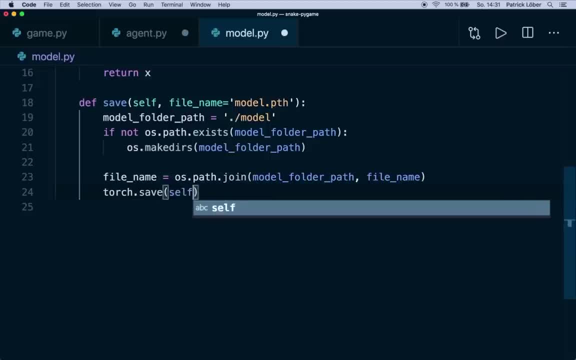 with torch dot save And we want to save self dot state dict. So I also have a tutorial about saving the model. we only need to save the model, And then we can save this, And then we can save this, And we only need to save this state dictionary And then, as a path, we use this file name. 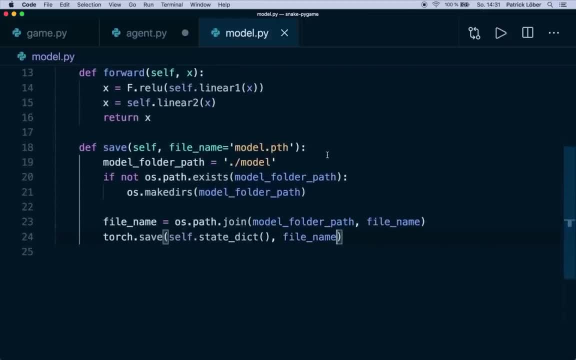 So now, this is all we need for our linear q net. And now to do the actual training and optimization. we also do this in a class that I call Q trainer, Q trainer. And now here, what we want to do: we want to implement a. 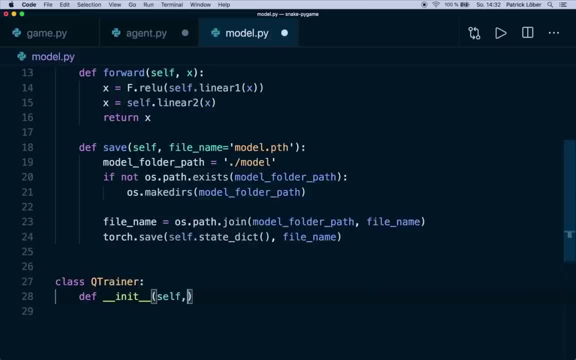 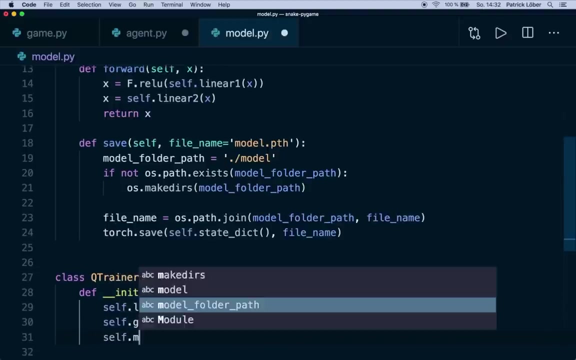 init function function which gets self, then it also gets the model, then it should get a learning rate and it should get a gamma parameter. And here we simply store everything: self dot l? r equals l r, self dot gamma equals gamma. And we also store the model. So we say self dot model. 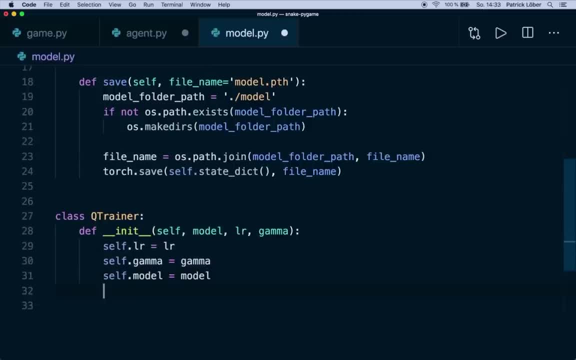 equals model. then to do a pytorch optimization step we need a optimizer. So we can create this by calling self dot optim, or let's call this optimizer equals, and we get this from the Opti module And here you can choose one optimizer. So I use the Adam optimizer And 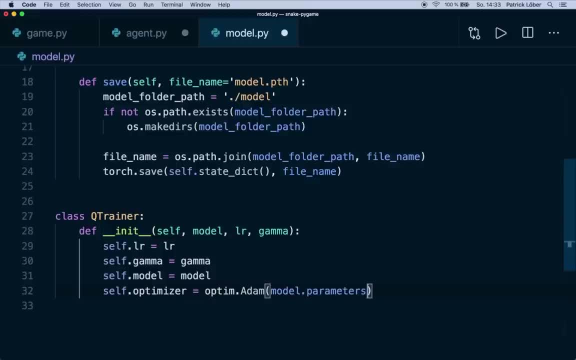 we want to optimize model dot parameters, And this is a function. And then it also needs the learning rate. So l r equals self dot l r. And now we also need a criterion or a loss function. So let's call this: self dot criterion equals. And now 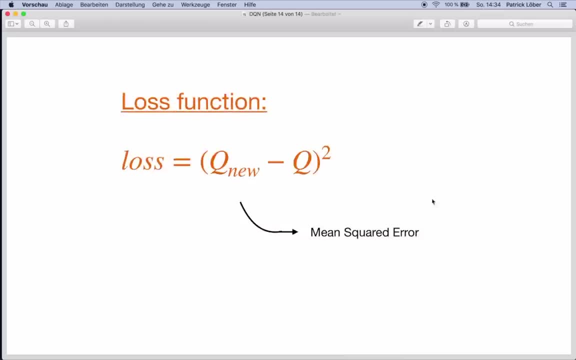 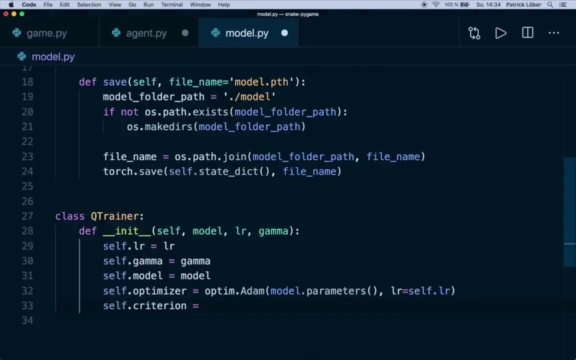 if we go back to the slides at the very end, we learned in the first part that this is nothing else than the mean squared error. So that's very simple. So we can create this here by saying self dot, criterion equals. So this is n? n dot m. 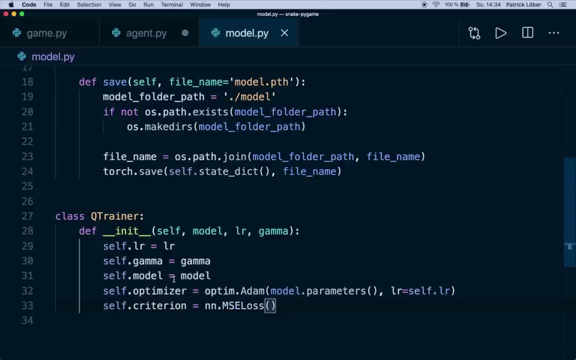 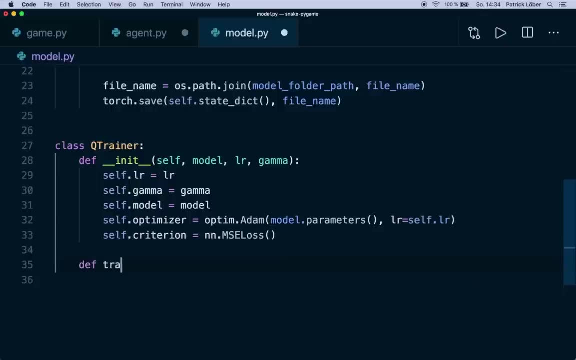 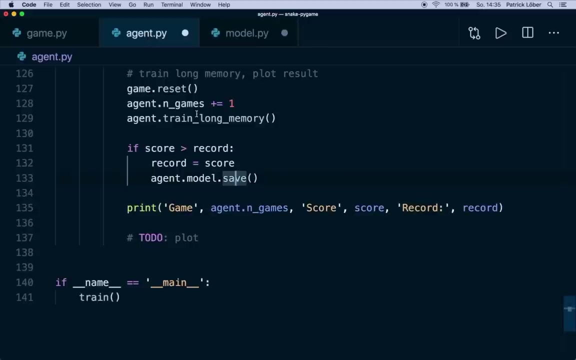 s e loss. And now this is what we need in our initializer. And then we also need to define a we call this train step function, which gets self, And then it needs to have all the stored parameters from last time, So it needs to have our. Let's have a look at this. So here, when we call this, it needs. 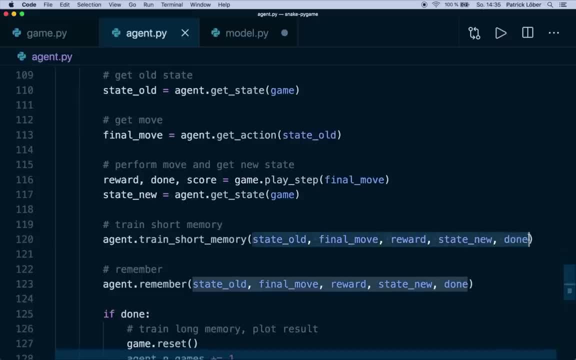 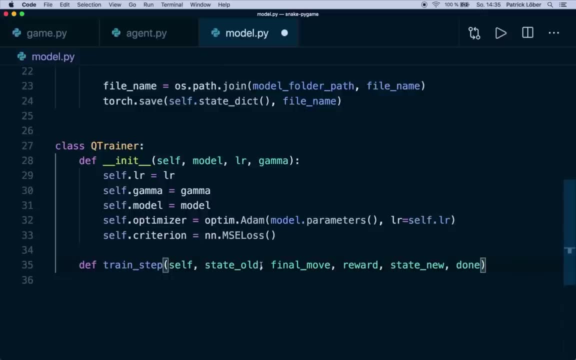 the state, the final move, the reward, the new state. and done So, let's copy and paste this in here and rename this slightly. So this is just the state, This is the action, this is the reward. So this is the new state. 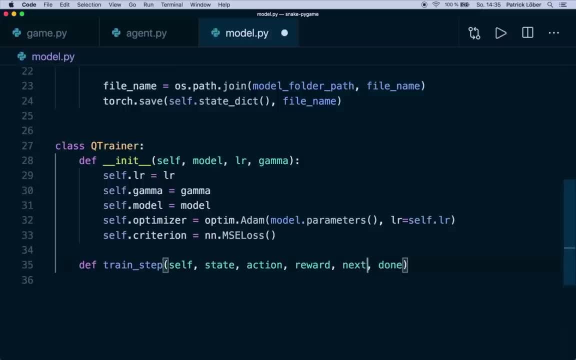 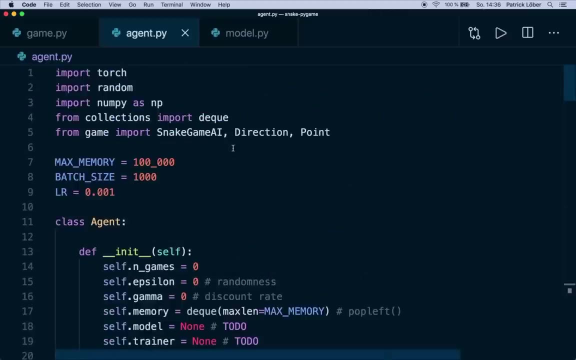 This can. let's call this next state here and then done can stay as it is, And for now, let's simply do pass here And before we implement this, let's go back to the agent and now set this up. So here we say from and we call this model and we want to import the linear. I think 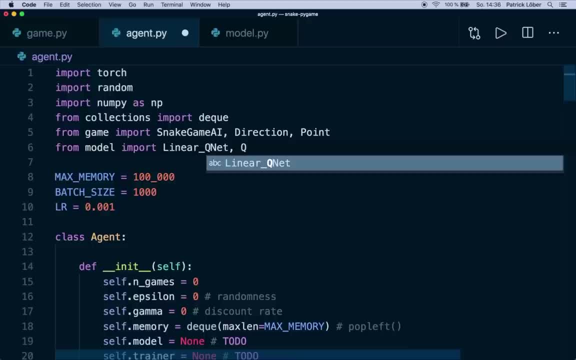 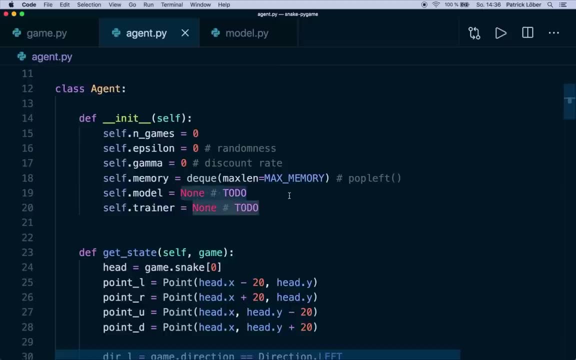 we call this linear q nets and Q trainer. And then here in the initializer we want to create an instance of the model and of the trainer. So self dot model equals our linear q net. And now this needs the input size, the hidden size and the output size. 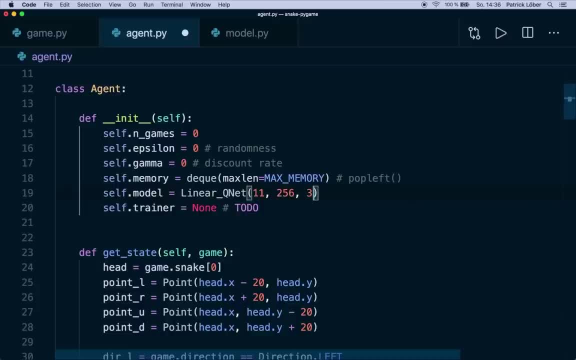 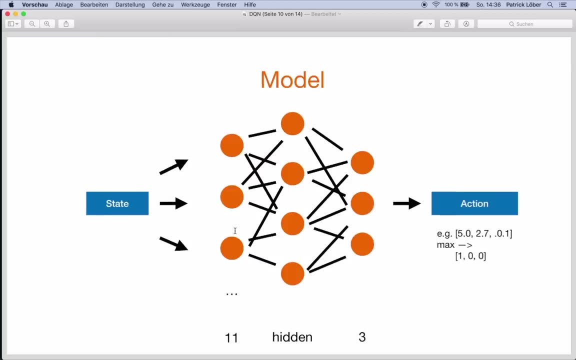 So here I use 11, 256 and three. So remember, if we have a look at the slides again, the first one is the size of the state. So this is 11 values and the output must be three because we have three different three. 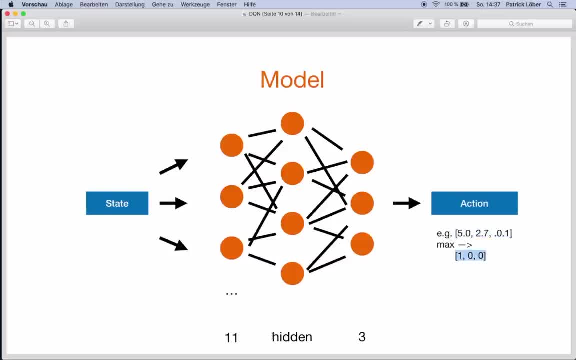 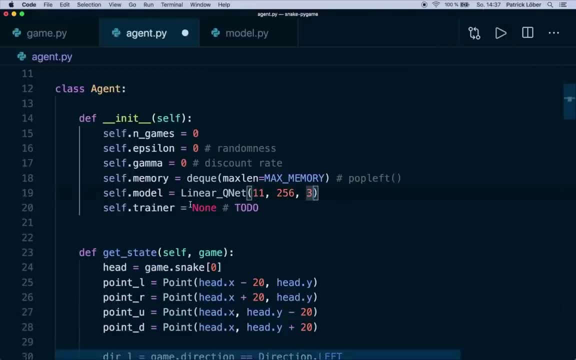 different numbers in our action And you can play around with this hidden size, but the other ones have to be 11 and three. So this is the model and the trainer And this gets the model. So self dot model. then it gets the learning rate equals the. 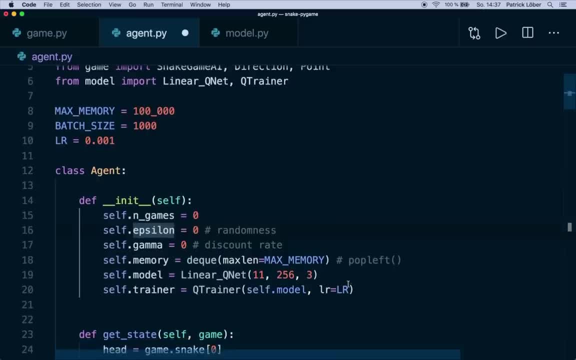 learning rate, which we specified here, And we also pass on the gamma value. So gamma equals self dot gamma And the gamma is the discount rate. So I this has to be a value that is smaller than one, And usually this is around point eight or point nine. So in this case, let's set this. 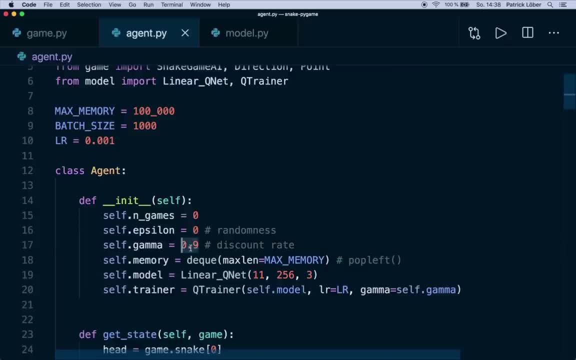 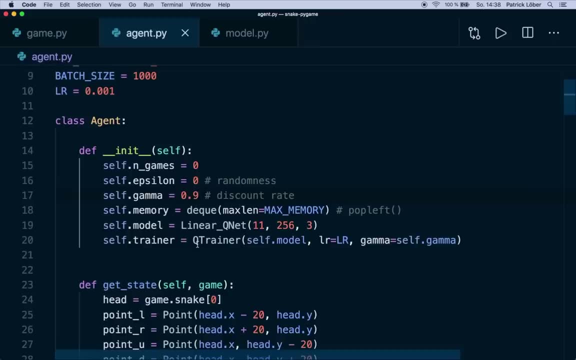 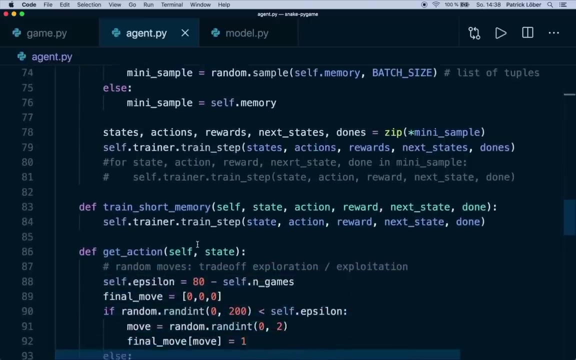 to 0.9.. So you can play around with this as well, But keep in mind that it must be smaller than one. So now we have this, and then I made one error in the last tutorial, So this is very important that we fix this right now. So here in the get action function, I actually 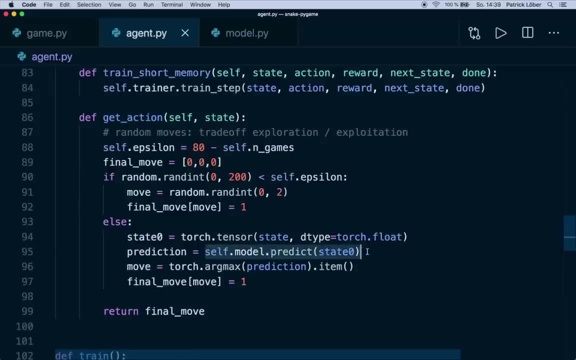 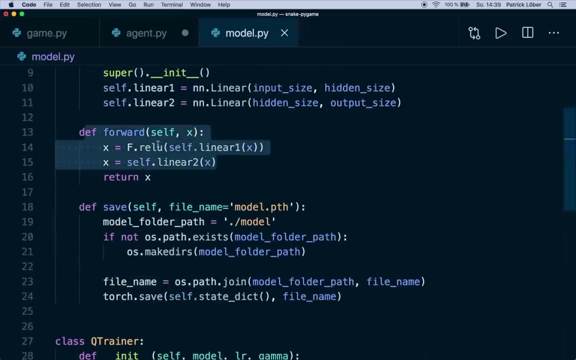 I call this self dot model predict, but actually pytorch doesn't have a predict function, So this would be the API for TensorFlow, for example. So in pytorch we simply call self dot model like this, And then this will execute this forward function. So this is actually. 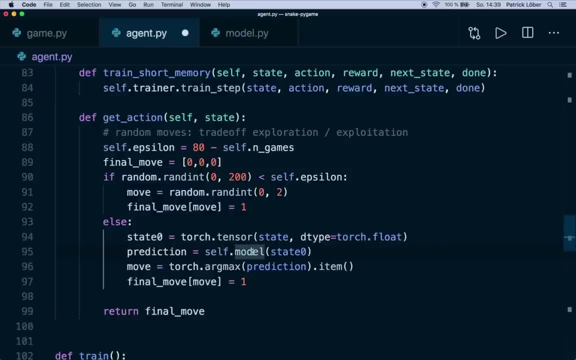 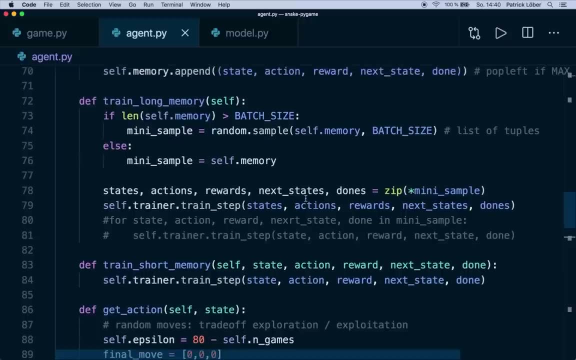 the prediction then. So yeah, please make sure to fix this. Okay, so now we have everything, And if we have a look and go back, then we see we call this self dot trainer, train step with only one parameter, but also with multiple. 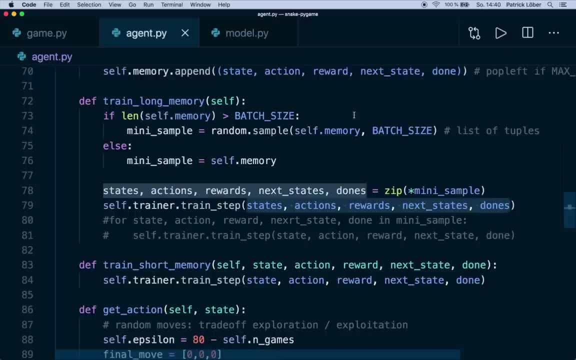 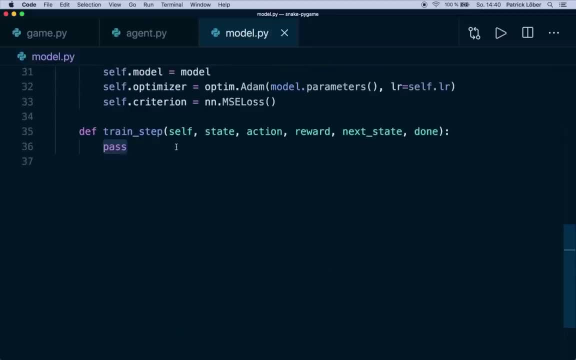 ones. So we want to make sure that we can handle different sizes. So now let's start implementing this function, And now the first thing we want to do. So right now, this is going to look like this, So this can be either a tuple or a list, or just a single value. 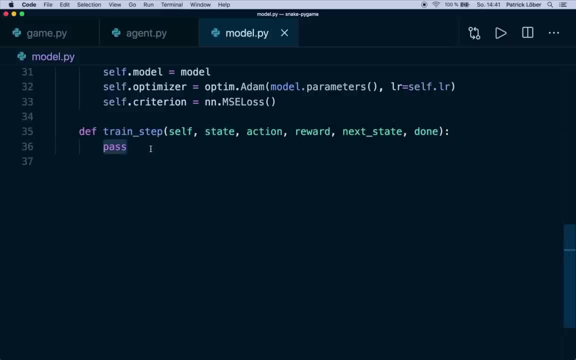 So let's convert this to a pytorch tensor. So let me copy and paste this in here. So we do this for the state, the next state, the action and reward, And we can do this by calling torch dot tensor and then the variable, and we specify the data type to torch. 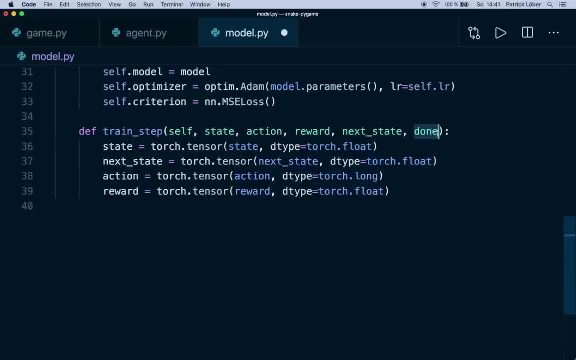 dot float And we don't have to do this for the done or game over value, because we don't need this as a tensor. And now we want to handle multiple sizes. So we want to check if the length, and then we can check state dot shape, And if this is one, then we only have one dimension. 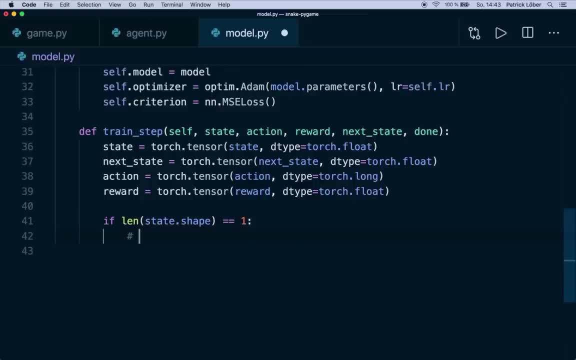 And then we want to reshape this, So right now we only have: if this is the case, then we only have one number, But actually we want to have it in the form one and then the values. So this is the number of batches. 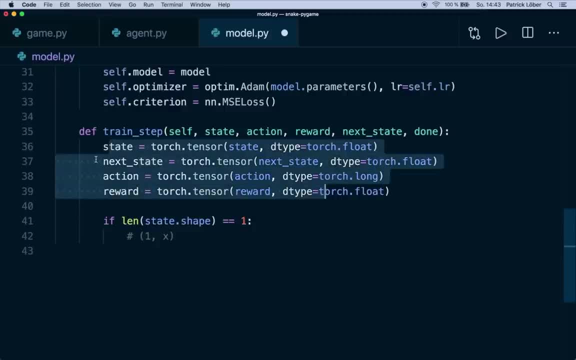 So if this is already, if this has already multiple values, then it's already in the, in the size n and x. So then it's already correct. And now here we want to, you know, append one dimension, And we can do this with the torch unsqueeze functions, So we 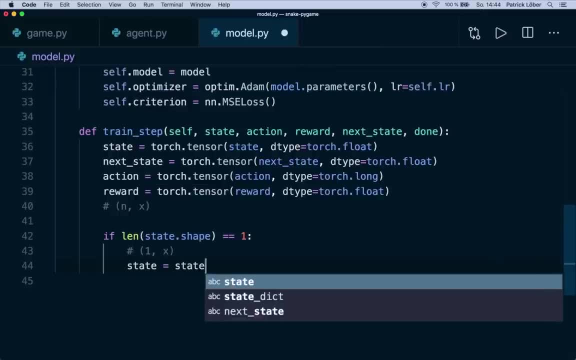 can say: state equals state dot r- sorry, not state, but torch dot on squeeze, squeeze, and then the states, and we want to put it in dimension zero or axis zero. So this means that it appends One dimension in the beginning and this is then just one. then I also wanted to do: 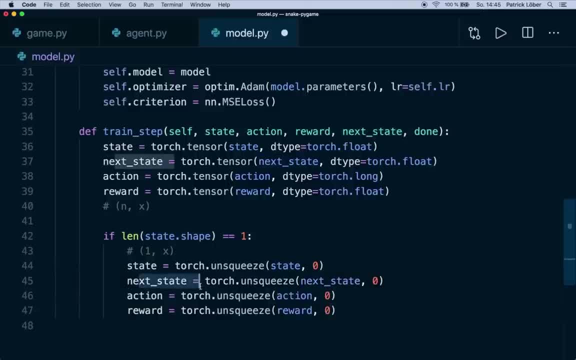 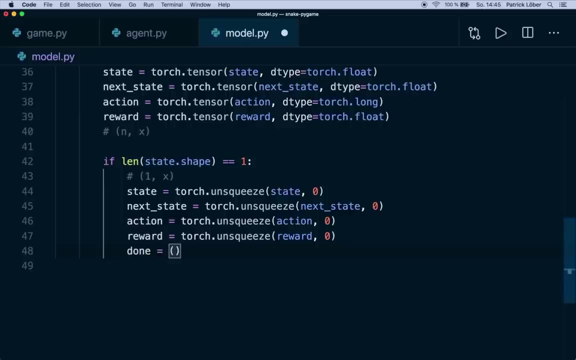 this for the other tensors, So for the next state, and for action and reward and that done value. we also want to convert this. So right now, this is only a single value And we want to convert this to a tuple, So we can do it like this. So now we have a. 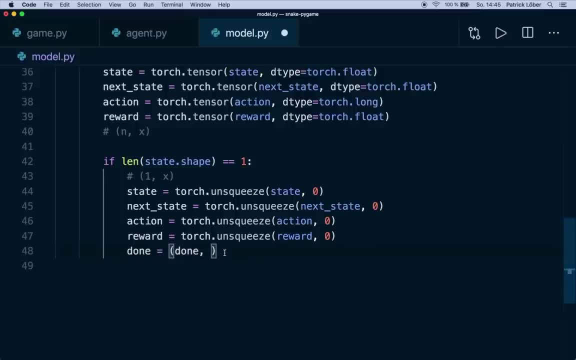 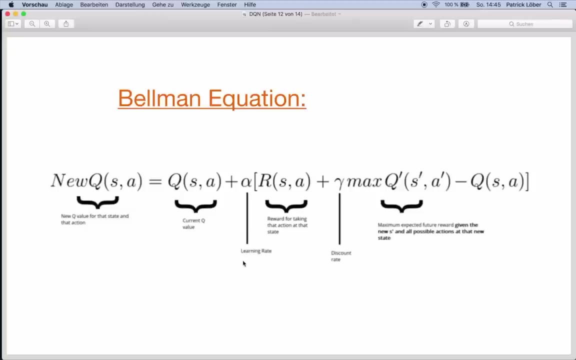 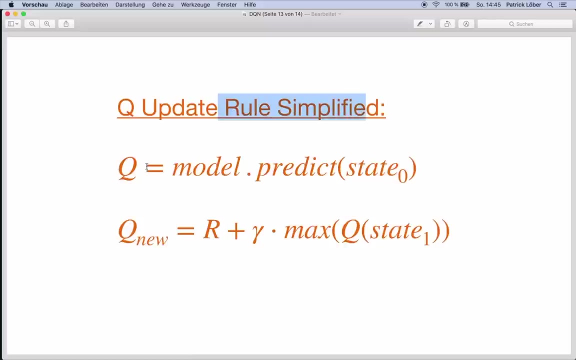 done. So. this is how you define a tuple with only one value, And now we have it in the correct shape. So now what we have to implement is from last time, or from the very first tutorial where I showed this Bellman equation, and then we simplify this, So we have the old. 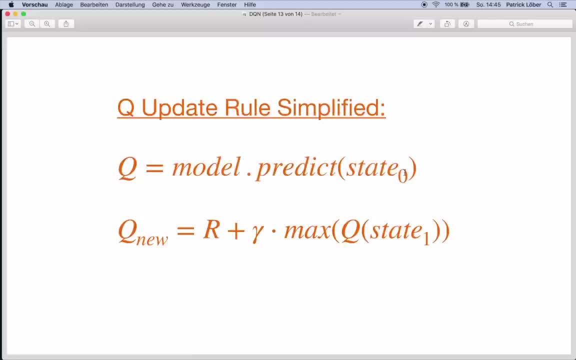 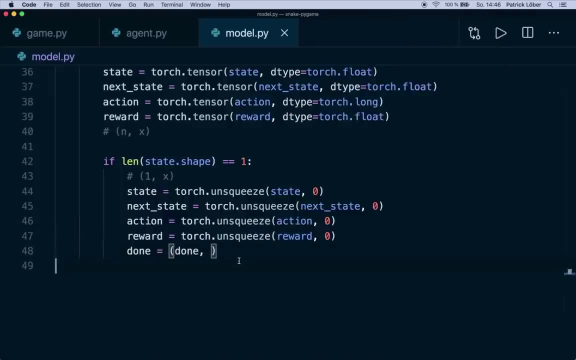 queue where we simply call model predict with the old state And the new queue with this formula. So let's do this. So first let's write a comment here. So, as first thing, we want to get the predicted, predicted Q values with the current state. 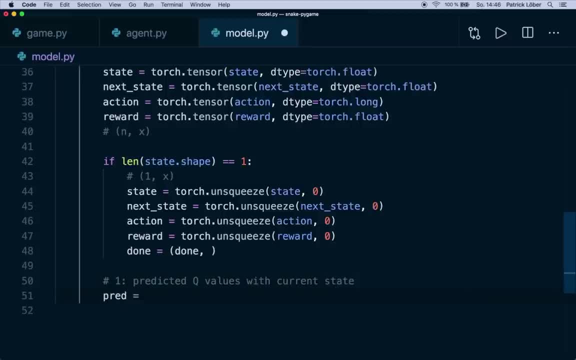 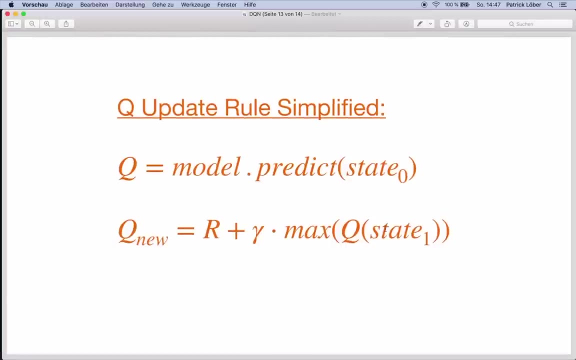 And this is simply by doing: let's call this: prediction equals self dot model, And then we want to do this with state zero, or we just call this state here, And then for the second part we need this formula: the reward plus the gamma value times the maximum of. 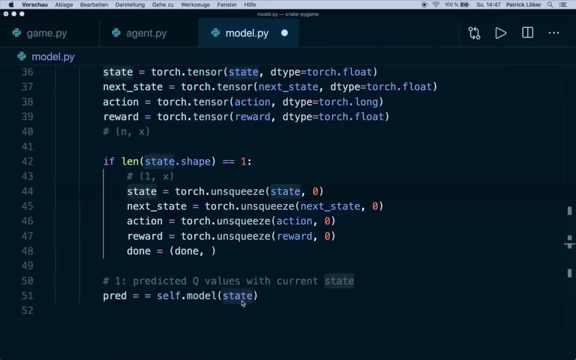 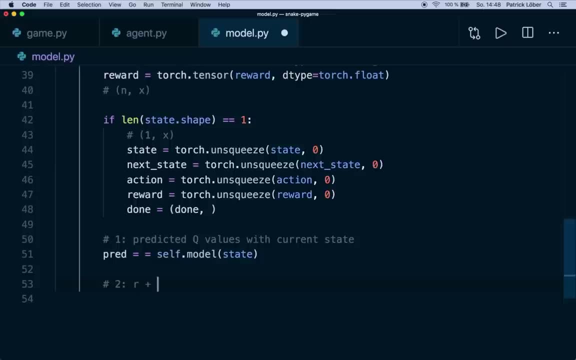 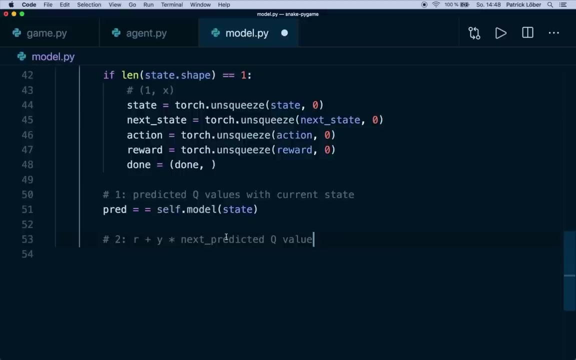 again model predict with state one. So first let's write this as a new comment. So the first thing is we want to apply this formula: reward plus gamma, Time times, and then the next predicted Q value, And then we want to have the maximum, So the 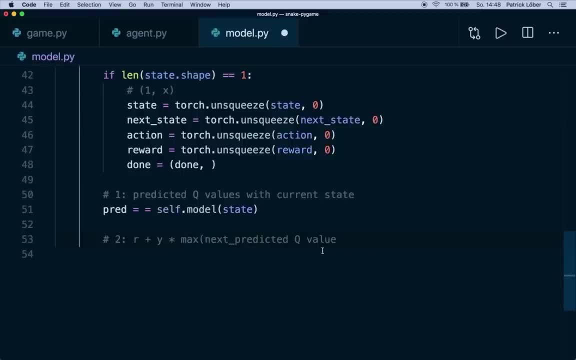 maximum of this, so maximum. And then this is a little bit tricky, So the maximum of this- sorry, let's do it like this- maximum of next predicted Q value. So this is only one value, But if we do it like as first parameter the predictions, this has actually. 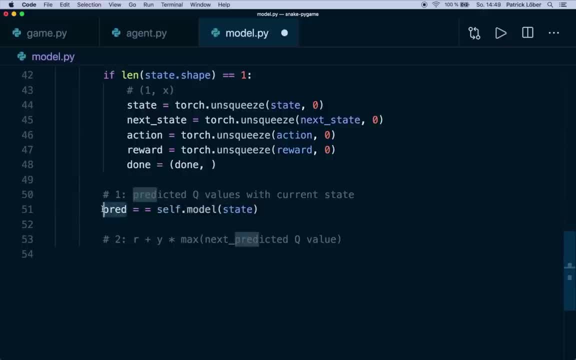 this is the action. this is actually three different values. So what we do to get the same here is we do a clone of this And then we set the index with this action to the new q value. So this is, let's call this q new, like I showed you in the formula, And then 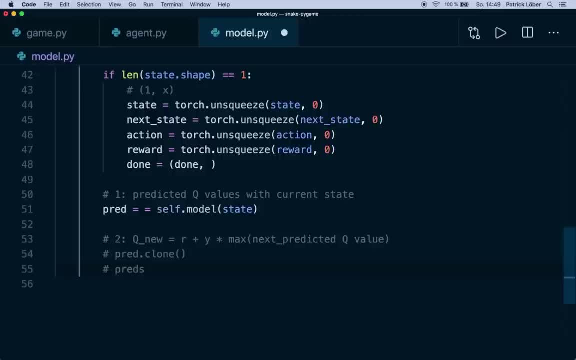 we set the- let's call this- predictions and then the index of the arc max of the action. we set this to our q new value. So again, this might be tricky. So again, we want to calculate the new q value with this formula that I showed you. But then we need to have 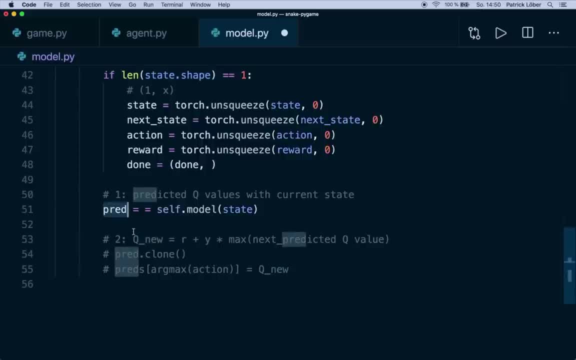 it in the same format, And for this we simply clone this. So then we have three values again, And two of the values are the same, but the value with the action. so the action is, for example, 100.. So the index of the one is then sets to the new q value. 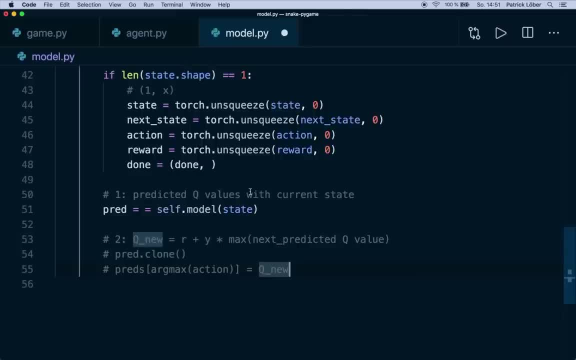 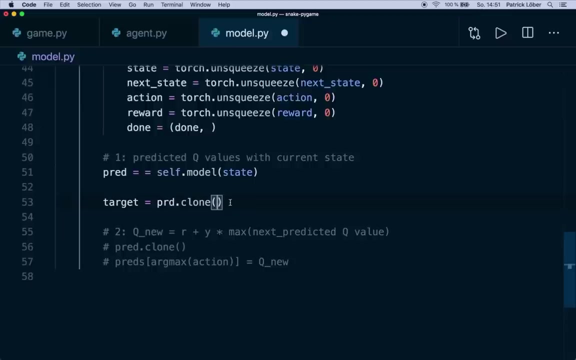 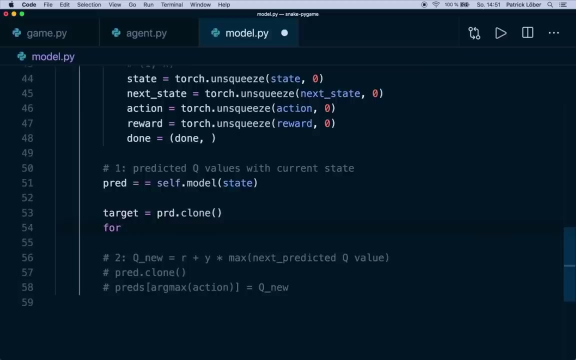 So this is what we want to do here. So for this let's first let's create a clone- targets equals prediction, dot clone- So we can do this with a pytorch tensor. And then we want to iterate over our tensors and apply this formula. So for this we say: for index in: 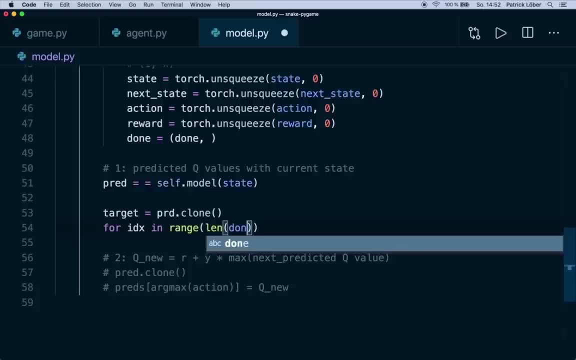 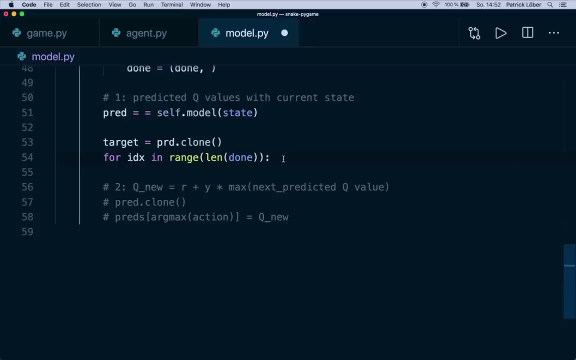 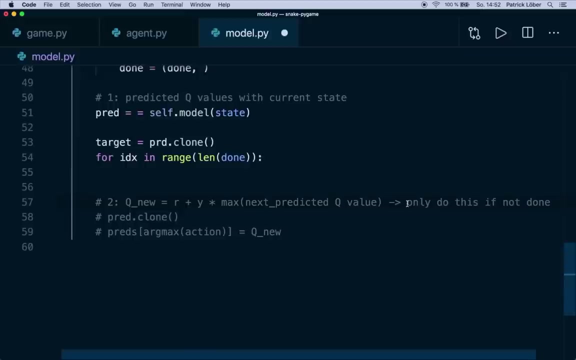 range and then the length Of the- let's call this done, And here everything should have the same size. So then this works. So now we iterate over this, And then one thing that I didn't mention so far is that we only only want to do this, only do this. if not done Otherwise, we simply take the 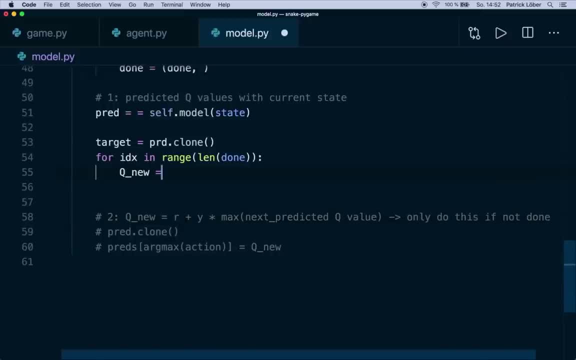 whole reward. So we say q new equals re ward of this Of the current, current index. And now we check if we are not done. So we say if not done and the done is of the current index, then we apply this formula. So now we say q new. 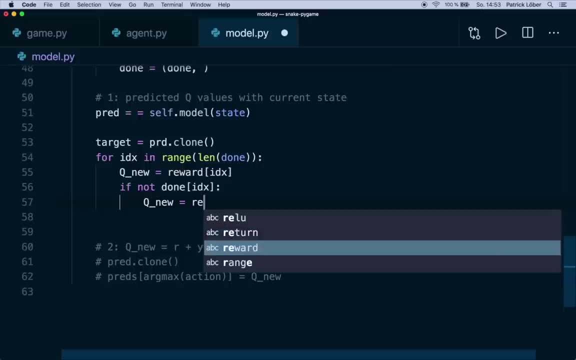 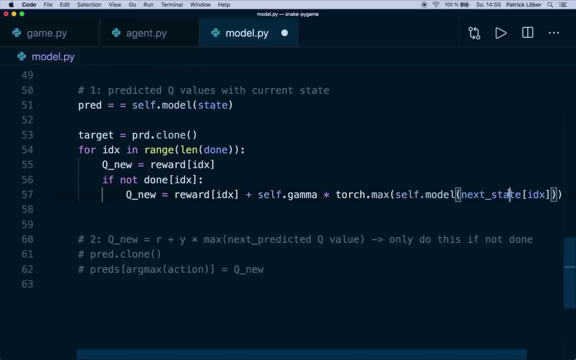 is actually the reward. So the reward of the current index plus self dot q, gamma, and then times torch dot max, the maximum value of the next prediction. So here, self dot model of next state of this index. So this is exactly what we have written here. 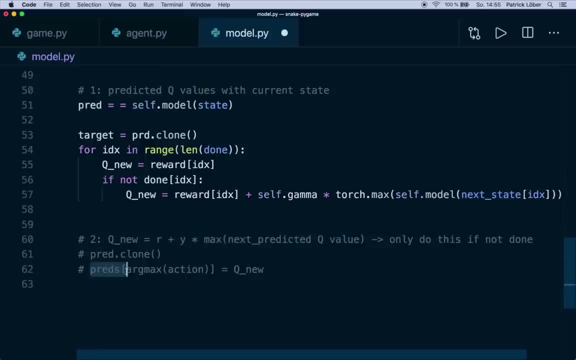 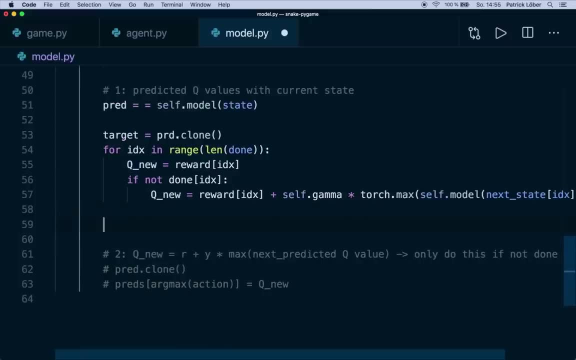 And now we need to set the target of the maximum value of the action to this value. So here we get the. let's we call this target So the target of the current index and then of the arc max of the action. So for this we can again say torch. 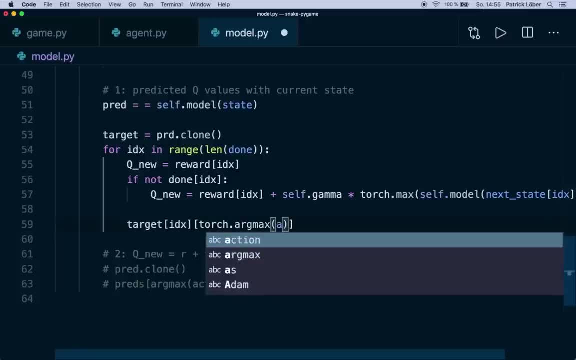 dot arc max of the of the action, and we want to have this as a item, so as a value, and not as a tensor. And now this is our q new value. So this might be a little bit tricky to understand. So I recommend that the that you pause here and go over this again. And now we have everything. 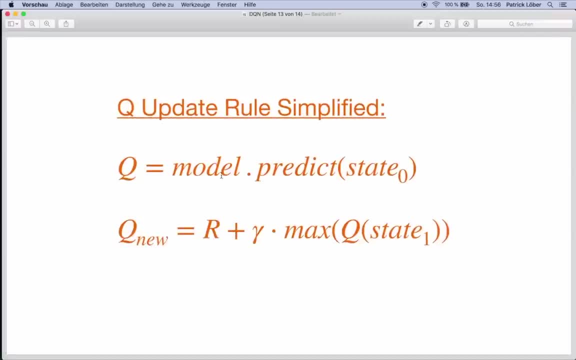 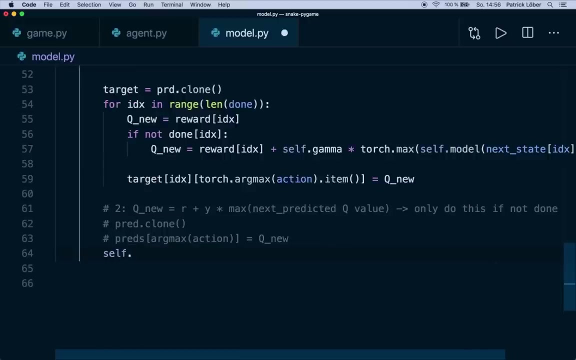 that we need. So let's have a look at the slides Again. we have our q and our q new, And then we apply the loss function, So the mean squared error and in pytorch. So what we have to do here, we can simply use this optimizer and do a step, And first we have to call this: 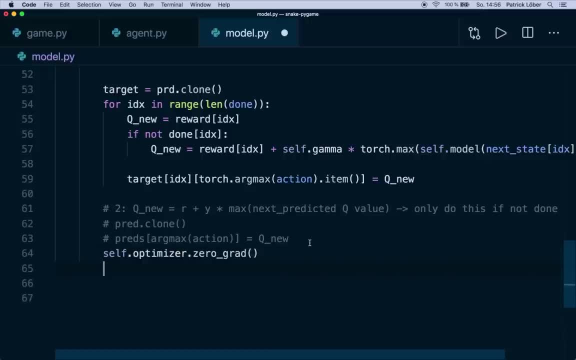 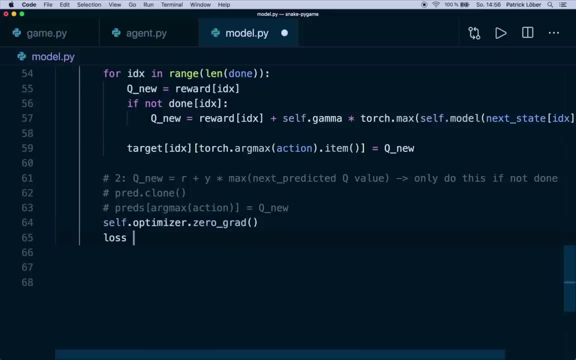 zero grad function to empty the gradient. So this is just something that we have to remember in pytorch. And then we calculate the loss by calling self dot criteria, And here we put in the target and the prediction. So this is q new. 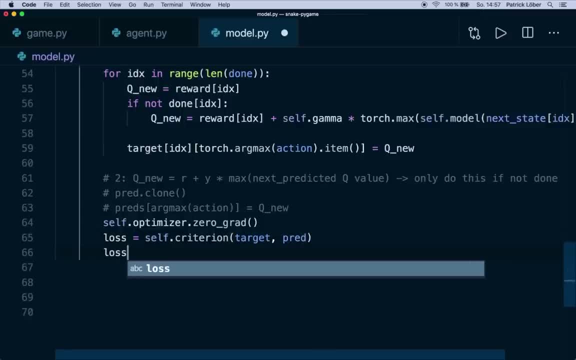 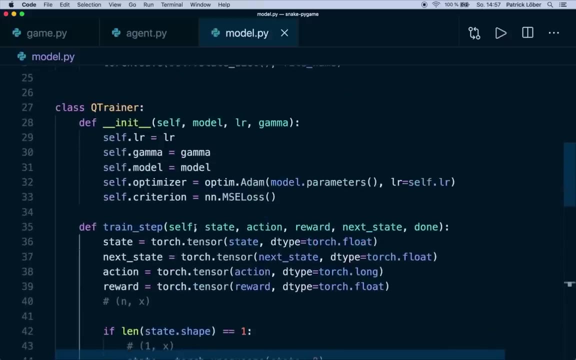 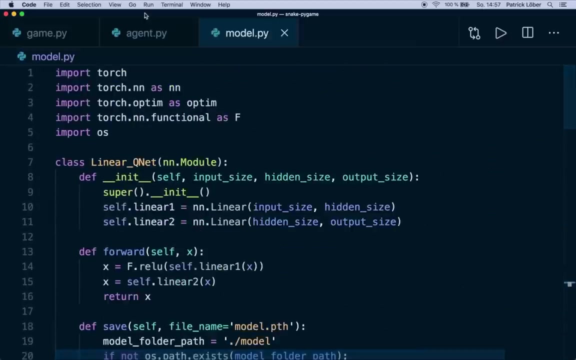 q new, q new And q. And then we call loss dot backward and apply back propagation and then update our gradients. And then we call self dot, optimizer, dot step. And this is all that we need in this training step. And now, this is actually all that we need in this model file. So now, 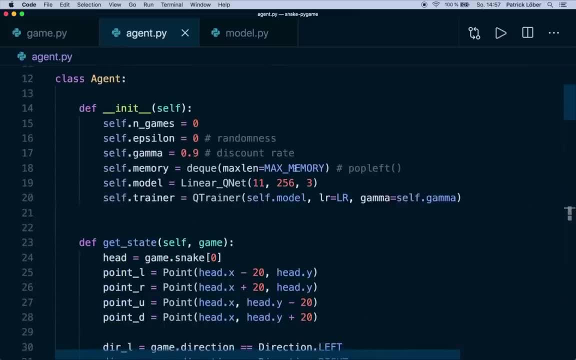 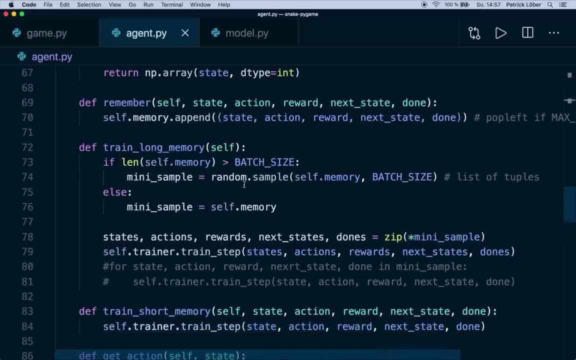 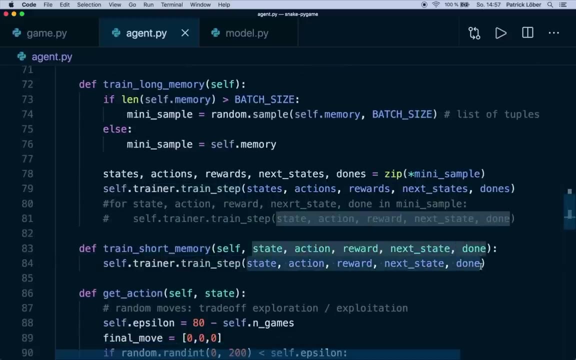 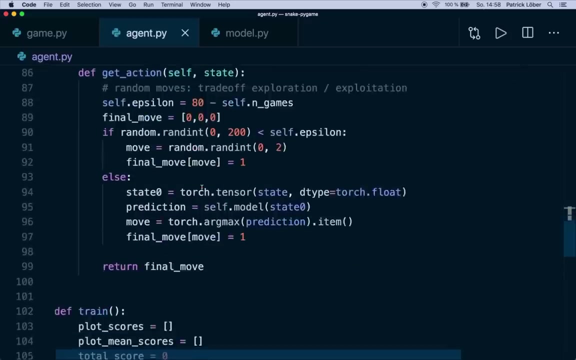 again. let's go back to the agent, And I guess we already set up the Q trainer, And then, when we train this, we call this train step function, either for only one of those parameters or for a whole batch. And now this function can handle different sizes. And now the only thing left to do here is: 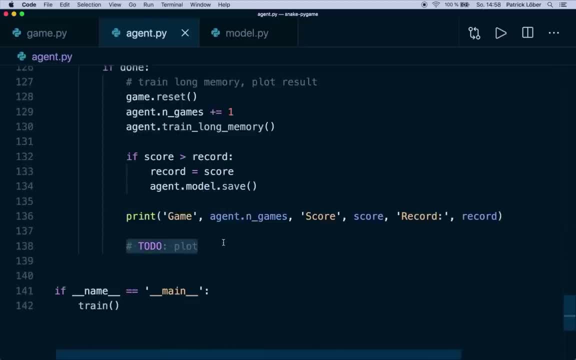 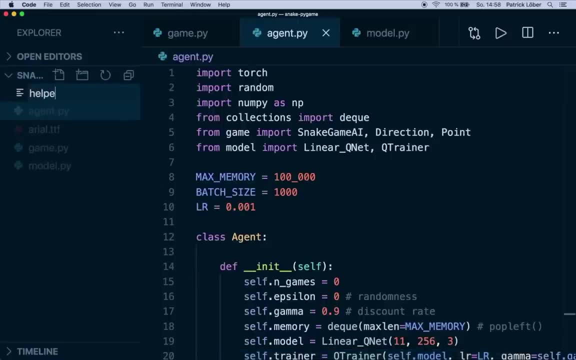 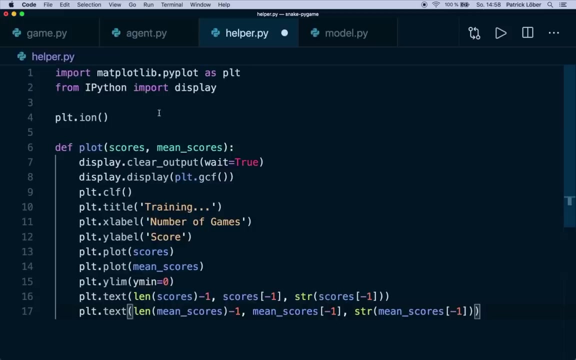 to actually have to plot the results. So for this let's say: let's say: let's say, let's create a new file And let's call this hell helper dot pi. And then here let me actually copy and paste this in here. So this is just a simple function with matplotlib and IPython. 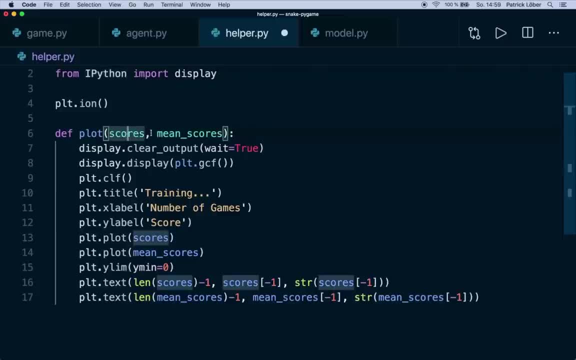 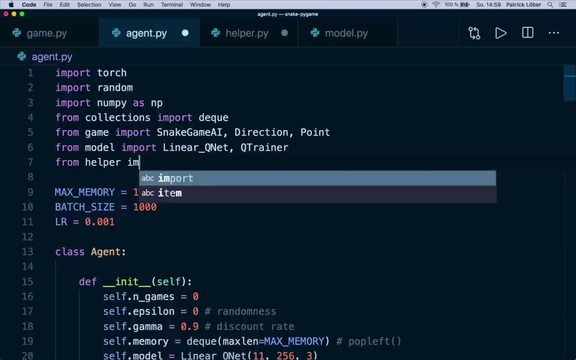 And yeah, here we want to plot the scores. So this is a list and we want to plot in the plot the mean score. So let's create a new one. And here let's say, let's say let's create them. So here in the agent we say from helper import the plot function and 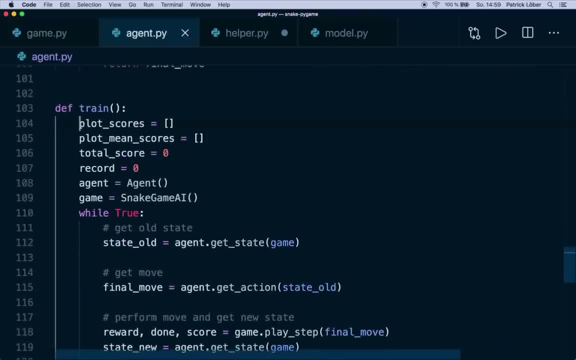 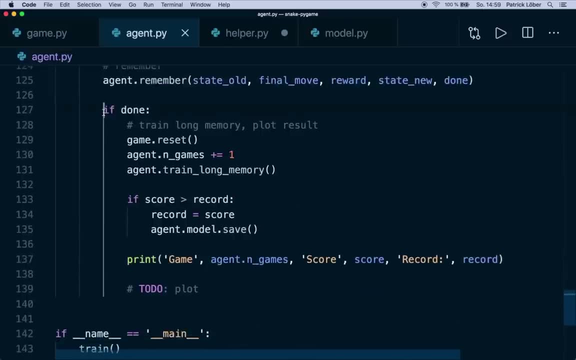 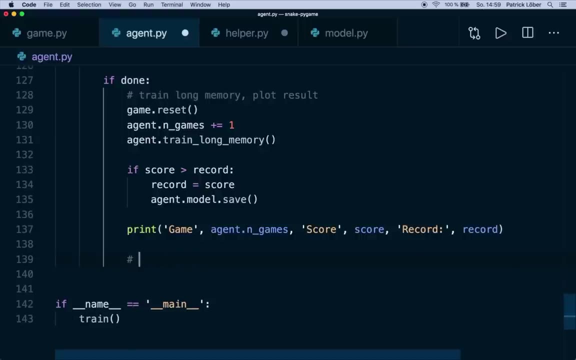 then down here and the training function. So we already created an empty list for the scores and for the mean scores And now after each game we want to append the score. So let's remove the to do and implement the score And this so we say plot scores: dot appends and then the current score. then let's calculate. 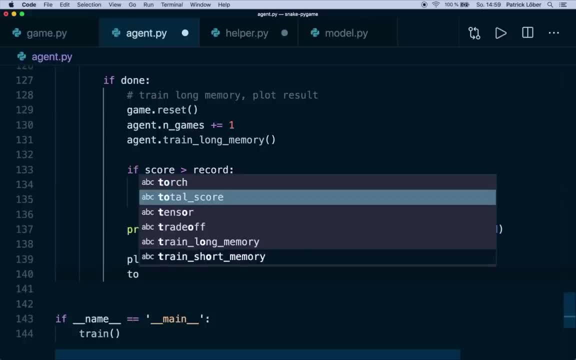 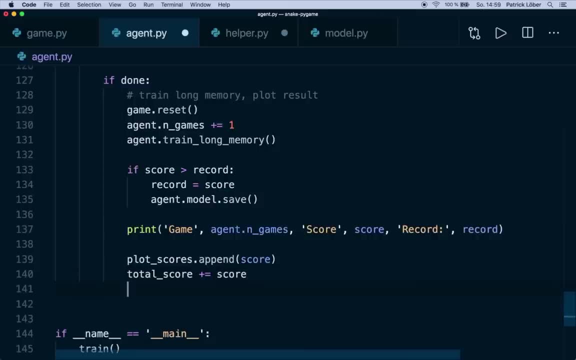 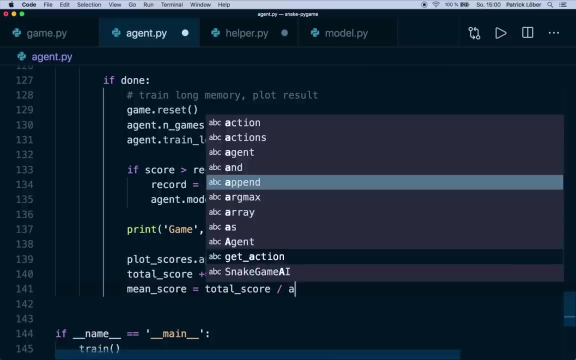 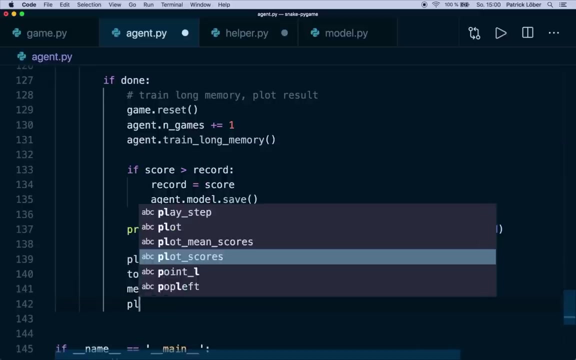 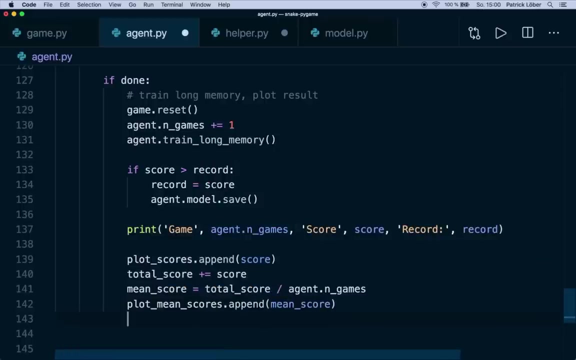 the new mean or average score. So for this let's say: total score plus equals the score, And then let's call this: mean score equals the total score divided by the number of games, So H. And then we append this to plot mean scores, dot append the mean score, And then we simply 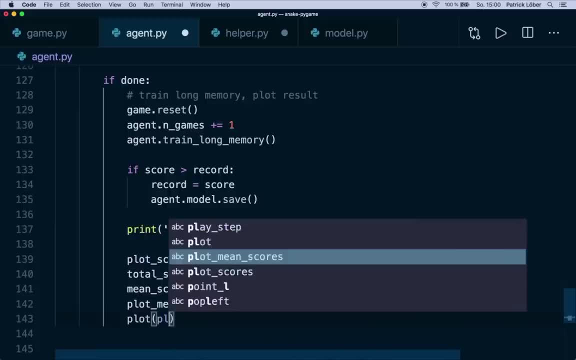 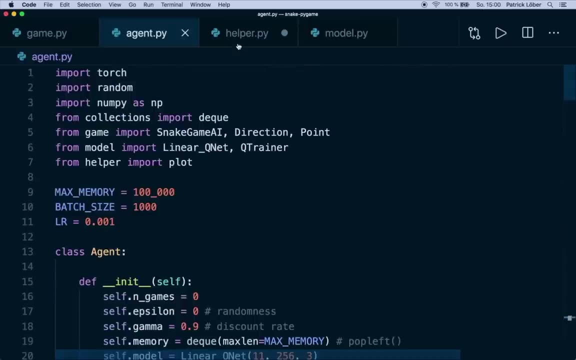 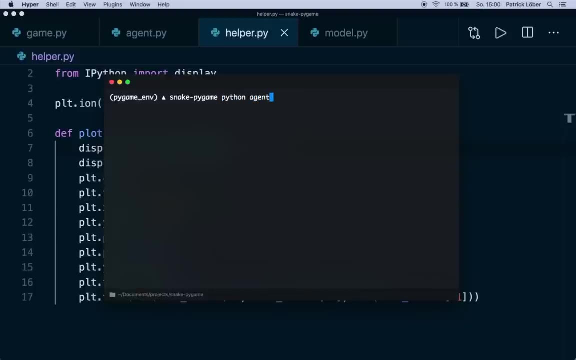 call the plot function with the plot scores and then the plot mean scores And now let's save this file And also let's save this file And then let's try it out. So in the terminal let's call H And dot pi and let's cross fingers. So we have a syntax error in the model dot pi file. 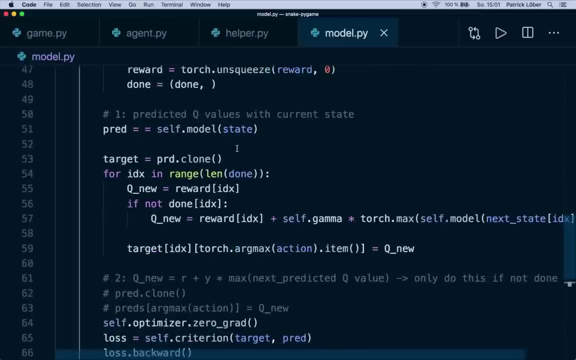 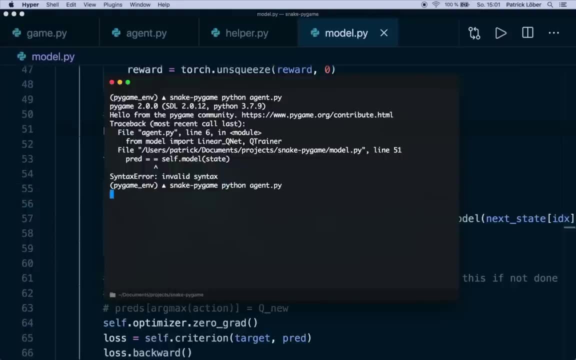 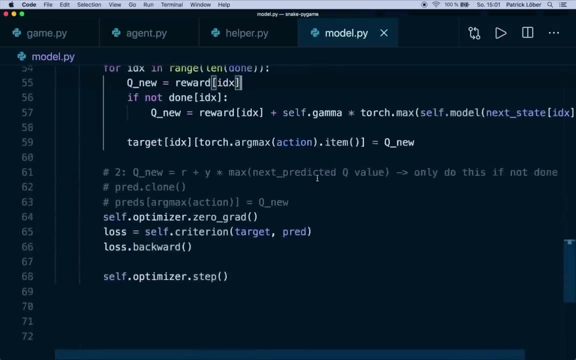 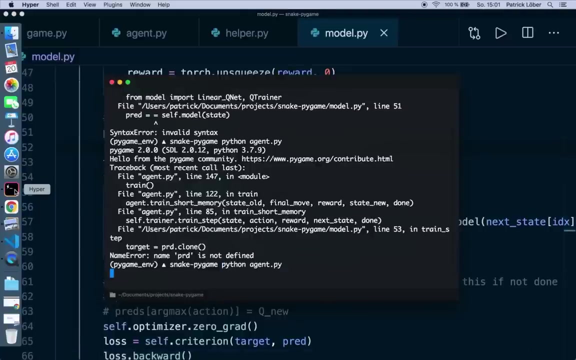 So here we actually, here we have to equal signs. So let's fix this and save this and run it again. And then we made another mistake: name error. So here this is actually called prediction dot clone. So again, let's save this and run this. And now it starts.